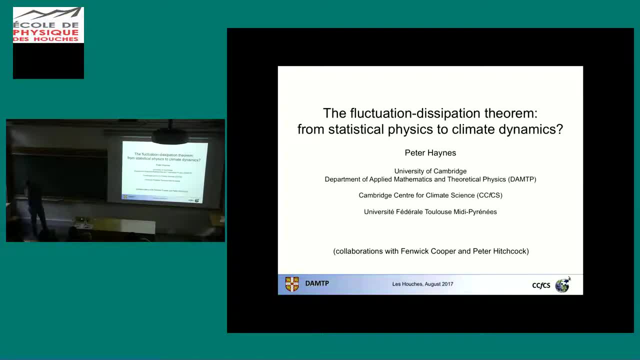 I'm going to try to give a seminar on the fluctuation dissipation theorem. So this is kind of a topic which I've been interested in over the last few years. Not really clear what progress I've made in this topic, but it's kind of an interesting one which draws 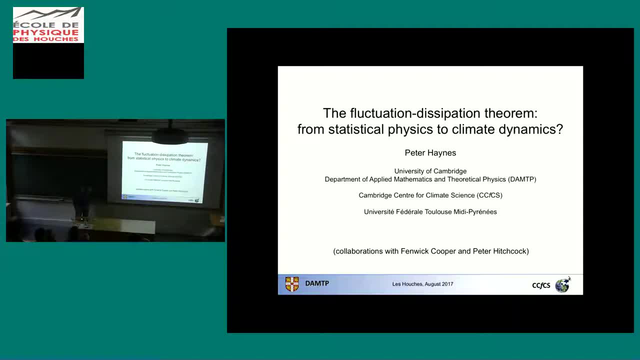 together different ideas and has some interesting possible applications. And I should say that this is. I've collaborated with Fennec Cooper on this topic and I've also had lots of interesting conversations with Peter Hitchcock, And the other thing I should say here is that 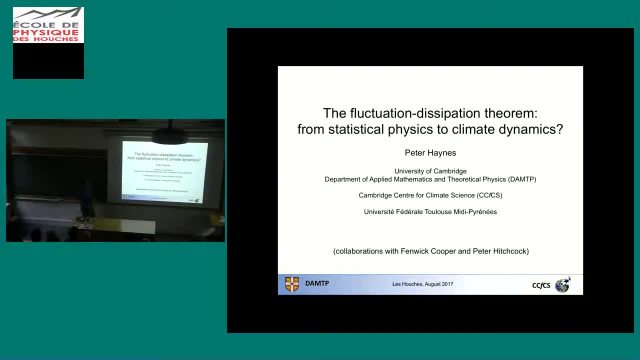 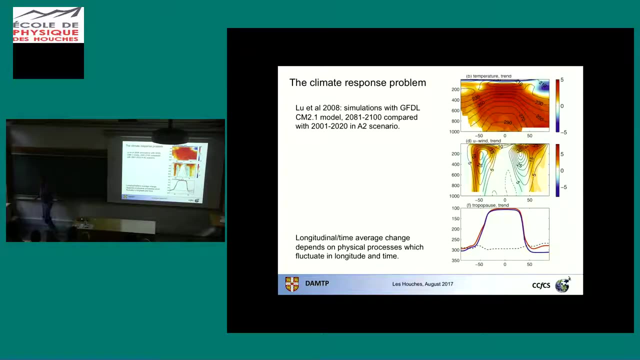 I've just spent quite a lot of the last couple of years in Toulouse and I sort of acknowledge their support for my research over the last couple of years, Right, So this is kind of motivation. So I imagine that in Ted Shepard's lectures he 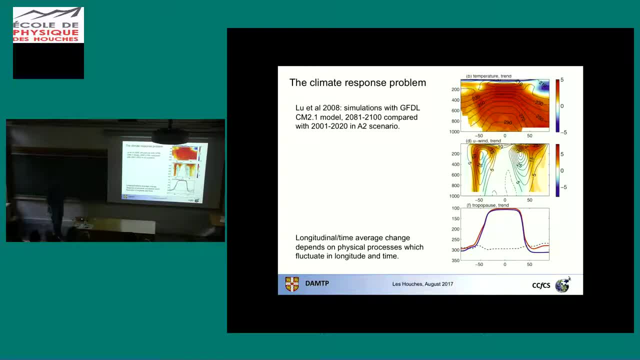 talked about these sorts of problems, So you could define something called the climate response problem. You say I'm going to, I'm going to increase greenhouse gases by some amount and how do different measures of the climate system change? And, if you like, the kind of traditional historical focus has. 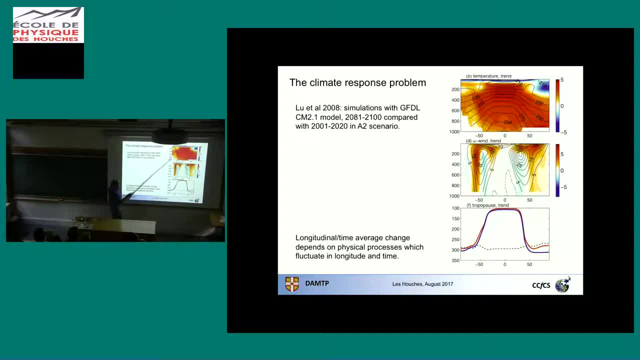 been on temperature so that if you increase greenhouse gases then you get systematic increases in temperature, You get warming of the troposphere, you get cooling of the stratosphere, And I guess one thing that's become of more interest recently is not just 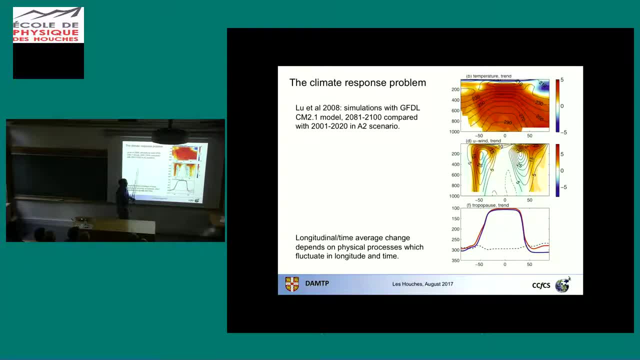 things like, Yeah, global average temperature, but also changes in circulation, And I'm toldI'm sure that Ted Shepard talked about issues- changes in circulation and regional climate et cetera. So in this kind of typical greenhouse gas increased experiment, not only was there an, 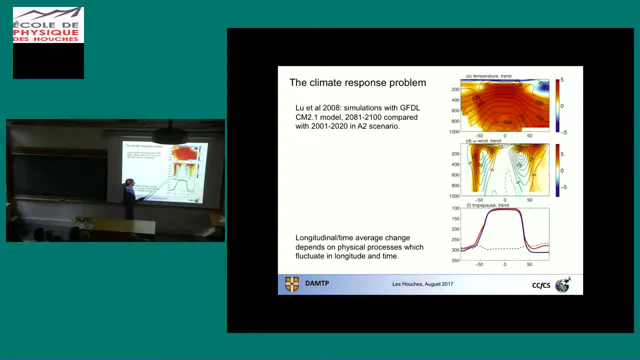 increase in temperature in the troposphere but there was a change in the winds, The colors of the change in the winds, the contours of the kind of climatological winds. This is a tropospheric view of the world. Pressure, Pressure coordinates, The stratosphere is kind of the top 10% of this picture, But the 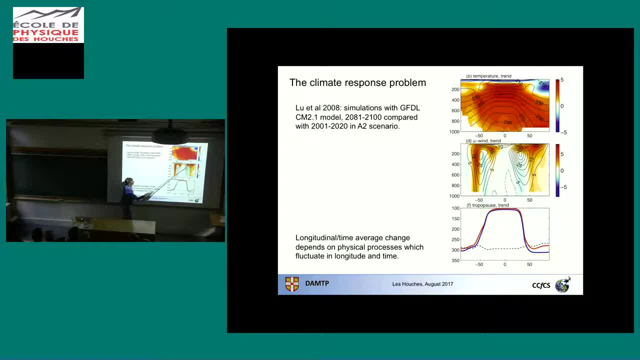 basic story here is that you have subtropical westly jets and, under increased greenhouse gases, those are moving poleward. okay, So there's a negative change in the wind at low latitudes on the equator side of the jet and there's a positive change on the poleward. 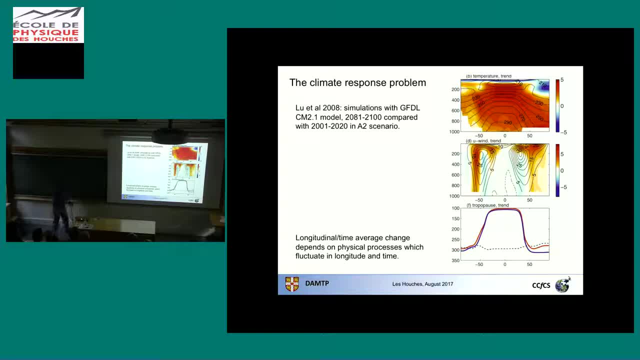 side of the jet. Now, of course, this is a longitudinal average picture And I think you know there's a lot of It's a longitudinal average picture And what we know is that you can't understand these sorts of changes simpler by looking at a longitudinal average dynamics, which 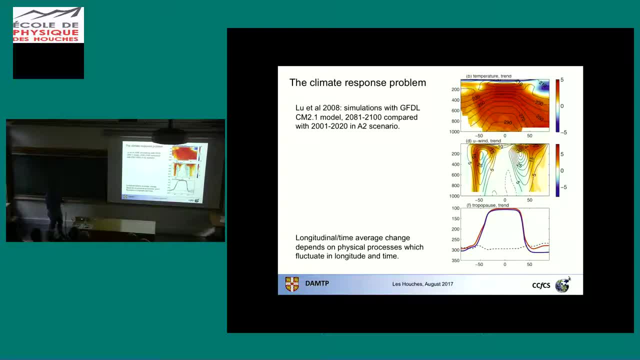 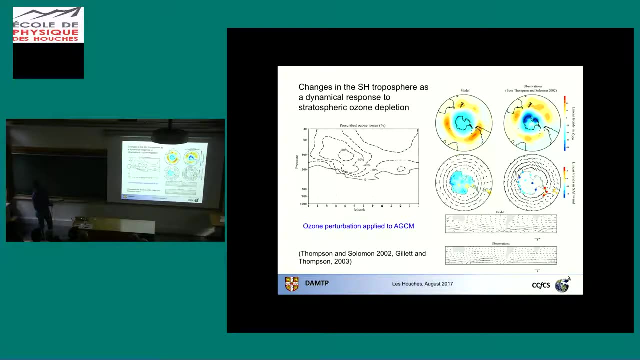 only considers longitudinal average quantities. You need to consider It is, You need to consider the fluctuations in longitude and time to understand these sorts of changes. I mean another example of this kind of problem: how does the circulation change if you change something in the atmosphere? is the response to stratospheric ozone depletion? So about, 15 years ago people started to realize that there were changes in the circulation in the southern hemisphere And you know work by Thomson and Solomon and Givison Thomson and many others have kind of established how ozone depletion in the lower stratosphere in late. 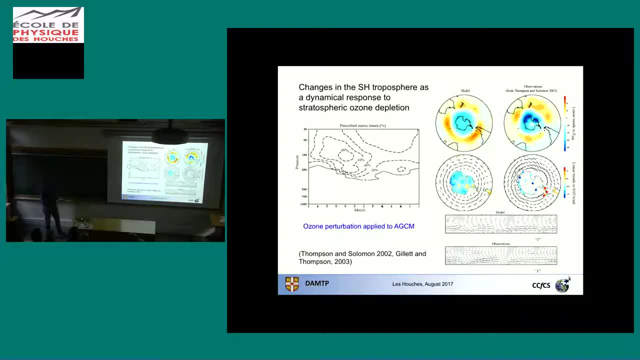 In autumn in the- Sorry, I mean in spring- in the southern hemisphere. So you know, there's a lot of, There's a lot of In the southern hemisphere- leads to a change in the tropospheric flow, And these are examples. 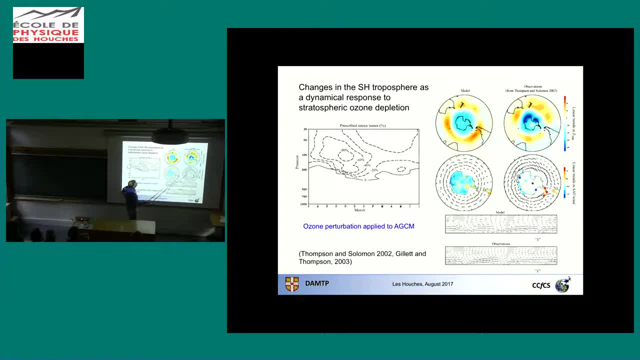 from model simulations and from observations. where one's looking at These are differences in geopotential heights. In this case observations, it's changes over a couple of decades between 1980 and 2000-ish. In this case, it's changes which are being driven in a model by an artificial. 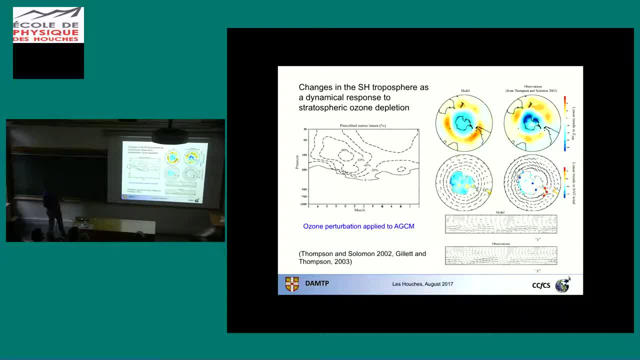 depletion of ozone And therefore removal of radiative heating in the lower stratosphere. And you know, these dynamical changes are associated with changes in the surface winds. So one gets an intensification and a poleward shift of the westerlies okay, which can have implications. 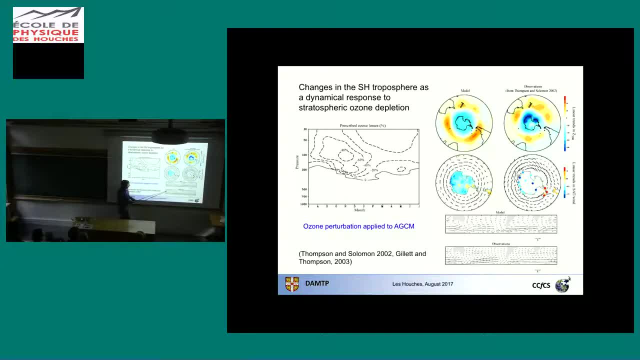 for rainfall, for example. So if you live in southern Australia and you rely on the prevailing westerlies to provide rainfall, so to speak, then the poleward shift of the jet is going to change regional climate. So this is another example of. we have a system, the tropospheric circulation. we apply a perturbation. 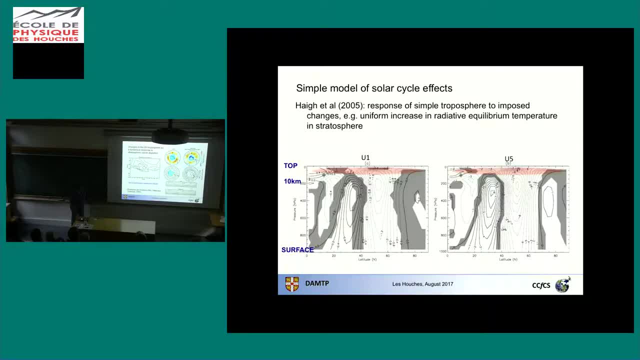 we reduce ozone, we get a response. Another angle on this is solar cycle effects. okay, So there's been a lot of interest over many decades in the possibility that the 11-year solar cycle may change. So you know, if we have a system that's at the top of the atmosphere, we have a system that's at the 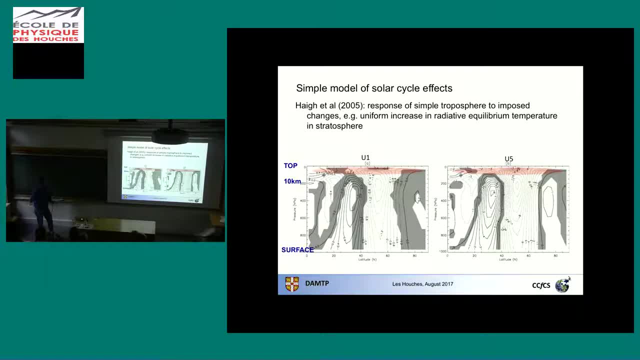 bottom of the atmosphere. we have a system that's at the bottom of the atmosphere and we apply a perturbation, So we reduce the response and we reduce the response. Another angle on this, the direct effects of which are only plausibly felt in the upper atmosphere. 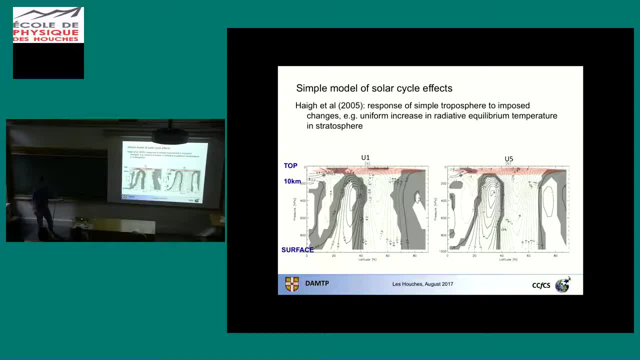 perhaps at around 40 or 50 kilometers or above, might be somehow transmitted to the lower stratosphere and to the troposphere. This is some results from a sort of idealized set of experiments by Hegetal again about 10 years ago, where they took a model tropospheric circulation. 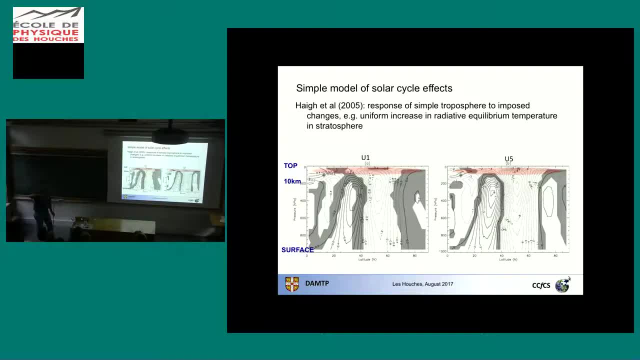 and they simply applied a kind of warming, artificial warming- in the stratosphere And they asked how the circulation changed. And these are the changes. This is now going from equator to north pole, equator to north pole. In these two experiments you basically had a sort of uniform warming applied in the stratosphere. 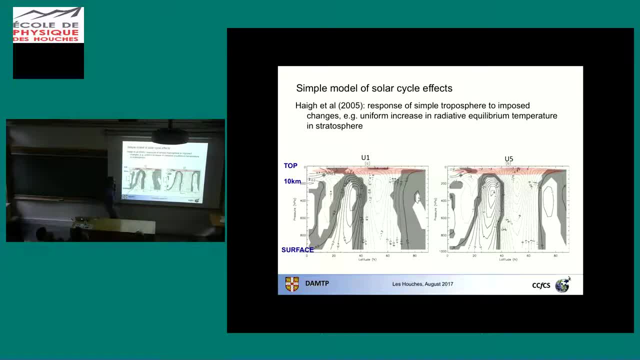 But in this case it was five times larger than here And again. well, the change here is manifested as a shift of the tropospheric jet. So then, in this case, in fact, you have positive wind anomalies to the south of the position of the climatological jet. 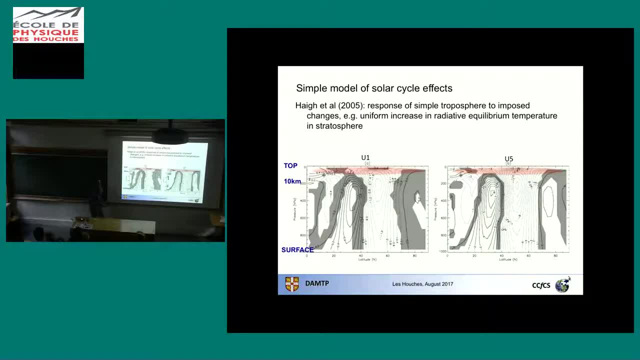 and negative wind anomalies to the north. And what's kind of interesting is that the patterns in these two pictures look the same, broadly speaking, And indeed they even kind of almost scale with the amplitude of the perturbation. So it kind of suggests that some kind of linear theory might explain these sorts of changes. 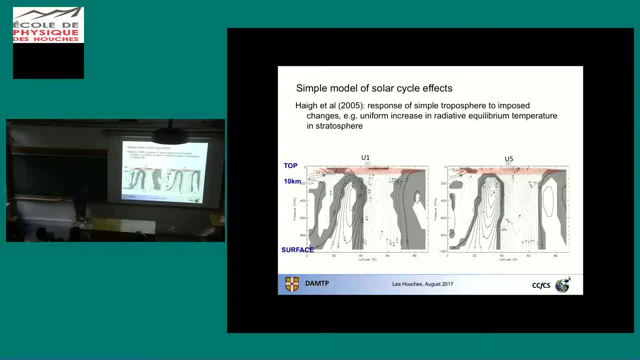 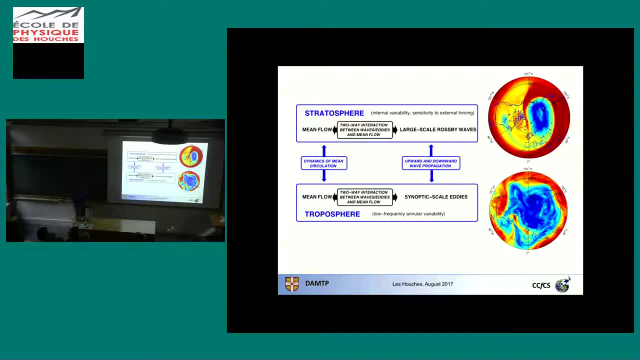 Although, of course, the question is: what sort of linear theory exactly? So just to kind of remind you about the kind of worlds we're talking about here- I mean, in fact, I'm not really going to talk very much about stratospheric dynamics- 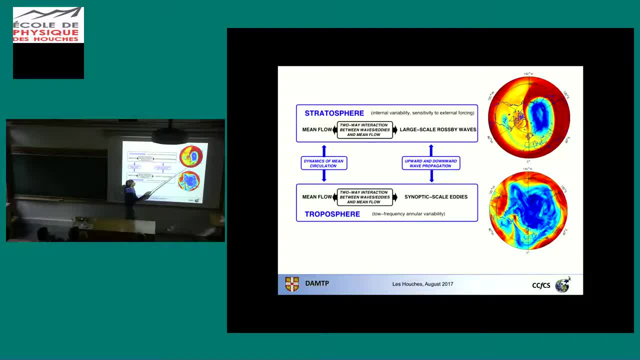 But in the stratosphere we have this sort of large-scale circulation. In the winter we have a vortex. The vortex is kind of displaced and distorted on the large scale, And in the troposphere one has rather smaller scales. These pictures are potential disty. 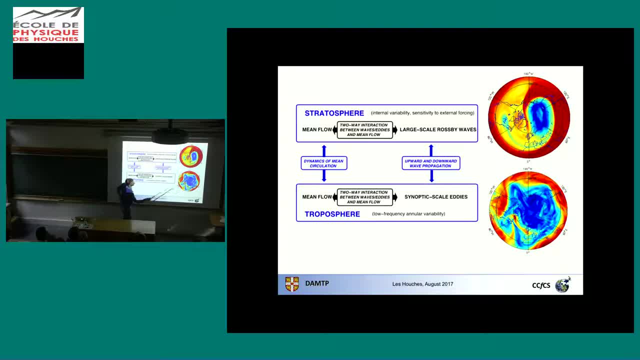 And one sees perturbations of the potential disty field on scales of 1,000 kilometers or so. So we sort of think about planetary-scale waves dominating the stratosphere and baroclinic waves and optic-scale waves dominating in the troposphere. 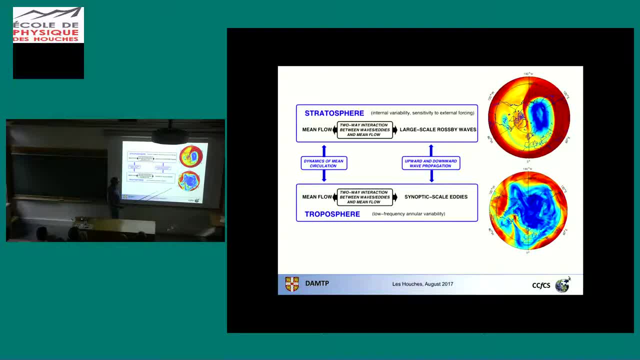 But there is modulation on the large scale as well, which is important, And in each case there's interaction between the mean flux, the mean flow and the eddies in the stratosphere, between the mean flow and large-scale waves in the troposphere, between the mean flow and synoptic-scale eddies. 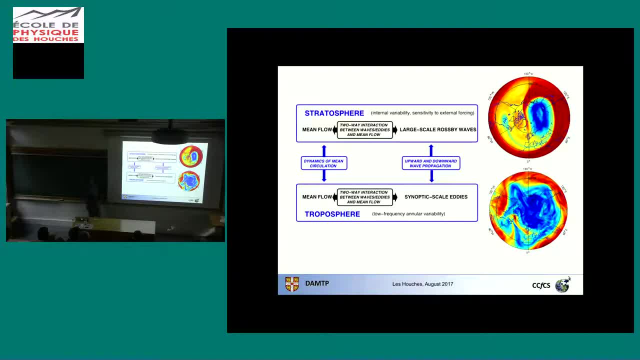 And these lead to important aspects of dynamics, In particular in the troposphere. one thinks of the two-way interaction between the mean flow and the synoptic-scale eddies as leading to sort of low-frequency variability, which people call annual variability because it's typically associated with shifts in the position of the jet. 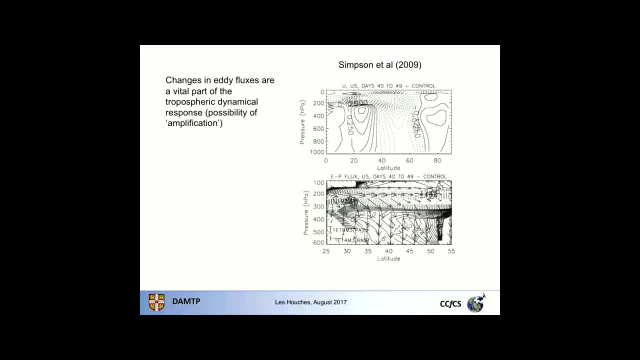 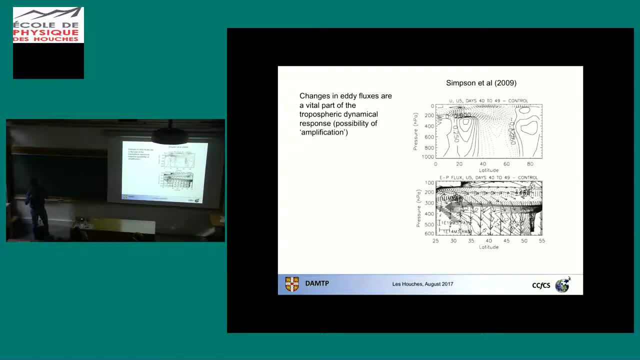 Okay, so going back to the response problem, I mean, what's very clear is that if you're considering the response of the tropospheric circulation to something, then you need to take account of the effect of the eddies, the eddy fluxes. 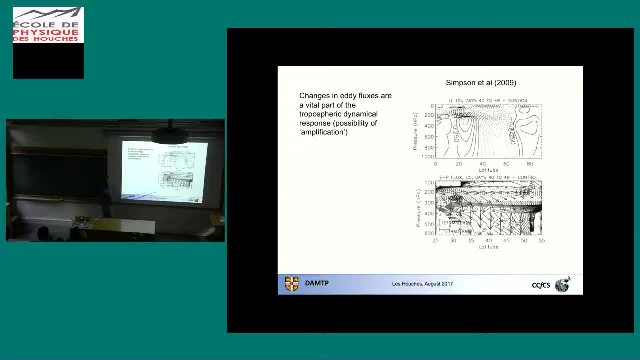 And this is simply a kind of The arrows here and the contours represent kind of standard diagnostics of the effects of the eddies, potential effects of the eddies on the mean flow. So all this slide is saying really is that when you apply a forcing, 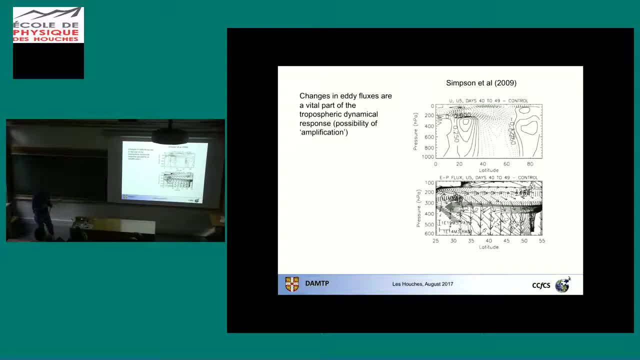 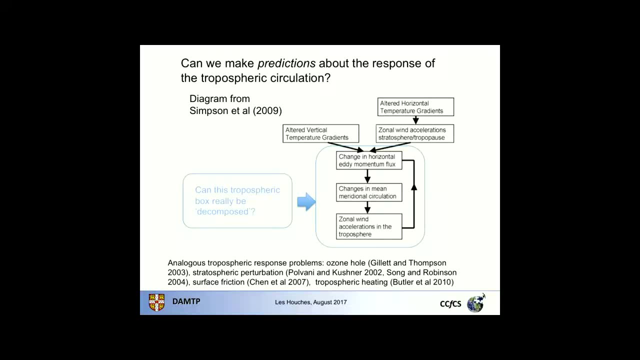 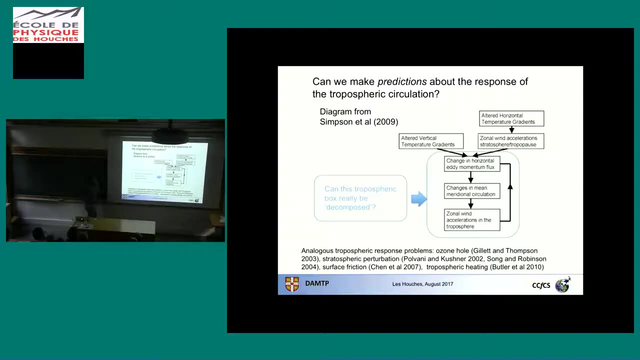 a longitudinally symmetric forcing. you change the eddies and the eddies are likely to have an effect on the mean flow. Now, so the challenge here is that this system is kind of tightly coupled. So Yeah, if we think in the troposphere one's got eddy momentum fluxes or wave activity fluxes. 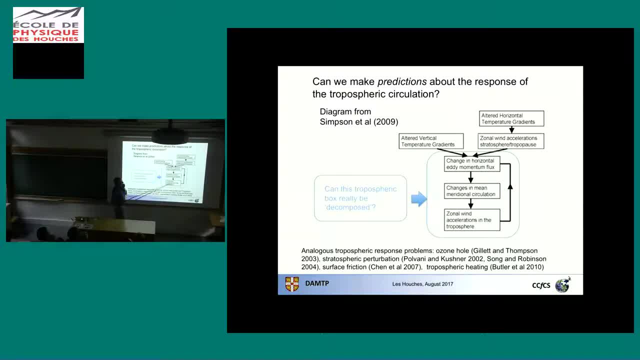 whatever you want to call them. You've got changes in the average zonal wind. You know changes in the eddy fluxes are going to change the zonal wind. Changes in the zonal wind are going to change the eddy fluxes. 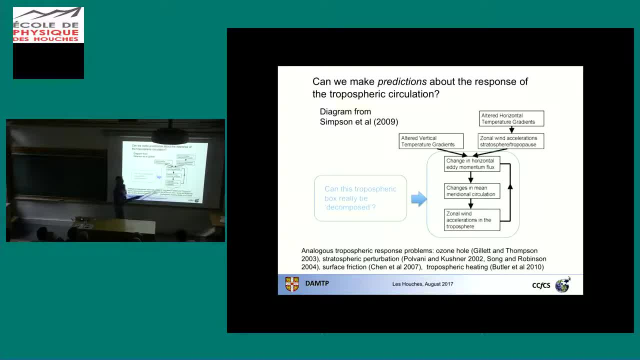 So you've got a sort of rather tight feedback loop here. Okay, And one of the challenges about the sort of experiments that I've, you know, very quickly described, where typically one is applying some zonally symmetric perturbation to the stratosphere or perhaps to the troposphere, is that you know. 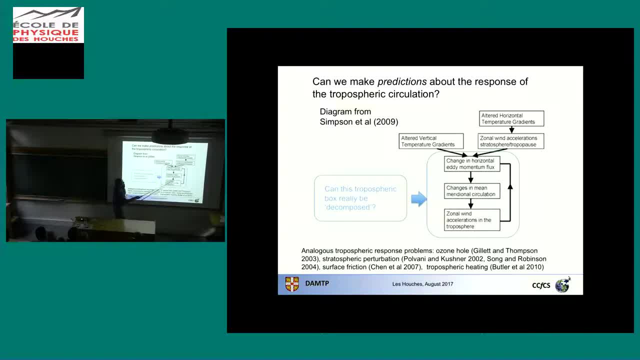 how do you explain the response when you've got this kind of very tight coupling between the eddies and the mean flow? And if we take this paper by Simpson et al as an example? I mean, well, I'm not criticizing this work because this is important work and this is a difficult problem. 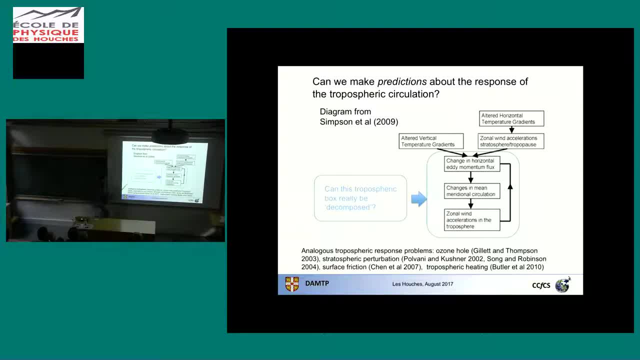 But the fact is that in this paper, for example, I mean, they're applying some kind of changed temperature in the stratosphere and then they're kind of saying: well, it looks like from the diagnostics that that's going to change the eddy fluxes and therefore we're kind of going to get 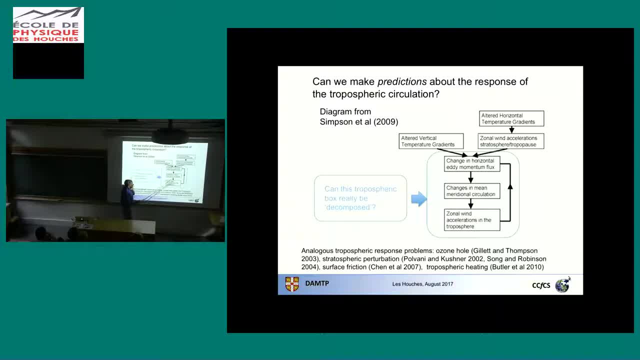 the forcing into the system here and then that's going to affect the mean circulation, that's going to affect the zonal wind. So they're sort of On the basis of empirical evidence and guesswork. they're kind of leaping into this feedback loop. 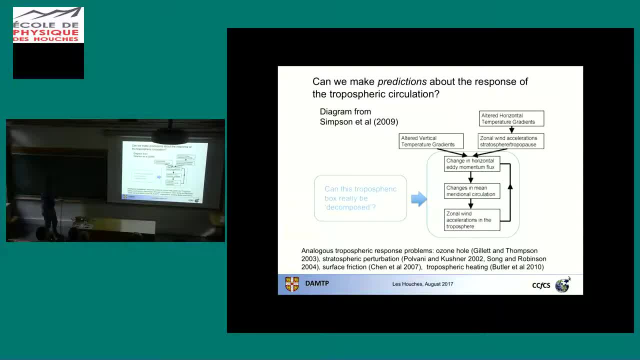 and saying this is the way to understand the response. So the question really is: you know, can you really decompose this tropospheric box, or do you just have to accept that all of these things are changing together? One can make the same comment about you know. 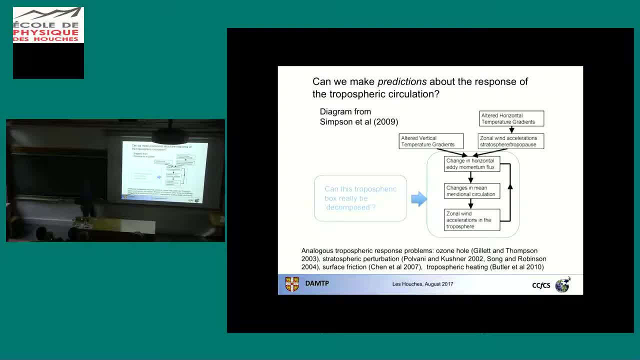 the ozone hole response problem about the effect of the stratosphere in general applying stratospheric perturbations. There are examples where people have perturbed surface friction and looked at the effect of that on the tropospheric circulation. There are cases where people have applied changes in tropospheric heating. 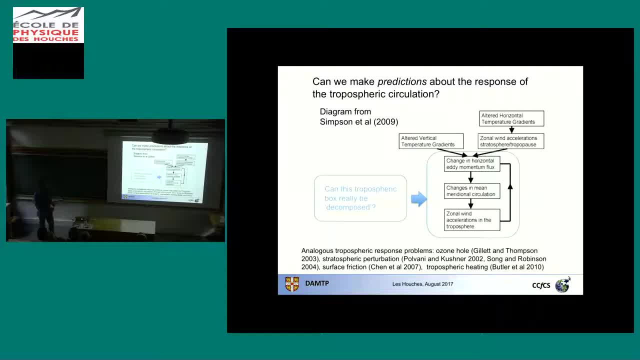 as a kind of simple representation of different sorts of greenhouse gas forcing. All of those have the same problem: that you're applying a forcing. What you want to know is: how do these things change? right? But because these things are kind of tightly coupled, 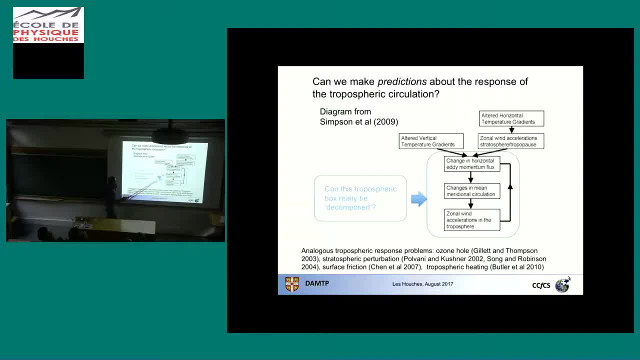 it's not really clear. you know where you get your forcing into this feedback loop. There's a You can say that people do experiments and they see a response and they can sort of post hoc explain that response. But in terms of making a prediction, 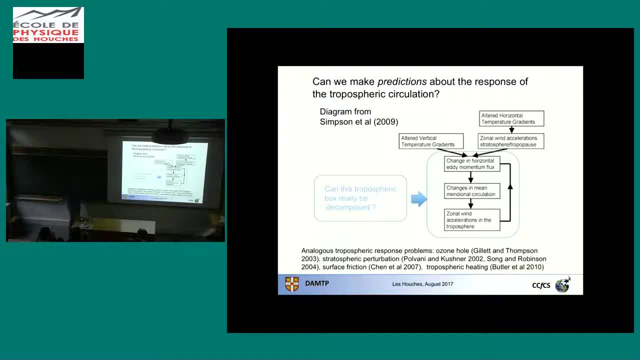 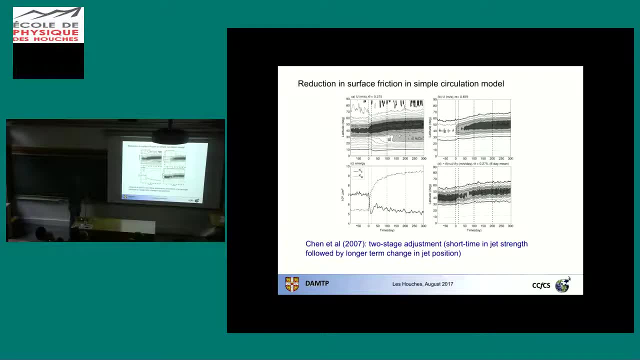 that's not really not really clear that the skill is there to make the prediction. Of course you- I mean you- can. The change is being predicted by a model, but in terms of sort of theoretical, mechanical, fluid mechanical arguments. 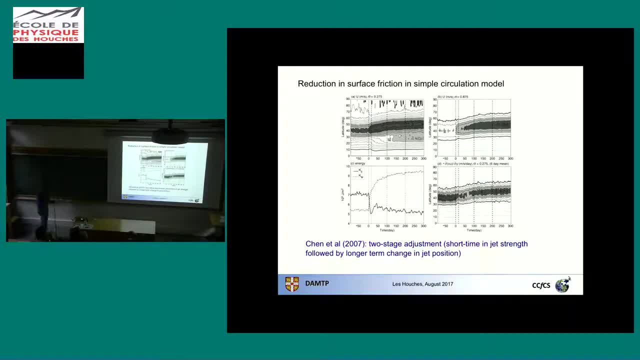 can you make a prediction? This is just another example of how this sort of thing works. I mean, this is a paper by Chen et al where they basically change the surface friction So they have a tropospheric circulation, They have some kind of value of a surface friction parameter. 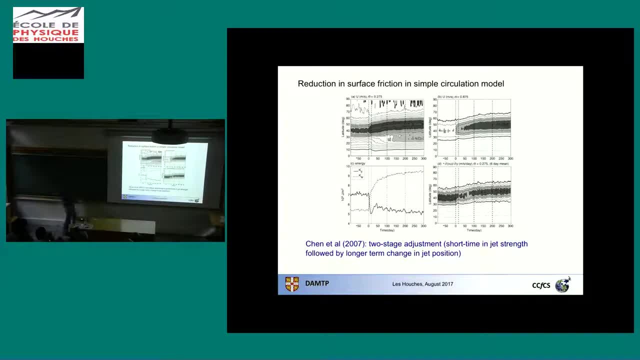 They reduce, They reduce the friction, okay, And then, So what there's a sort of This is the, You know, this sort of upper level wind as a function of latitude. This is where you change the friction, So you sort of get a rather quick acceleration in the winds. 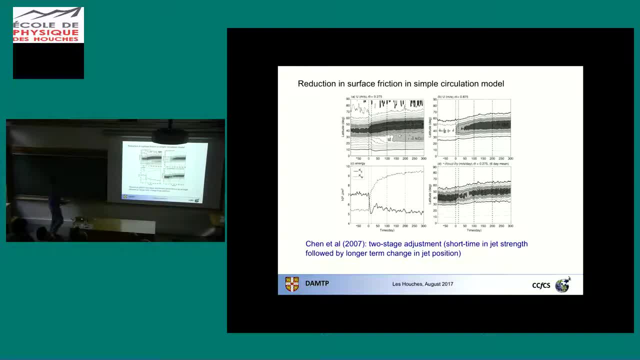 as you might have expected, because you reduce the friction. But then there's a sort of longer and slower adjustment to a new position of the jet, okay, And that adjustment involves both the eddies and the mean flow In this sort of tightly coupled response. 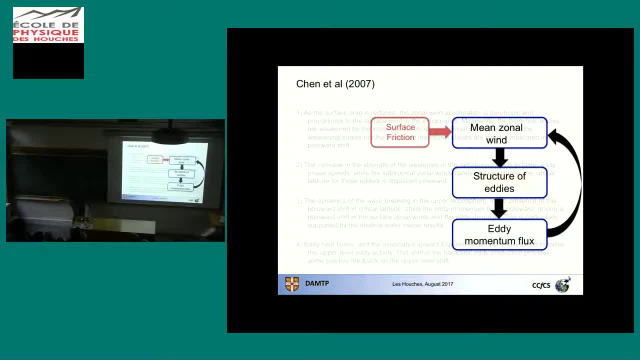 And again, I mean Chen et al had a kind of complicated story about how this worked. okay, I mean, they had the same kind of feedback loop in the troposphere. but they sort of said, okay, well, we think that the surface friction 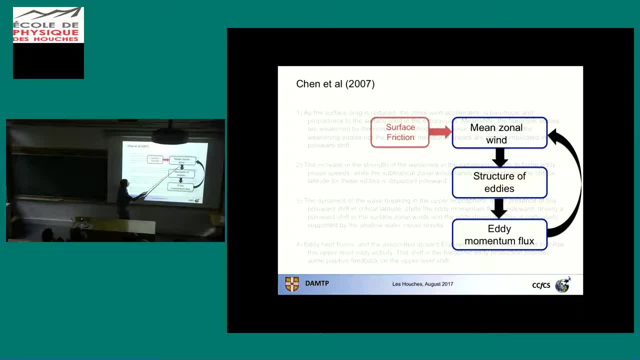 is kind of getting into the system here. It's changing the winds, Therefore that changes the structure of the eddies, That changes the eddy momentum flux, But it sort of It's a sort of post-hoc description rather than a prediction made in advance. 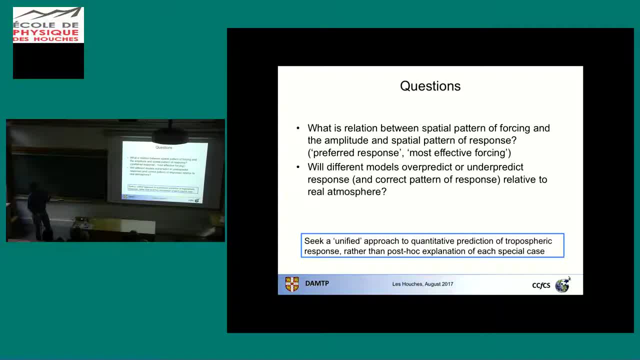 Okay, now the question that one is asking, The question one would like to answer in these sorts of problems is: what's the relation between the spatial pattern of the forcing and the amplitude of the response and the spatial pattern of the response? okay, 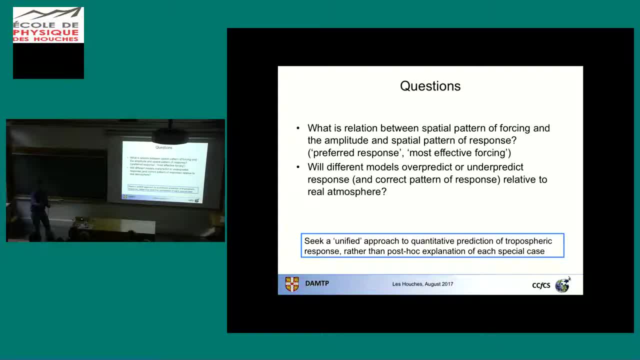 You know, we've seen examples where the jet shifts pulsates. We've seen examples where the jet shifts equate-award. Is there a kind of preferred response, you know so that many forcings give similar patterns of response? Is there a sort of most effective forcing? 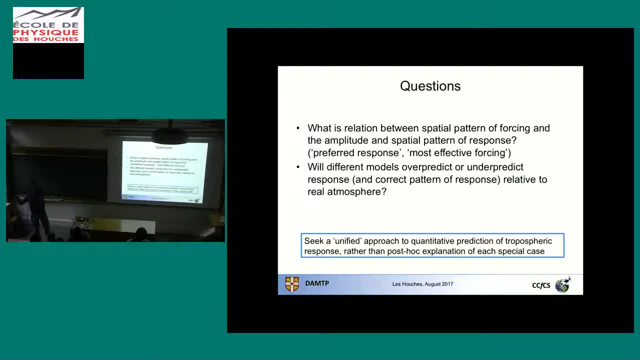 So if I have a certain amount of forcing, can I sort of, If I put it in one place, do I get a bigger response than if I put it somewhere else? You might also sort of think about the question of what you know what models do. 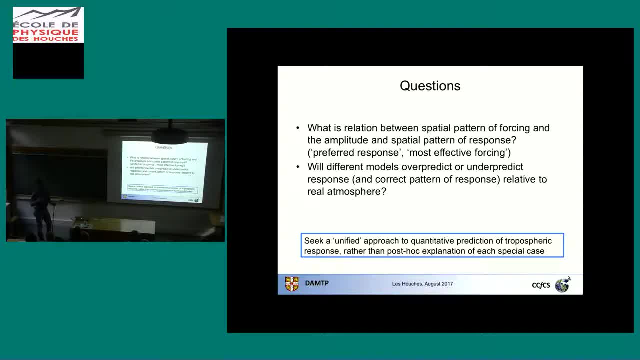 I mean, if I take two models of the atmosphere, two climate models, perhaps you know, do those model? How do those, The predictions made by those models, relate to each other? How do they relate to what the real atmosphere does? 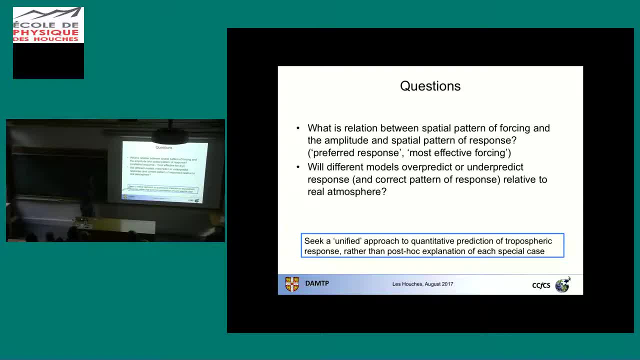 So I mean, what I'm going to talk about is this sort of- It's almost a non-dynamical approach, right, But it's, you know, it's an approach. What one really wants to do is one wants to make a prediction. 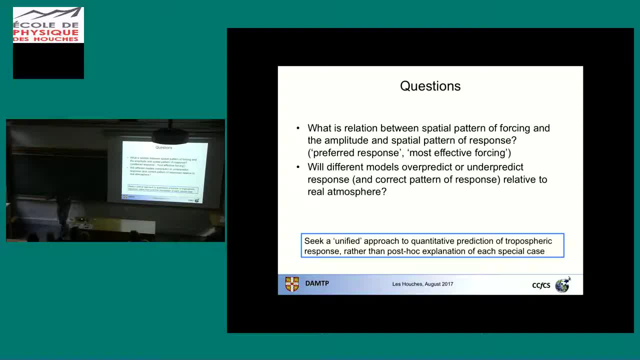 of the Traub's ray response, rather than doing an experiment and afterwards saying: oh, we sort of understand how this all works, because we see the eddies change and we see the mean flow change. Okay, so this is where the fluctuation-dissipation theorem comes in. 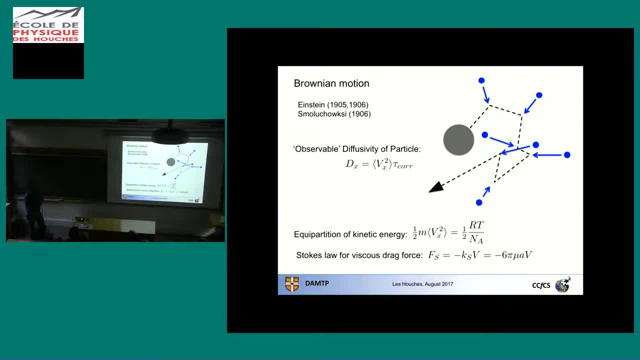 So this is a kind of historical aside about what the fluctuation-dissipation theorem is. So this was a kind of, you know, one of Einstein's classic papers And it was about Brownian motion essentially, And you know he was considering the phenomenon of Brownian motion. 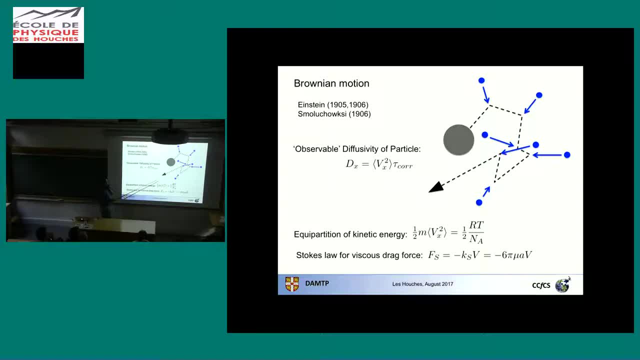 which had been identified previously. So we have a particle in some kind of liquid And, you know, the idea is that the molecules in the liquid are making collisions with the particle, And so what I see is that the particle executes some kind of random walk. 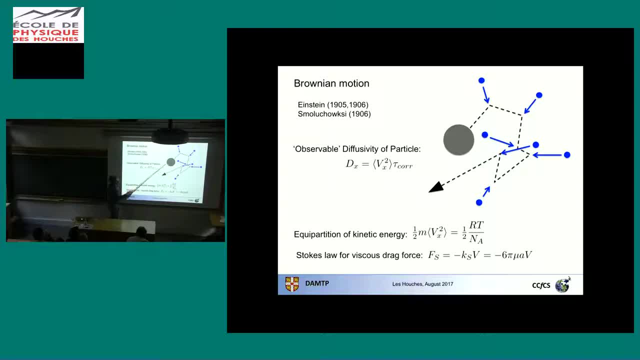 And the random walk made by the particle, let's say it's sort of sphere, can be described by diffusivity. okay, And the diffusivity is the mean square velocity fluctuation multiplied by the correlation time of the velocity fluctuation. 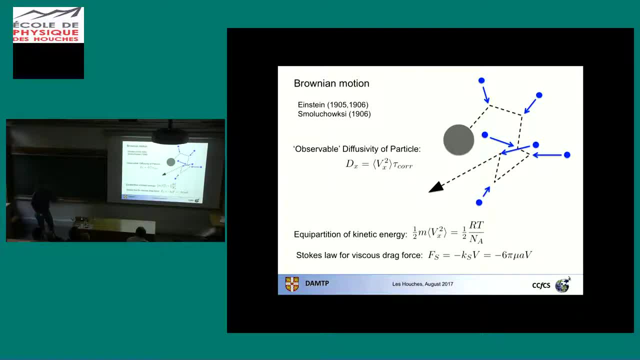 So then Einstein kind of took various bits of physics and put them all together, And one piece of physics he used was from thermodynamics, the idea of equal partition of energy, And basically he said that the average kinetic energy of the sphere would be the same as the average kinetic energy of each individual molecules. 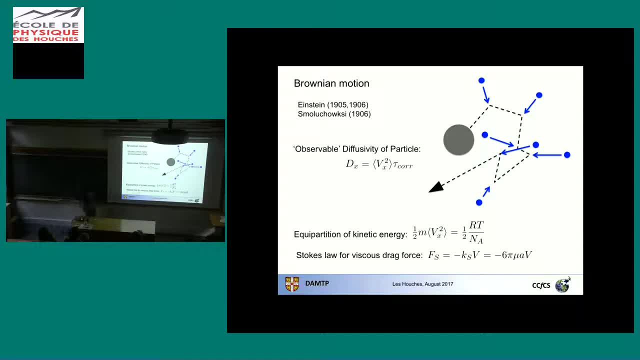 Okay, And so that led him to this expression for the kinetic energy of the sphere, And this is accurate. This is Avogadro's number here, right? So this is a kind of important number in physics which is appearing in this expression. 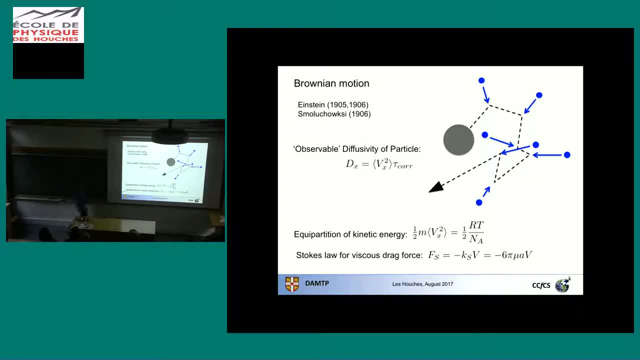 Now, he then also used the Stokes law, you know, which had been derived a few decades earlier, which was said that the force on a sphere in a viscous fluid is linearly proportional to the velocity, and in fact it's actually. 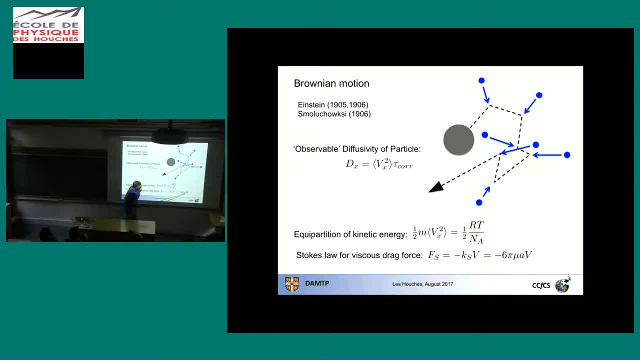 the constant of proportionality is actually this thing here, involving the size of the sphere and the viscosity of the fluid. Now, in order to predict the diffusivity, okay, well, we've got the mean square velocity, but what we need is the correlation time for the velocity fluctuations. 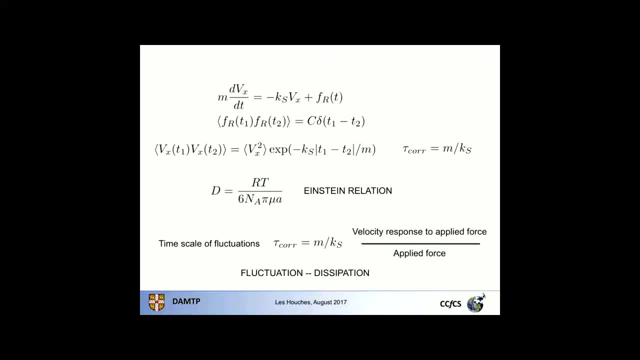 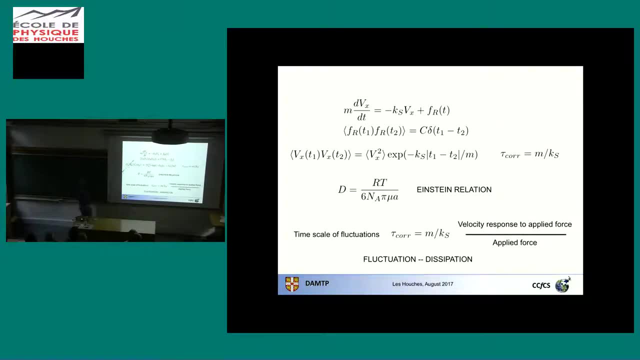 And Einstein, you know, derived that by considering a simple kind of Langevin equation saying: well, this is the equation for the motion of the sphere, so the mass times, the acceleration of the sphere, is equal to the minus the resistance force. 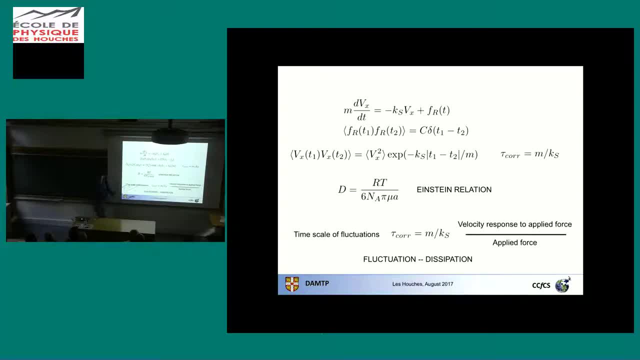 plus some kind of random force which is being exerted by the collisions of the molecules. We assume that this random force is delta-correlated, and what that leads you to is the fact that the time correlation- I mean this- is the lag covariance of the velocity of the sphere. 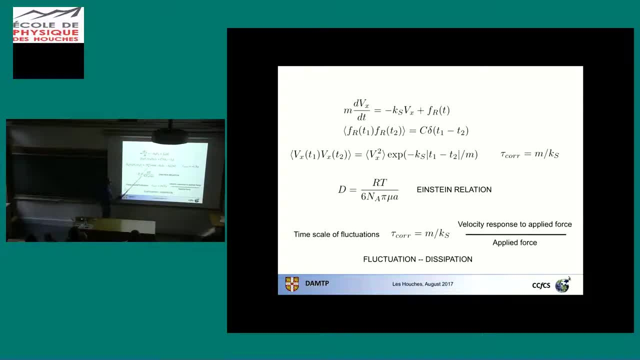 is equal to the mean square velocity of the sphere multiplied by this exponential in time difference, and the time scale which appears here is m over ks. so it's the mass of the sphere divided by the, you know, the drag constant, if you like. 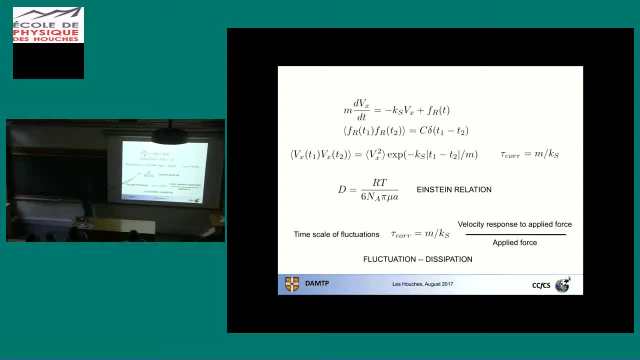 So, then, Einstein put all this together, and what he found was an expression for the diffusivity in terms of well-known quantities like the gas, constant temperature, the viscosity, the radius of the sphere, but also Avogadro's number right. 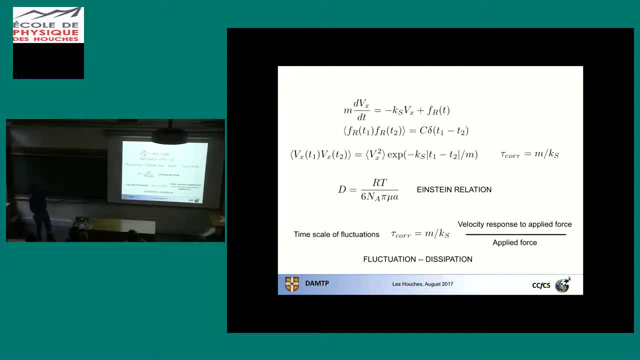 So the kind of one of the main big contributions of this piece of work was that you have a sort of macroscopic observable involving Avogadro's number so you can estimate Avogadro's number. and this was a time when actually the whole idea of 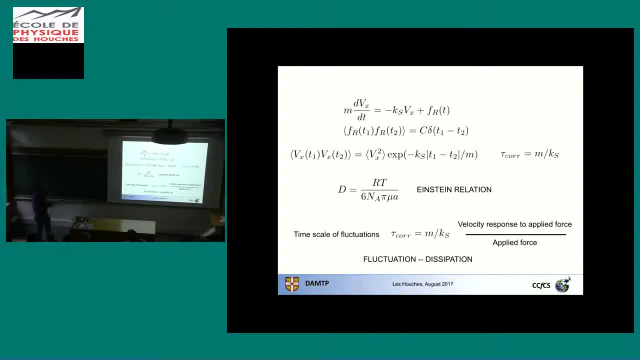 you know the sort of particular. the atomic or molecular nature of matter was still quite controversial. so, if you like, displaying verifying this relation was a way of verifying the molecular theory of matter, or whatever. So Einstein didn't get a Nobel Prize for this work. 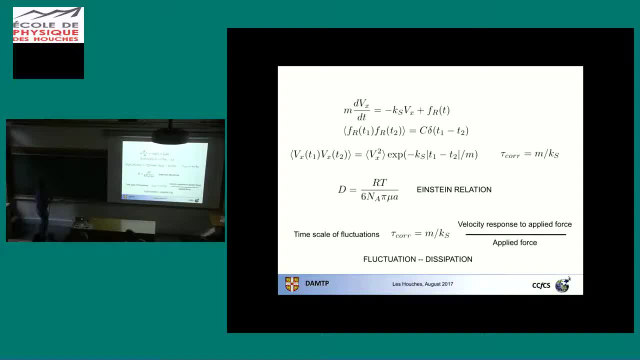 but someone else did later, for you know, some kind of experimental continuation of this. So that's all kind of interesting, but then let's go back to the problem that we're interested in. Well, the important point here is that is this time scale of fluctuations. okay, 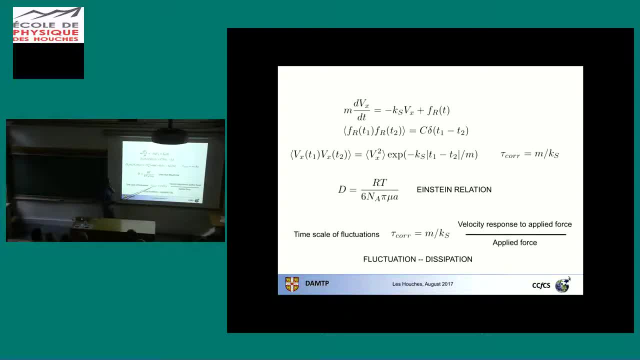 So that the time scale for the fluctuations in velocity is simply this mass divided by the resistance force, and this is basically the ratio of the velocity response to an applied force over an applied force. all right, So M and Ks were first of all appearing in. 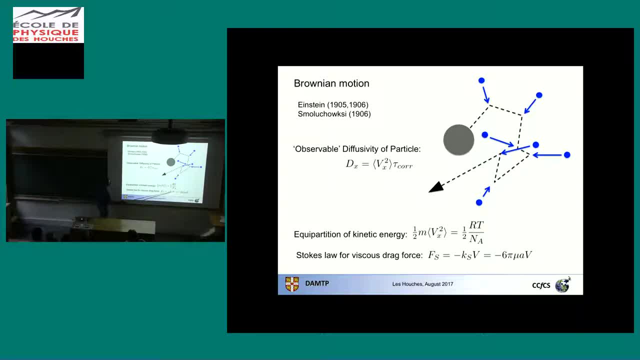 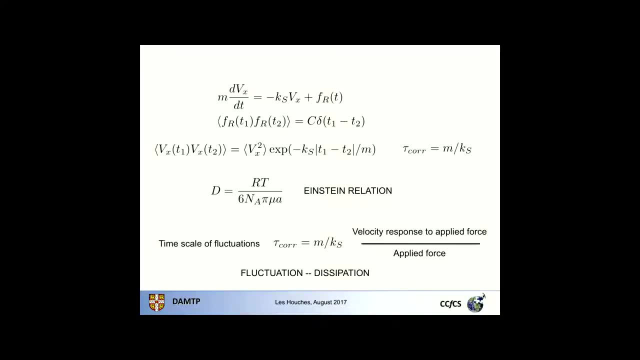 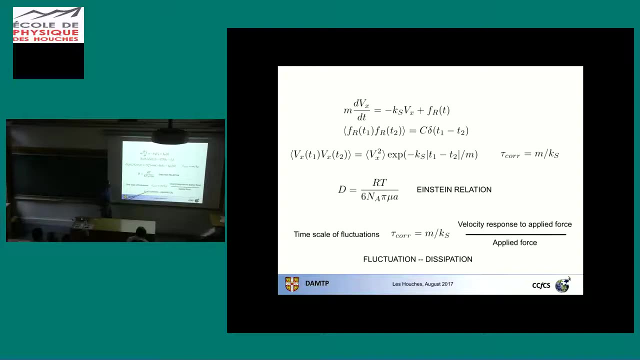 you know the idea of a sphere moving steadily with a force exerted on it, and are now appearing in an expression for the time scale of the fluctuations. So there's a relation here between a characteristic of the fluctuation and the dissipation of energy. 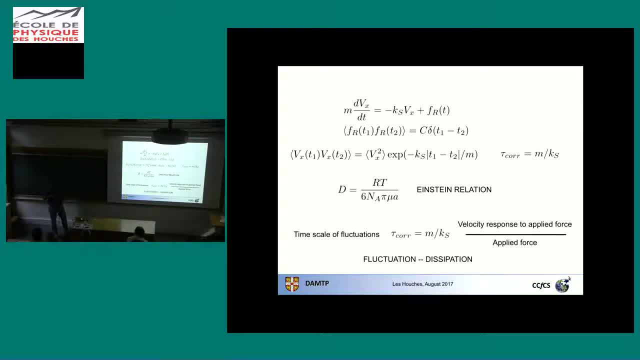 as expressed by the resistance force, by the rate of. you know, if you apply a force on a sphere, you do work which is dissipated okay, Hence the name fluctuation dissipation. But the important insight is that the correlation time for the fluctuations 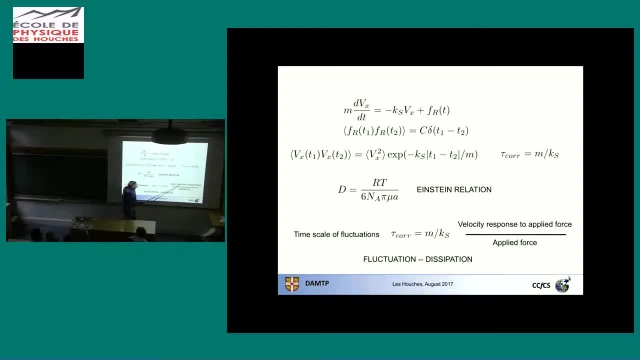 is given by the response of the system to an applied force, divided by the applied force. Now, in the world of climate, response all right, or any other response problem. actually, we are interested in this quantity, We are interested in how much response you get for a given forcing. 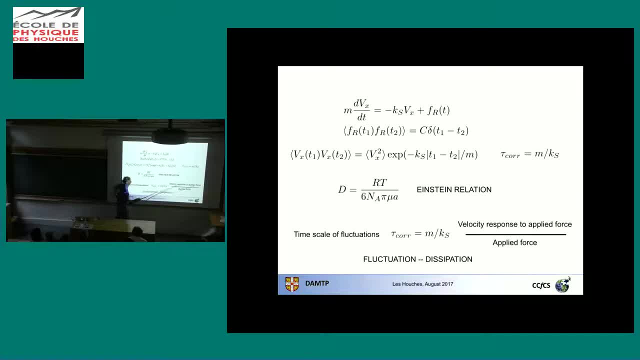 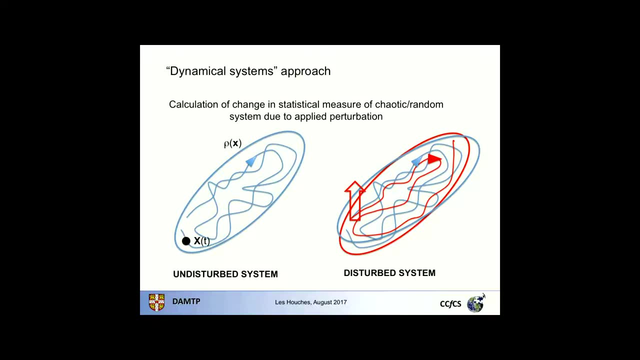 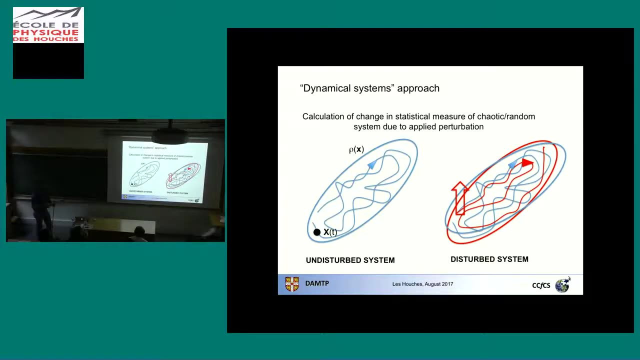 So the question then is: can we get insight into this thing by looking at the correlation time of the fluctuations? Okay, now let's sort of move viewpoint a bit. If I'm thinking about so you know, I'm thinking of the tropospheric system here. 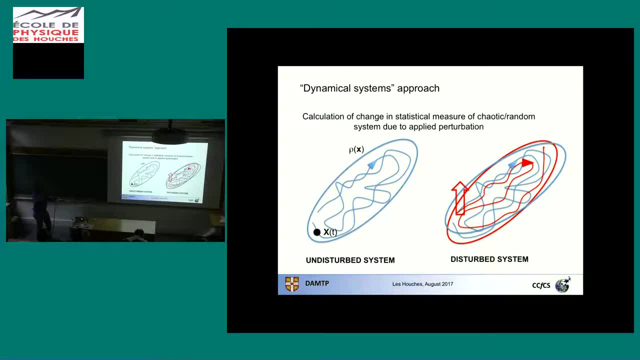 as a chaotic system. okay, So it's. you know it's executing its random, quasi-random evolution. I can think of that, as you know, represented in some kind of phase space, The position of the system in the phase space. 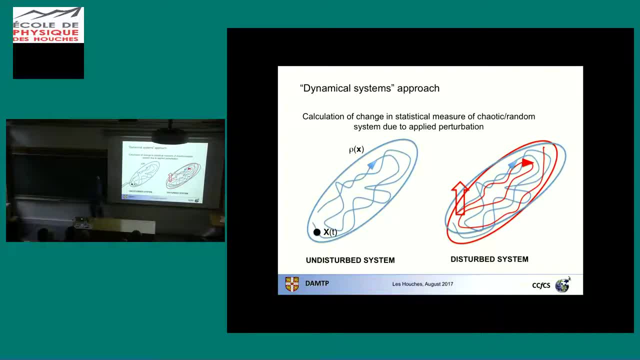 is represented by some probability density function, If you like. the probability density function in the phase space is the climate, And so this is my undisturbed system. okay, And then what I'm going to do is I'm going to apply some kind of forcing to this system. 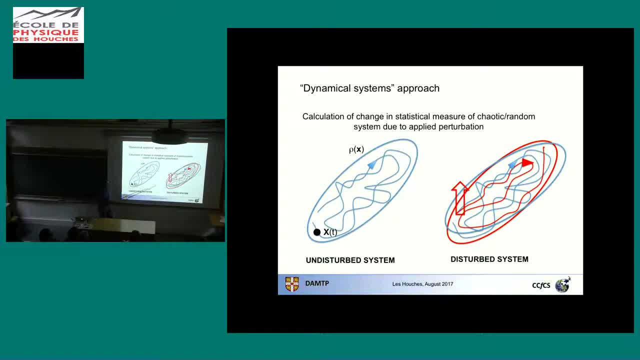 And, of course, every individual trajectory will be affected by the forcing And correspondingly, the probability density function will also be affected by the forcing. So the question is: how does the probability density function change as a result of applying the forcing? So yeah, writing that mathematically. 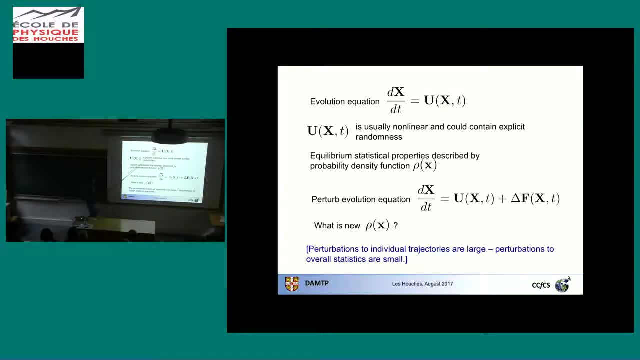 yeah, we're considering some kind of evolution equation in some kind of phase space. Yeah, we could imagine that the system behaves kind of quasi-randomly because this is a nonlinear function, or else we could incorporate some kind of explicit randomness into this evolution equation. 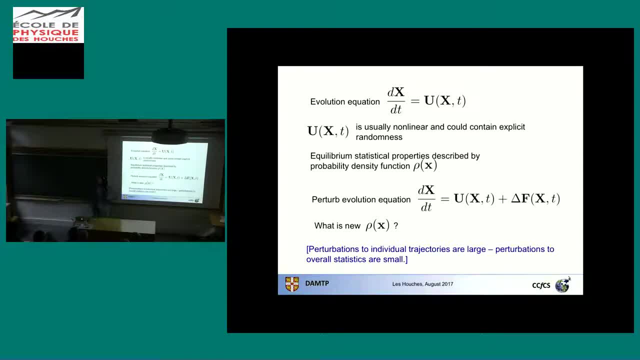 We imagine that there's a probability density function which describes the equilibrium statistical properties. We're going to perturb the evolution equation by applying a forcing term. And what's the new probability density function I mean? one important point here is that I mean in these systems. 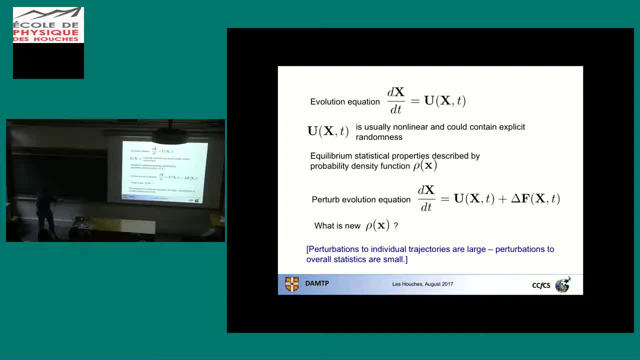 we expect that trajectories are going to be chaotic. So if we apply a small perturbation to the system, individual trajectories will eventually diverge, right. So individual trajectories will not be describable by some kind of linear theory. But on the other hand, 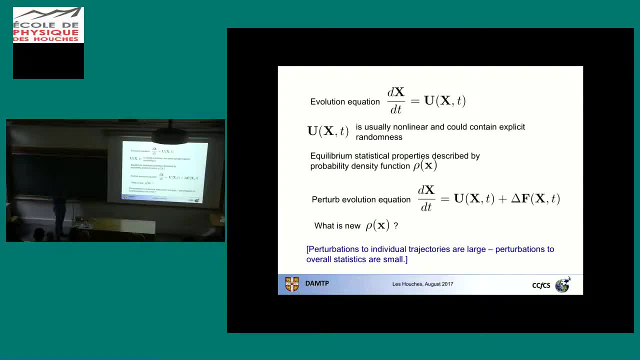 we might imagine that the statistics of the system changes only weekly, so that we're applying a linear theory to the statistics but not to individual trajectories, And this is a subtlety which has been discussed in statistical physics. There's something called Van Kampen's objection. 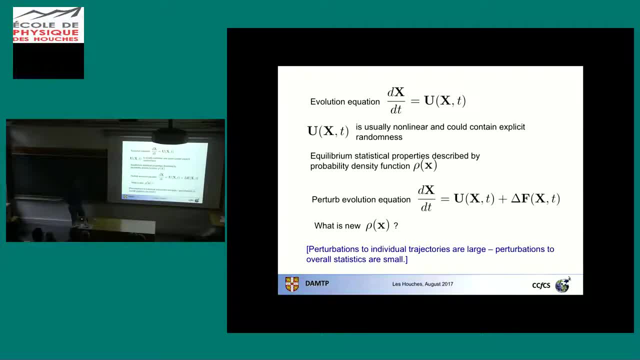 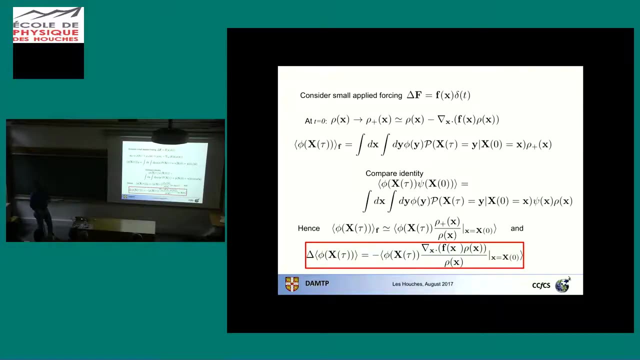 which was basically saying you can't apply linear theory to chaotic systems, right? Well, you can if you, provided that you take some kind of statistical average first. Okay, so the key step here is to sort of say we wanted to do a problem where we were applying. 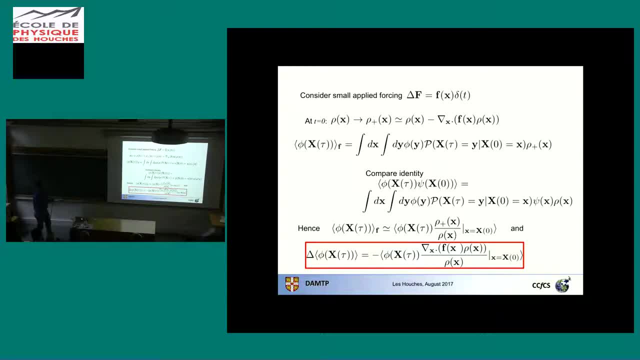 some kind of, let's say, steady forcing, but it could be a forcing that was a function of time. We're describing this in terms of a linear theory, so let's consider a delta function in time forcing and then superpose lots of delta functions. 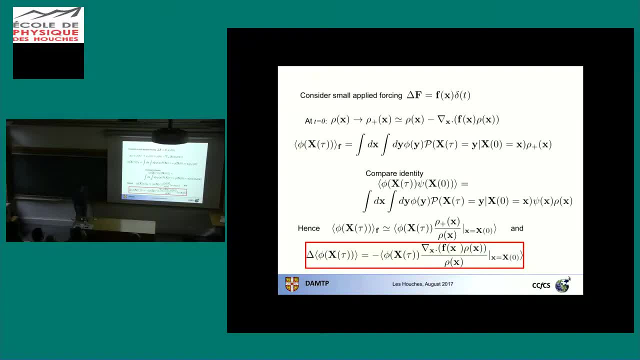 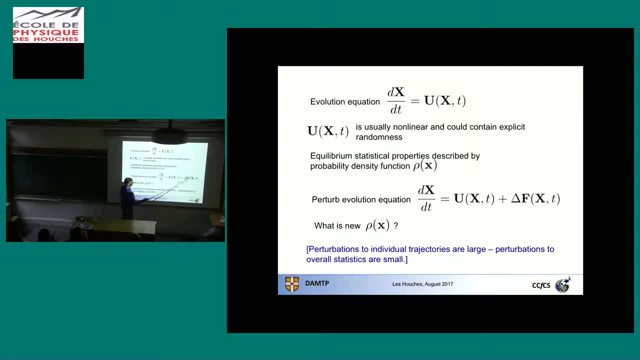 Now, as we kind of all learn from studying differential equations. if I apply a delta function forcing in this equation, then the effect is basically to kind of shift the trajectory by a finite amount from before the delta function to after it. Okay, So what that's essentially doing is 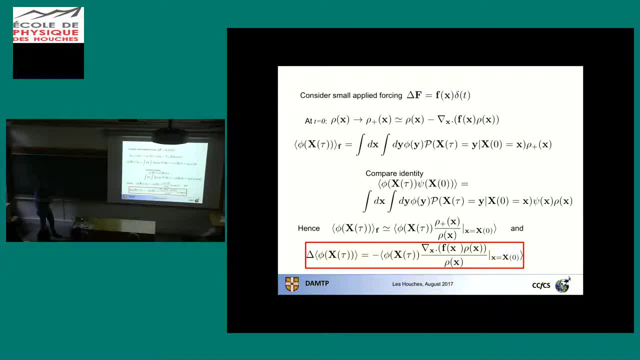 I mean, I'm starting off in a situation where the system is in its standard equilibrium statistics. So let's imagine I've got many, many copies of the system each doing its own thing, and then I apply the delta function forcing, and in each of those systems 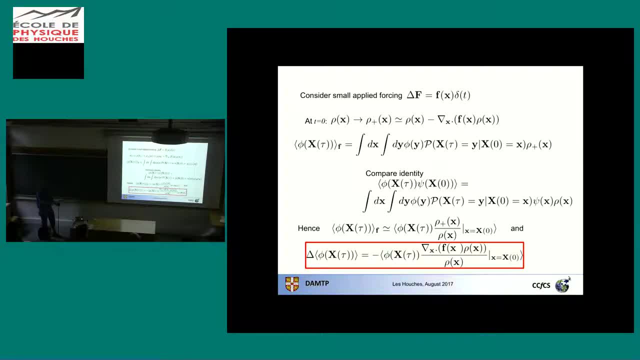 the trajectory is displaced, okay, by an amount which is proportional to the forcing, And then I again take the average and I get the new probability density function. So the, you know, just before the delta function, forcing is applied. 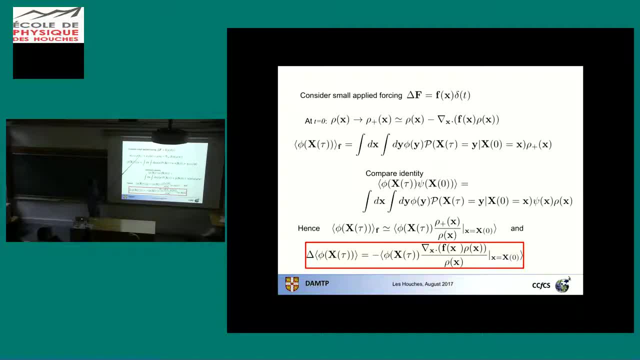 I've got the equilibrium probability density function and then, after the delta function forcing is applied, I've got a new probability density function and there's probably a delta T missing here. but basically that's. you know, I can write down an expression for the new probability density function. 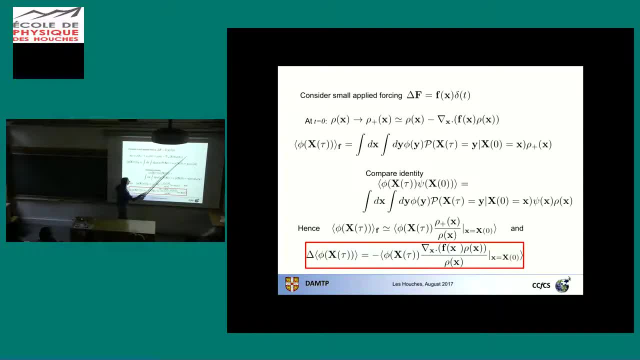 the new probability density function in terms of the old. There should be a delta T here. So then, if I now think about, if I now think about a sort of observable of the system, so some function, the average value of some function of x at time, tor. 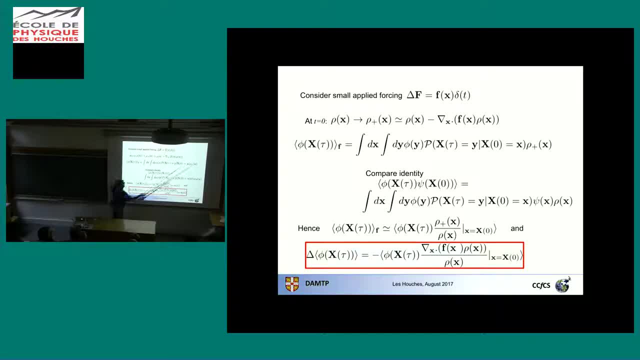 okay, I can write this down as this integral over the, the probability density function of the system just after time zero, and there's also a probability density function describing the evolution from the position at zero to the position at tor. So this is now what I want. 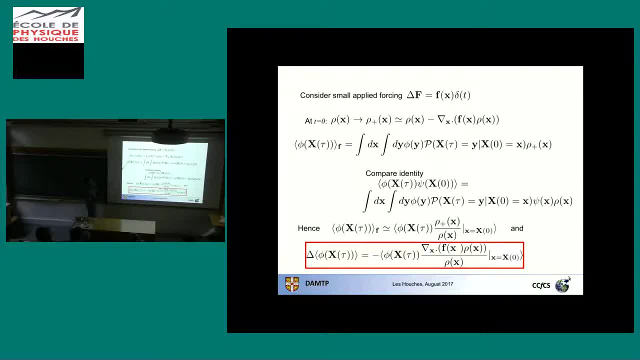 what I want to know is: what is the change in the observable associated with the forcing? okay Now. so then you can kind of exploit an identity. you know this is an identity which holds for all phi and psi. It expresses this lagged expectation of the product of phi and psi. 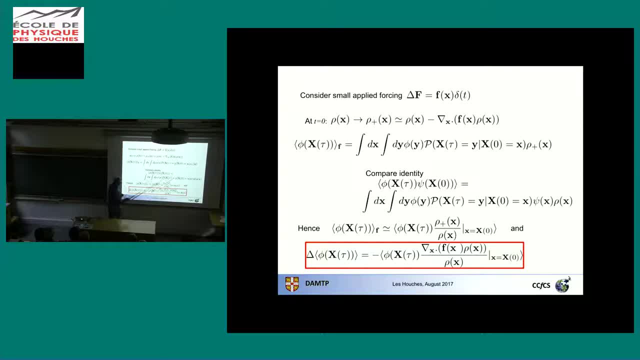 in terms of, again, these conditional probability density functions and the sort of equilibrium probability density function and the function psi and the function phi, and you can choose a psi, so that what you get is this expression here, And so what you can end up deducing is that the change in the observable 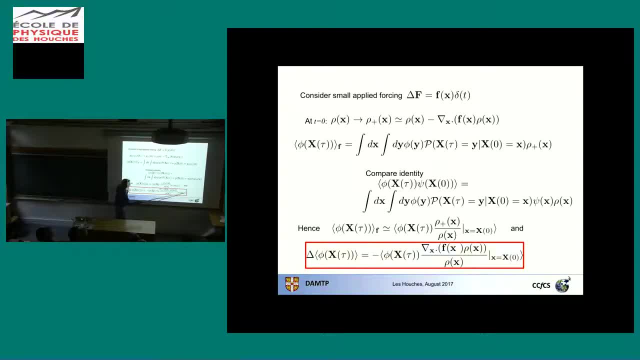 is equal to this expectation. okay, And so this expectation is of phi evaluated at x of tor and then this function evaluated at x of zero, right? So this is all about lagged correlations, And it's about lagged correlations in the equilibrium unforced. 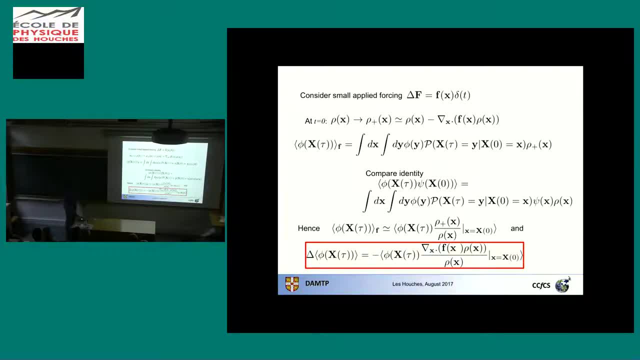 you know the unforced system. So this, so the, what you have here is an expression for the change in observable under the application of a delta function force in terms of lagged correlations evaluated for the unforced system. And then, if you now do the integral in time, 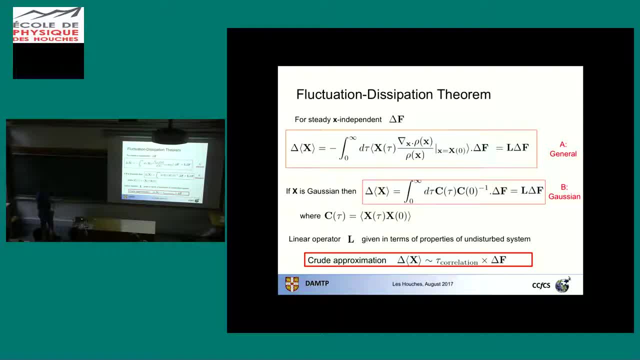 this leads you to the sort of simple formula, along with the fluctuation dissipation theorem. And so let's take a simple observable which is just the change in the position, so to speak, in phase space, And that change is a linear operator. 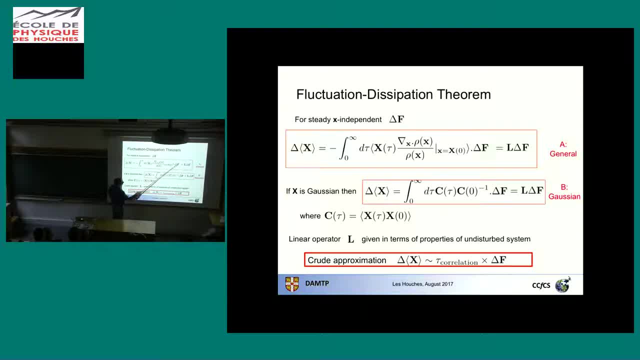 which is this operator here acting on the forcing, And this linear operator involves lagged correlations evaluated in the unforced system. Okay, now the complicated. this is a general expression. okay, So it holds for all systems, provided I know the probability density function rho. 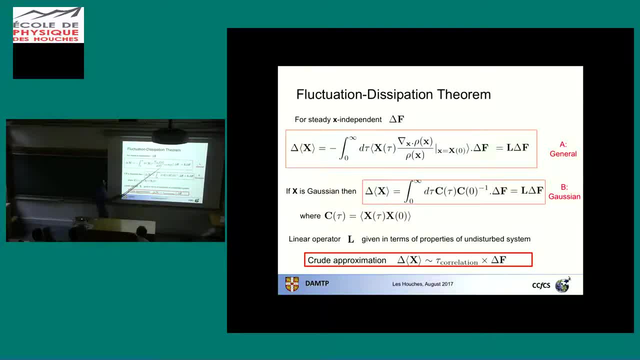 There's a nice simplification that if rho is Gaussian, then this expression here reduces to essentially, you know, some constant matrix times x of zero. And so in the special case that the probability density function is Gaussian, then what one has is that the change in x. 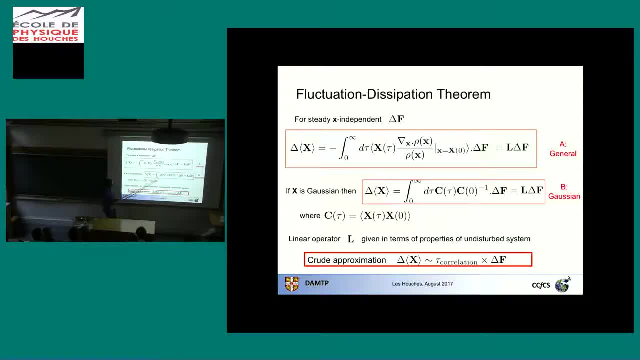 the exploitation of x is given by this expression in terms of the covariance matrices. Okay, so one now has one's operator, which takes you from the forcing to the change in the simple observable, And the operator can be evaluated if you know these covariances. 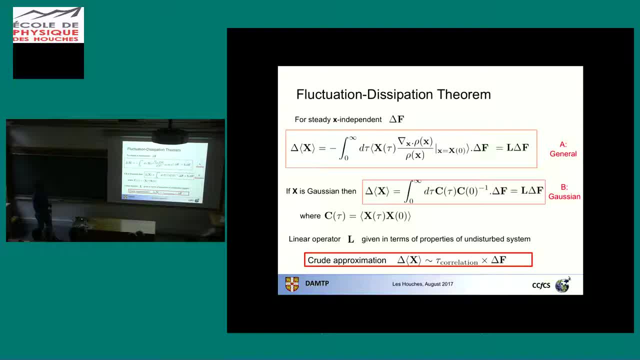 for the unforced system. Now, in very crude terms. I mean this thing here is a kind of time integral of a correlation function, of a covariance divided by the variance right. So this is, it's a sort of measure of memory time of the system. 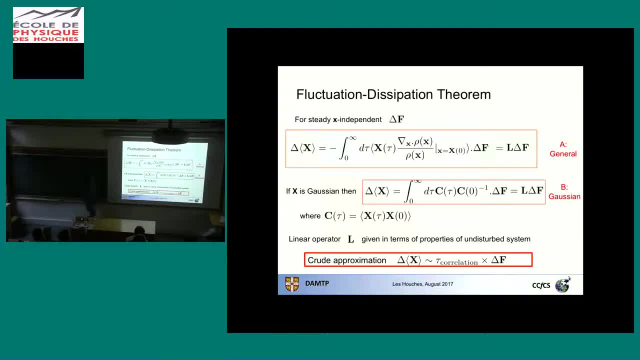 So the kind of very crude insight from this would be that the change in the observable is is the correlation time, although perhaps the longest correlation time in the system, because if you've got a system of many dimensions, you have many correlation times. 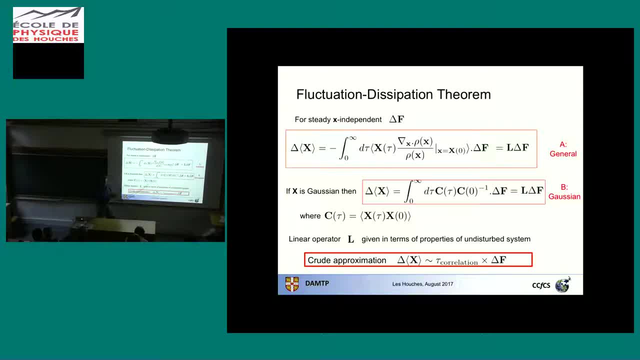 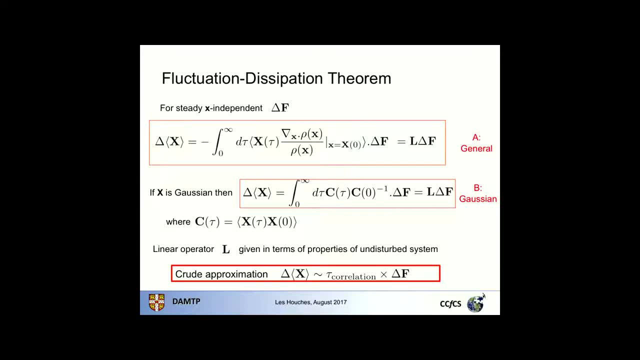 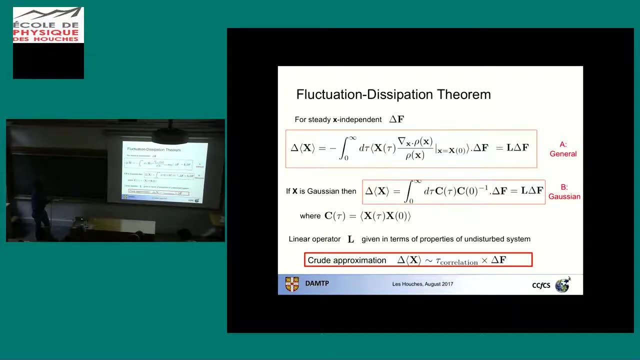 multiplied by the forcing right. So this makes kind of intuitive sense. Okay, so now the question is: well, can one apply this to the climate system? Okay, and there was a paper by Leith, I think in 1975,. 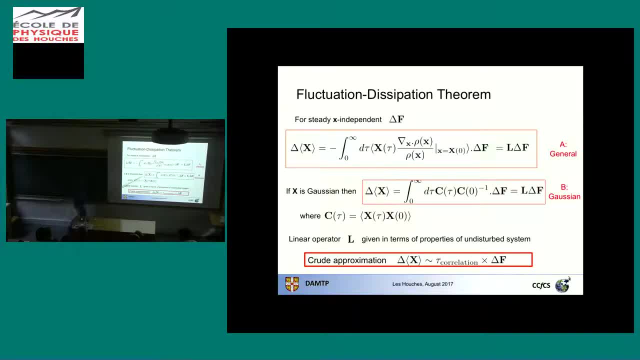 that proposed the fluctuation dissipation theorem in its Gaussian form, because this is the form which you know tends to be sort of most used in standard physics. Yeah, I find it helpful if you could return to the problem you originally posed. 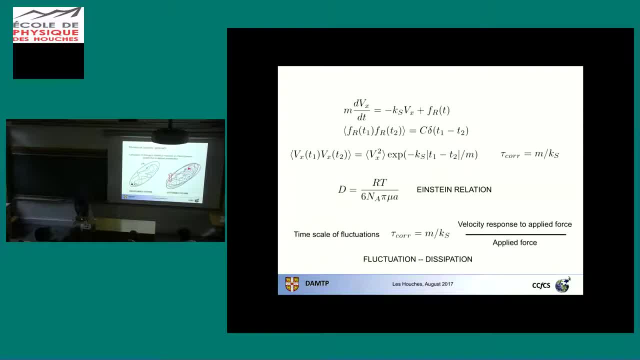 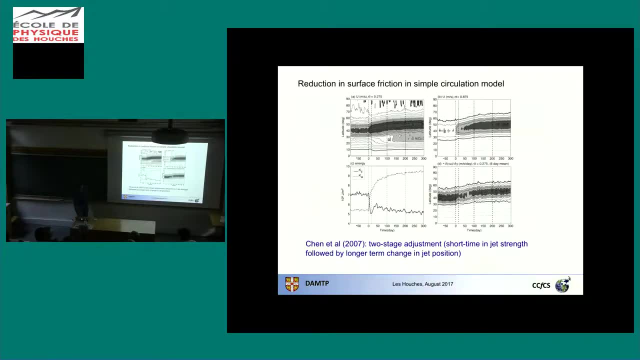 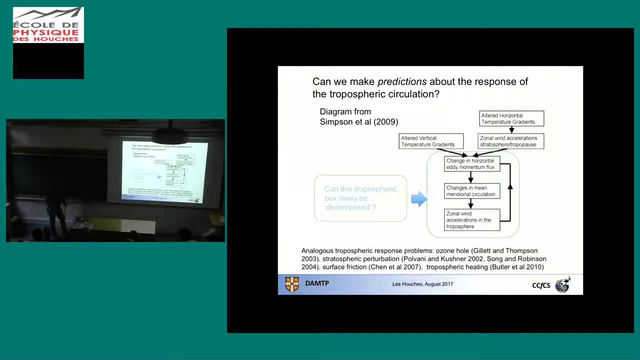 which was breaking into this feedback loop Is now a good time to discuss how this. I think what I'm saying is that I mean I'm breaking into the. The reason why people try to break into the feedback loop is because they're trying to predict the response right. 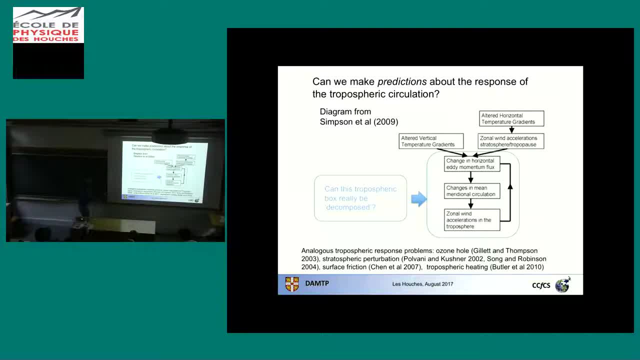 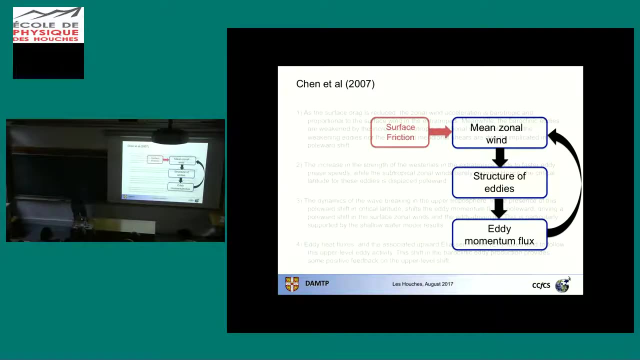 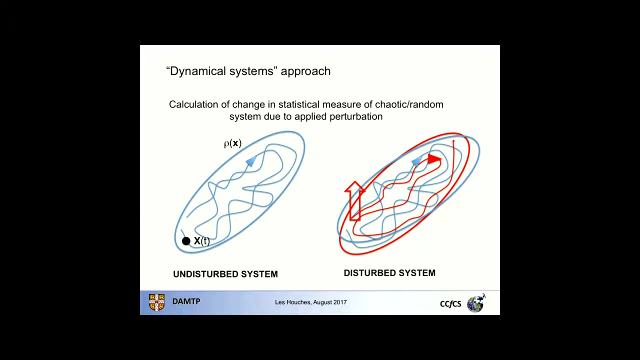 So I'm, if you like, saying: breaking into the feedback loop isn't leading me anywhere. Therefore, I'm going to try something different. Yes, Yeah, well, the key is. so I mean, That's right, there was a sort of break, right. 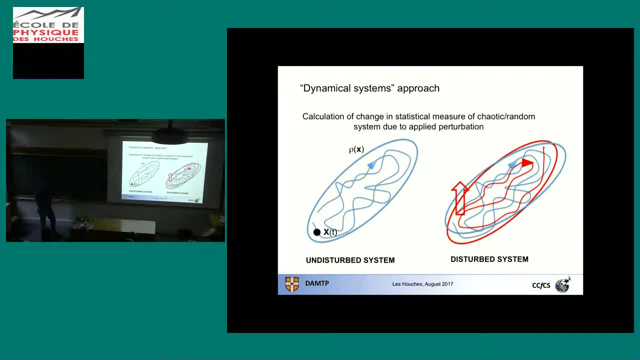 I mean, I talked about something that was sort of recognizable atmospheric dynamics, right, And now I've kind of stopped and I've said this isn't going anywhere, Let's come from another direction. But later on I will go back to the relation to atmospheric dynamics. 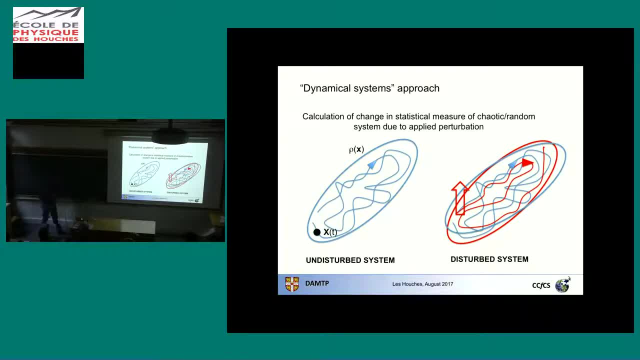 So some people try to do this problem by using the adjoint Of: Yeah, using an adjoint model. that's right, And so it looks like those gradient of the probability function look a bit like the gradient of the. It's not quite the same. 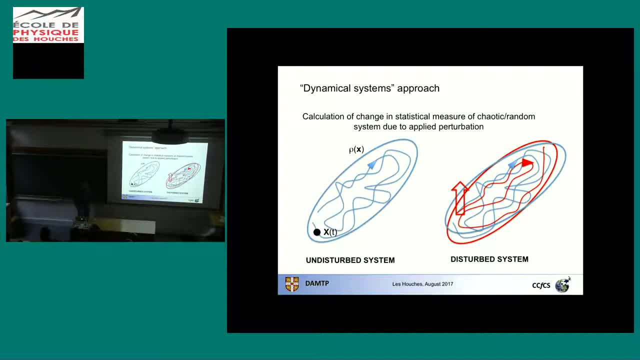 Yeah, I mean so. But one could address the problem of what the response is to forcing by looking at the adjoint. Yeah, but the fundamental problem there is that the adjoint approach is based on linearization of individual trajectories. About individual trajectories: 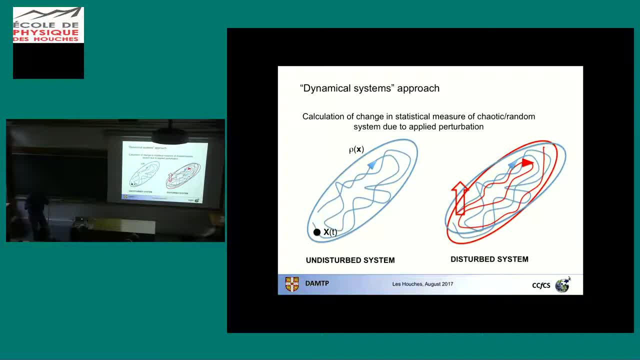 So if you have a world where, If you have a chaotic system, then your linearization about individual trajectories is only going to work for a finite time. Okay, so there is a fundamental technical problem with You. could write down an expression for the response? 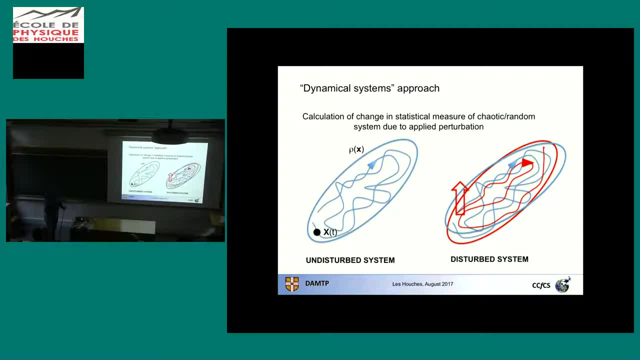 in terms of linearization, about trajectories, But the problem is that you know the size of the things that you were trying to estimate would become larger and larger and larger, So you would have a kind of convergence problem. Okay, so that. 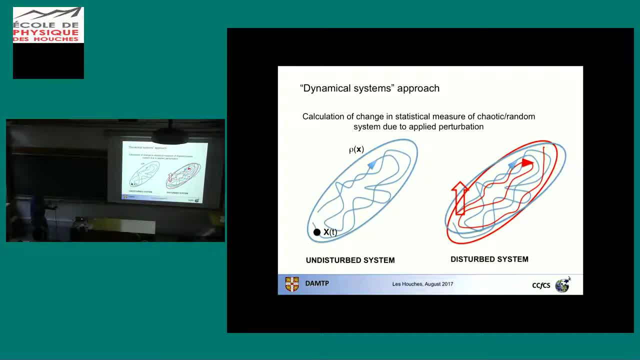 That doesn't get you anywhere. It's a fundamentally time-limited problem And I mean there is- Yeah, there are- people who've tried to resolve that. I mean so there's a, I mean some work by Meider and Abramov. 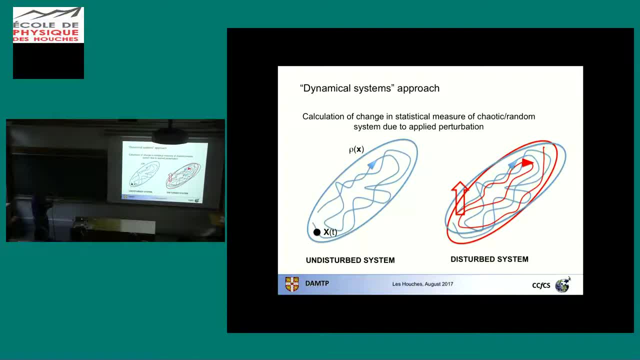 have done something called blended response theory right Where they, Where they basically use an adjoint approach, essentially linearizing about trajectories for some time, And when they kind of hit the barrier, they then say, well, we're going to use some other approach. 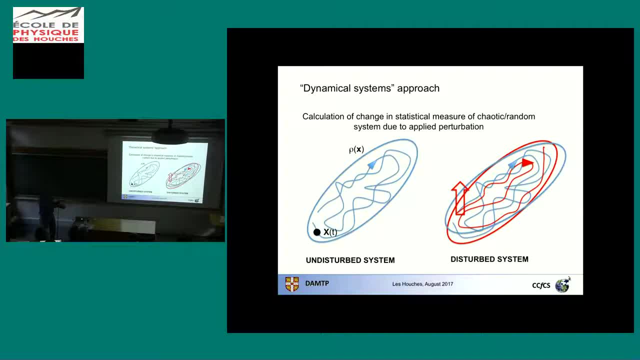 to estimate the differences. You don't look convinced, but anyway, Yeah, It's essentially because you're. If you're in a chaotic system, your linearization would say that you're, You know you're The distance from your. 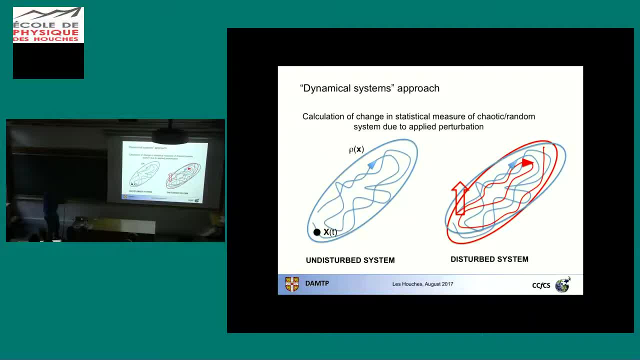 If you're thinking about separation of trajectories, the separation from the original Between the original trajectory and the perturbed trajectory, becomes larger and larger and larger with time. okay, So all the other quantities you're trying to estimate become larger and larger and larger with time. 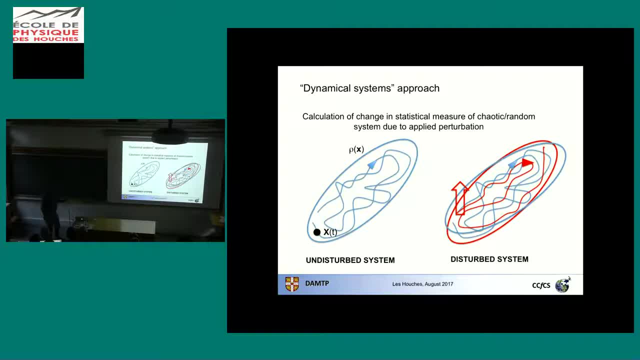 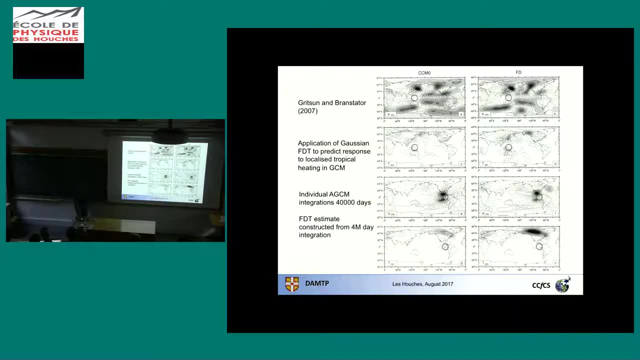 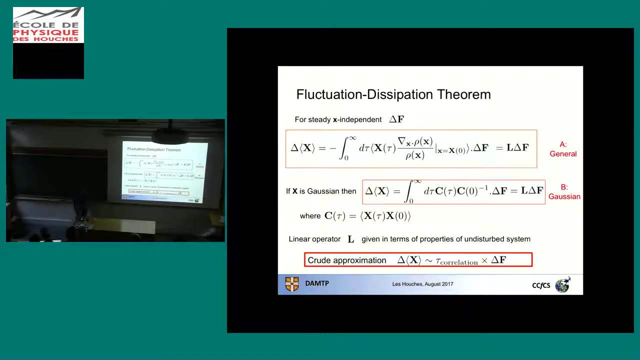 So therefore, you get a sort of Yeah, you get a divergence. Okay, so people, People have tried to apply this approach in a serious way to the atmosphere. Just a question about the terminology: What do you call a fluctuation-dissipation theorem? 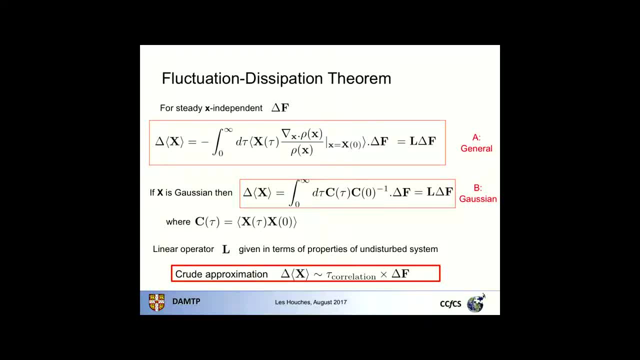 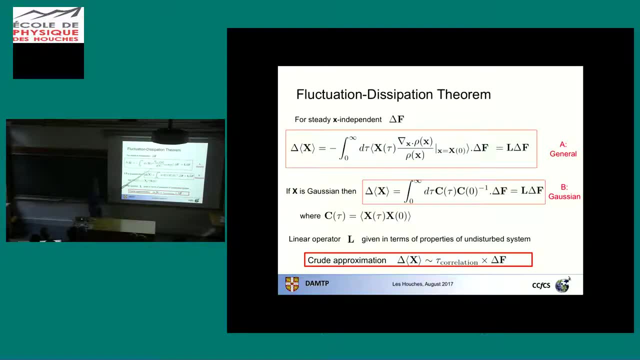 Is both results here. Yeah, I'm thinking of both of these as fluctuation. They are two forms. This is the general form of a fluctuation-dissipation theorem And this is the form which is special to Gaussian systems. Okay, 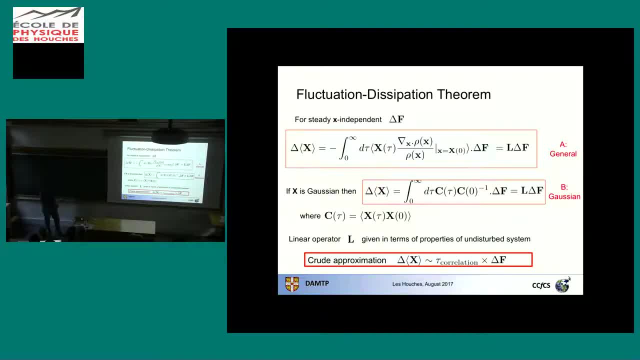 But sometimes this is, This is sometimes called, you know, fluctuation-response theorem And it's sometimes called linear-response theory. I mean it's And the dissipation. as I say, if you go back in the history, it all seems to be to do with the fact that 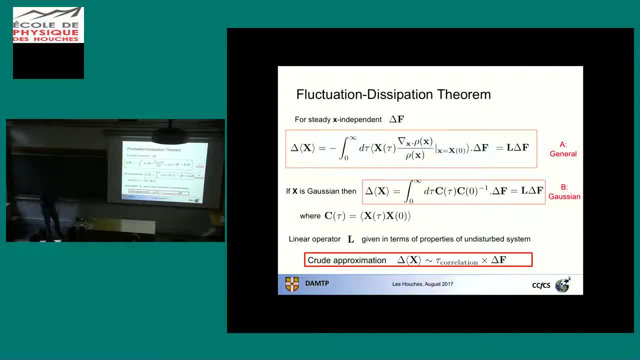 when you consider something like the resistance force on a sphere, it's associated with dissipation of energy, right? So you might say that the link to dissipation is a bit tenuous, particularly in the world of atmospheric dynamics. So we could call it fluctuation-response theorem. 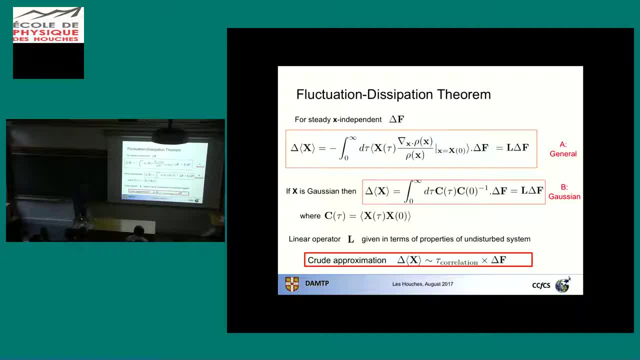 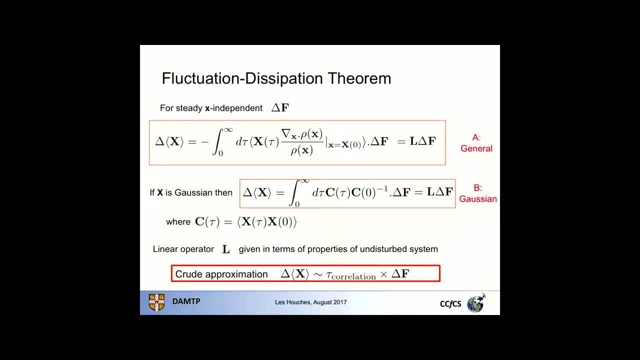 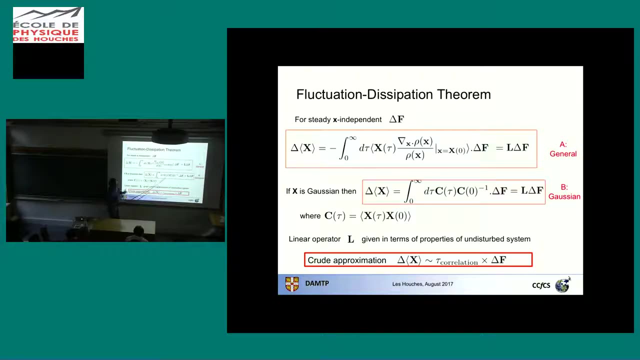 if you like, because that's got the two key words: fluctuation and response. So the key, you know. The question is: can we apply this? And of course, then the issue is sort of practicality, because if you're looking at some kind of 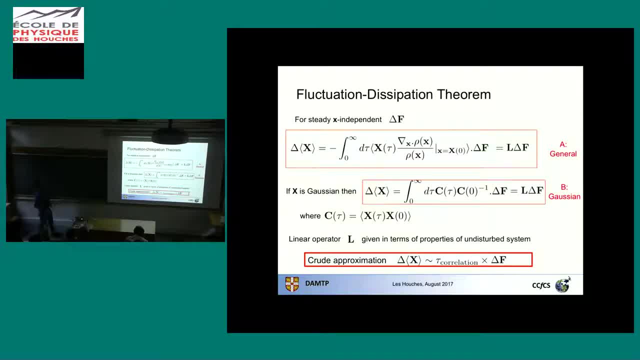 Looking at the atmosphere or looking at a serious atmospheric model, then you have a system with many degrees of freedom. So you've got to. You would be estimating these covariance matrices, So can you provide, you know, good estimates of those from some kind of given? 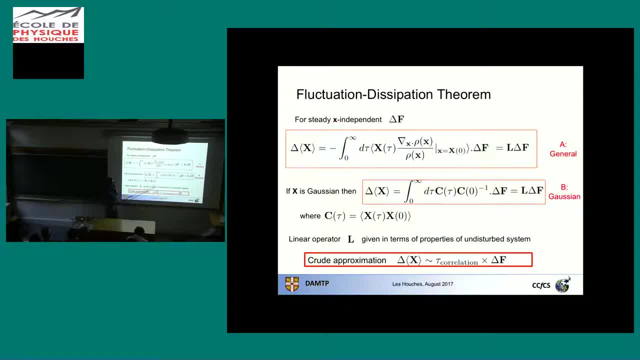 Some kind of given finite record of the system. There's an inverse here. you know which is problematic. You've got to evaluate this time integral, so you've got to truncate the time integral in some way. So the issue comes down to sort of practicality. 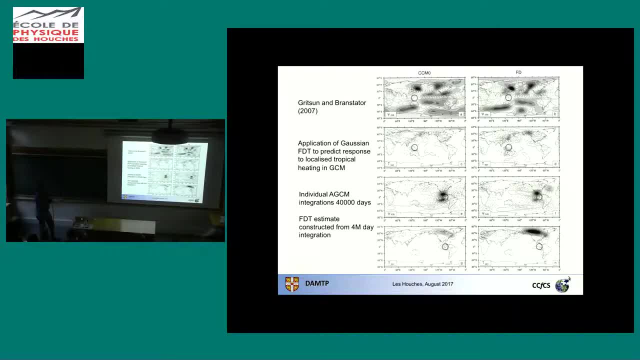 So this is work by Gritsen and Brandstatter. So basically what they did was they ran an atmospheric general circulation model and they sort of reduced the phase space to some extent. okay, to make the dimension of their phase space smaller, to make their calculations more tractable. 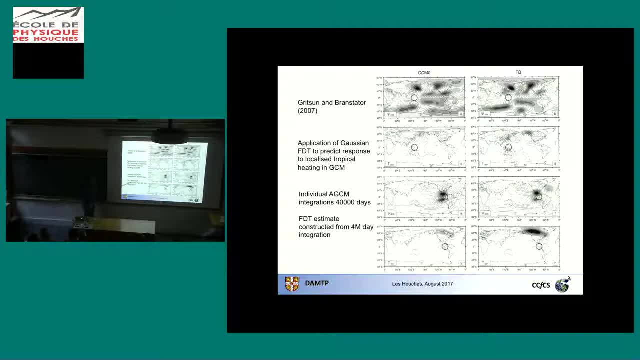 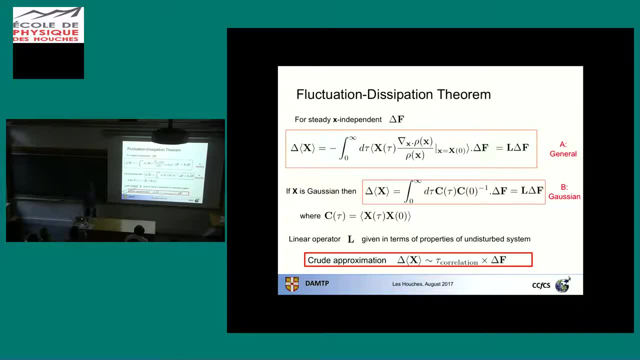 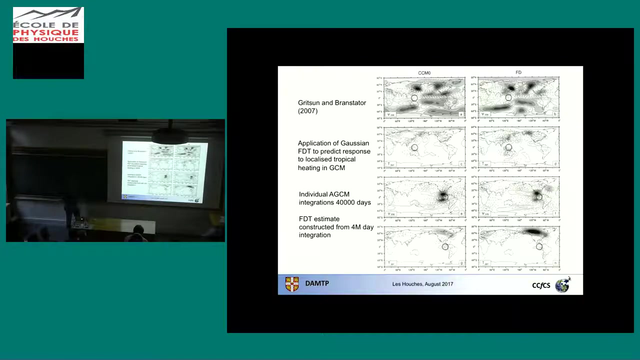 So when they calculated their estimate of this fluctuation dissipation theorem operator, in other words, when they estimated this thing, they used- you know a sort of history of the unperturbed system for four million days, right? So that's quite a long time. 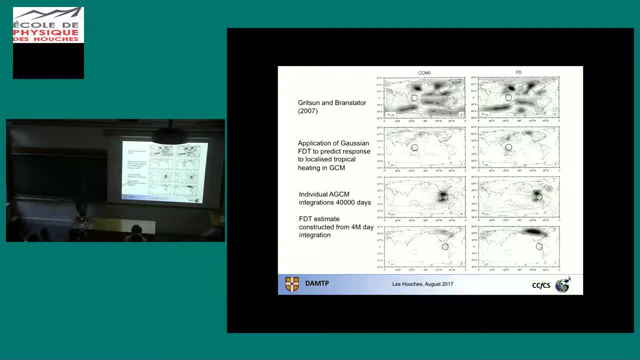 I mean so- And then they compared against. So then they're doing a set of experiments where actually they're applying a tropical heating and they're looking at the time average response to a steady tropical heating and they're comparing the fluctuation dissipation estimate. 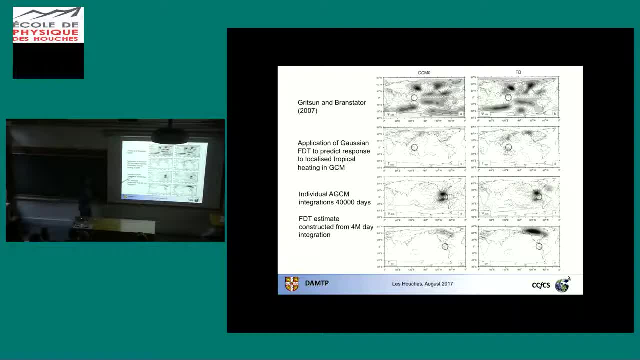 with the. you know the estimate. you know the estimate, which comes from a long integration of a model, with the perturbation in it, as compared to a control simulation, And what you're seeing here is that. So this is. These are different measures of the response. 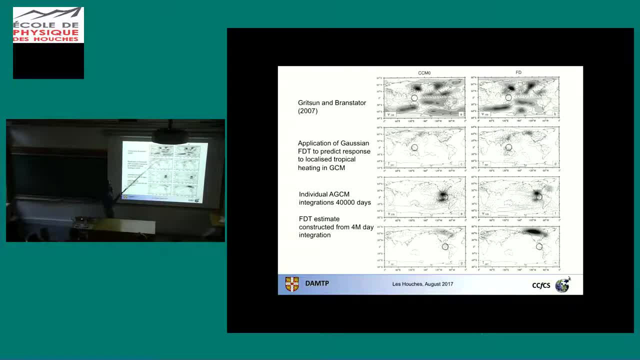 to the tropical heating. These are two different fields: low-level temperature and upper-level stream function. The heating is applied here. Okay, this is the response as measured by the individual, by the AGCM integrations, And then this is the response as estimated. 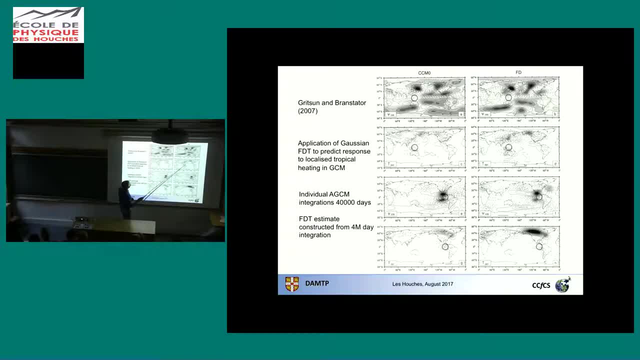 by the fluctuation dissipation theorem in this picture. And then these pictures correspond to a different location for the tropical heating. So you know, one looks at these pictures and there are similarities and differences. Okay, so I mean, if I look at these two pictures, 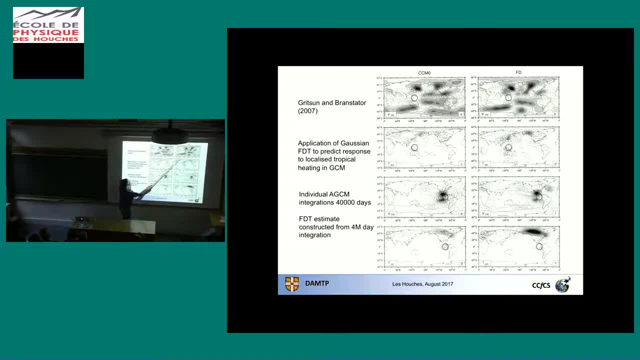 these two features, right then I would say that the fluctuation dissipation theorem is doing a good job. But if I was to look down in this region, well you know, perhaps it's not doing such a good job. One might you know. 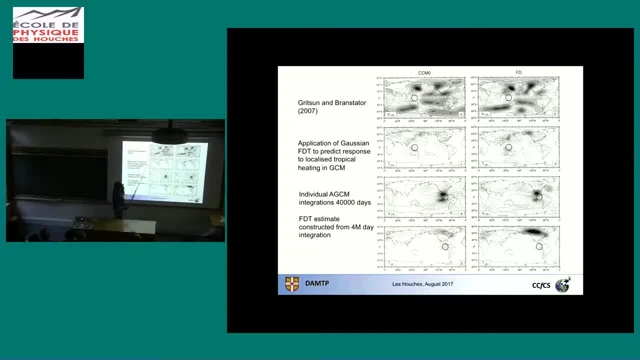 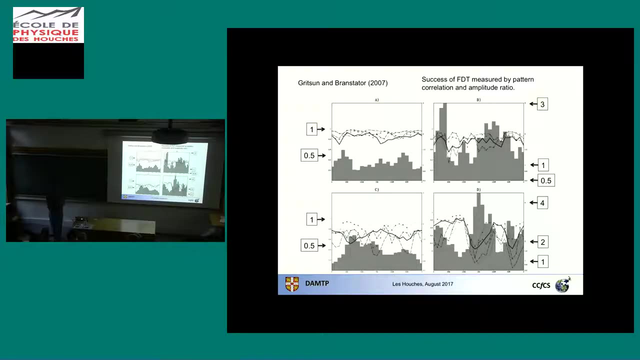 do the same comparison with surface temperature Again. so there are similarities and differences. There are encouraging differences but there are discouraging sim. sorry, encouraging similarities but discouraging differences. It all depends on your point of view. Yeah, So the approach that they used, 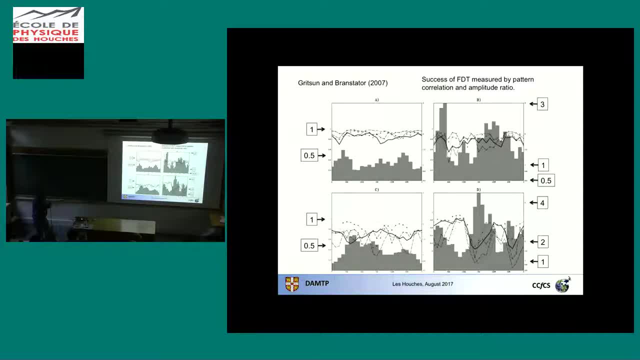 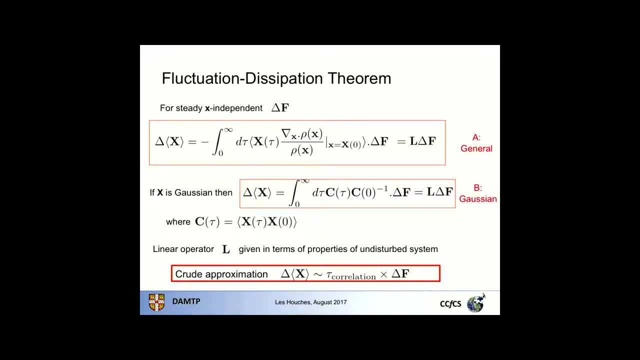 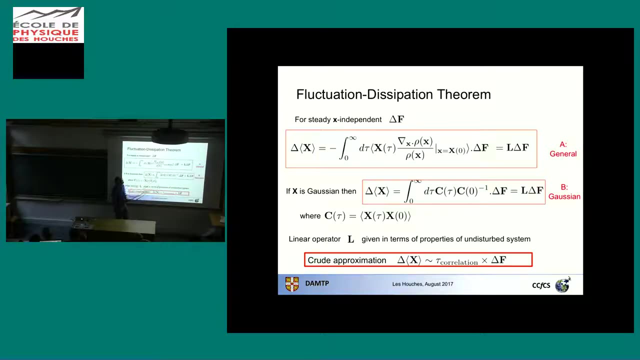 was based on the calculating the probability density or just in initial trajectories, like you mentioned. No, in fact they were assuming the Gaussian form. Okay, So with the Gaussian form, they don't need to. well, they've assumed that rho is Gaussian right. 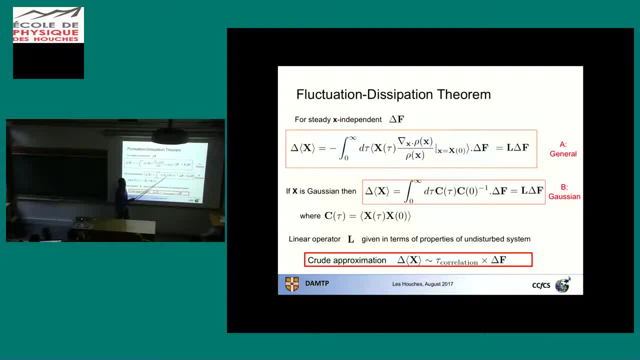 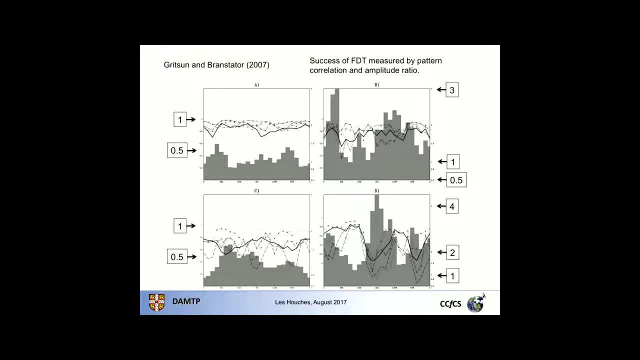 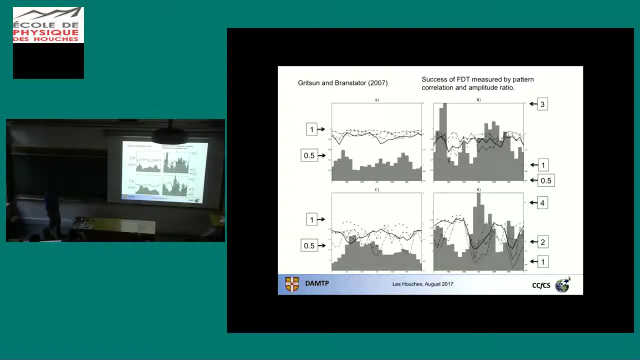 So what they need to do is calculate the covariance matrices. Okay now. so then here are some of their kind of quantitative measures of how well the two things agree. I mean, they have something called a pattern correlation, which I think are the lines here, right? 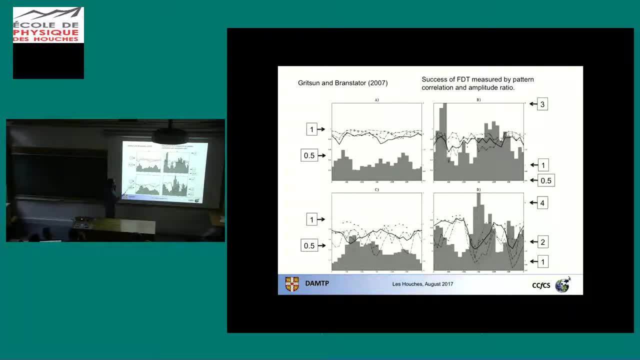 So, and these are for different locations of the tropical heating. So yeah, this is sort of saying if I put my tropical heating at 60 degrees east, then I get a correlation between the pattern in the fluctuation dissipation prediction and the fluctuation pattern. 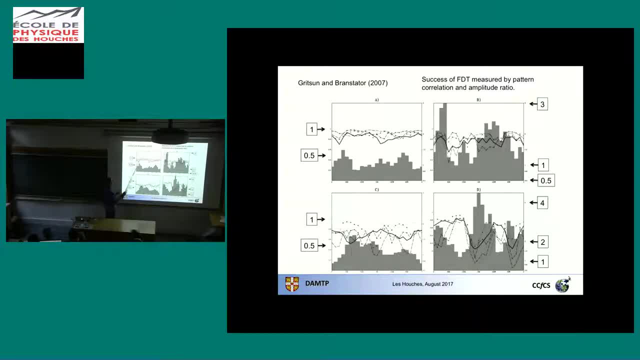 from the explicit simulation of sort of somewhere somewhat around 0.9 or something. On the other hand, if I go to some, put my heating in a different place, I get you know a lower pattern correlation. But the pattern correlation is only part of the story. 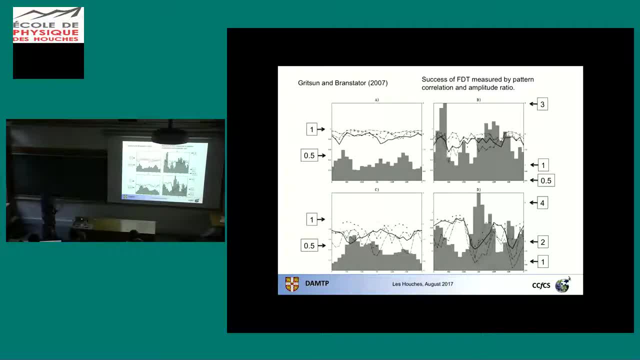 because there's also an amplitude Ratio, okay, And the numbers on this figure are pretty small, but yeah, the amplitude ratio is given by this, these values here as a function of position of the heating. This is the value 1, right. 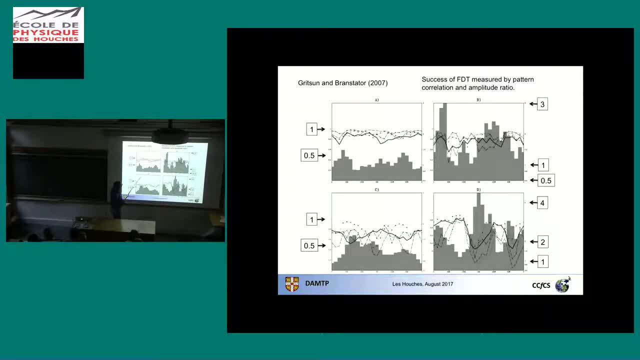 So you can see that for this experiment you're kind of going between 0.7.. 0.8, perhaps, and about 1.5.. There are other examples where you're perhaps looking at different fields or different spatial locations for the heating. 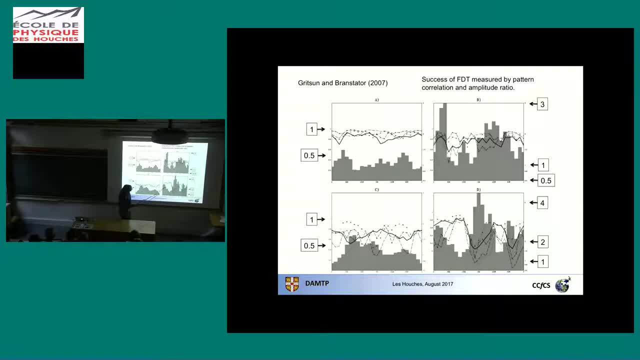 where you're getting much bigger variations in the amplitude ratio. okay, So if you thought, if we focus on the grey bars, there's the value 1. Well, you're getting the right order of magnitude. but then the question about good agreement is: 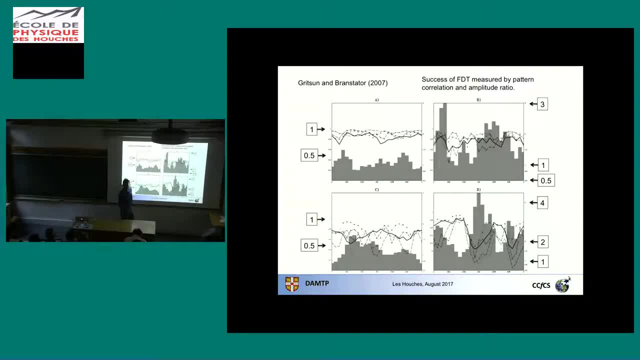 well, do you think that 2 is good agreement? 2 is good agreement with 1, right, It's sort of. It depends what you're trying to do, you know. I mean Ring and Plum have also looked, So actually one thing I should have said. 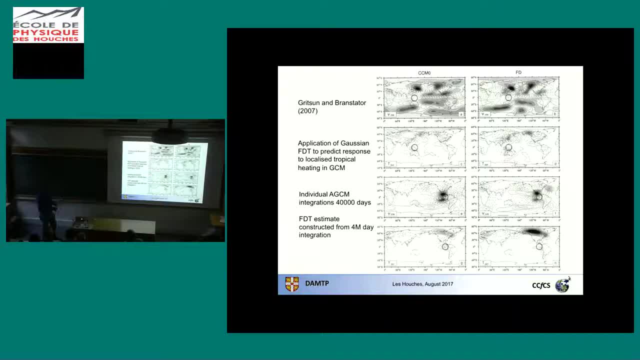 was that this Gritsen and Branstadter work I mean? previously I'd sort of emphasized the problem of the change in the zonally average circulation in response to forcing The Gritsen and Branstadter work is actually looking. 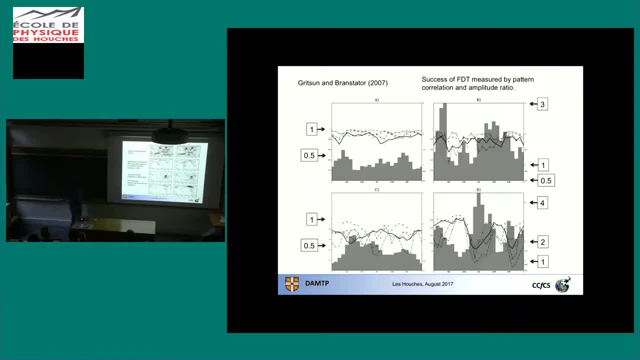 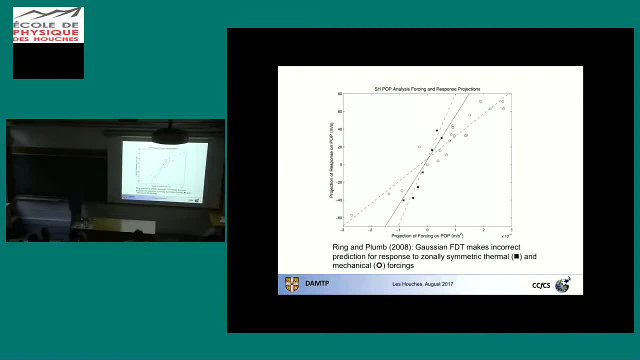 at longitudinal structures as well. Ring and Plum looked at the sort of more zonal average picture Again. well, they find In a world where fluctuation dissipation was working, these three lines would have the same slope right. But they don't. 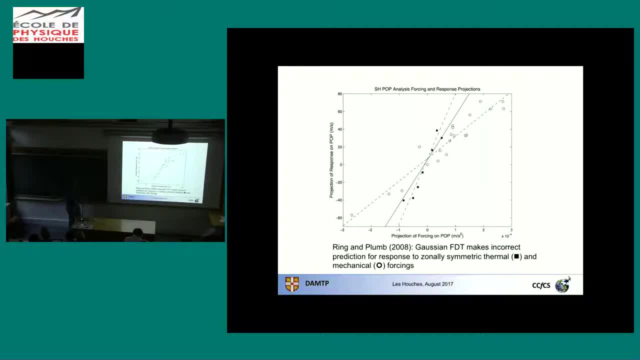 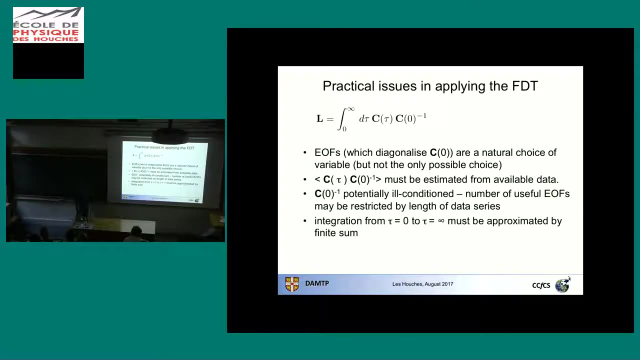 So the point is that when one tries to apply this result, one gets order of magnitude agreement, but significant numerical differences. Yeah Well, I'm going to come on to that. It seems very reasonable that if the forcing is, you know, small enough, 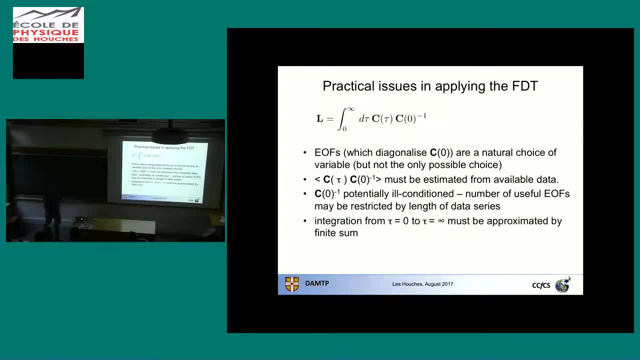 just make it smaller and smaller and smaller. eventually it's linear, and then there should be a linear response to the forcing, And you seem to have proved it right. You've given us something which amounts to a formula which- Yes, that's right. 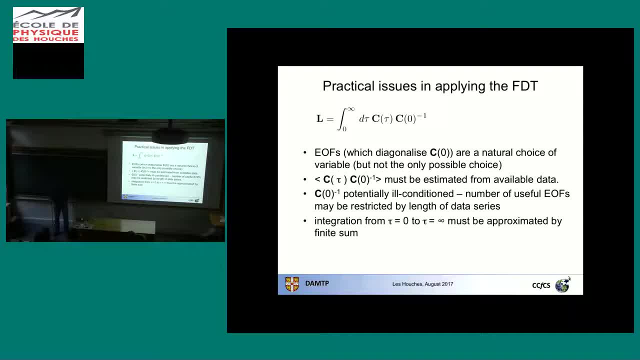 And that's I mean. so I think I'll sort of come on to talk about the various ways in which this might break down. right, I was going to say the only reason it fails is because the forcing isn't small, or because 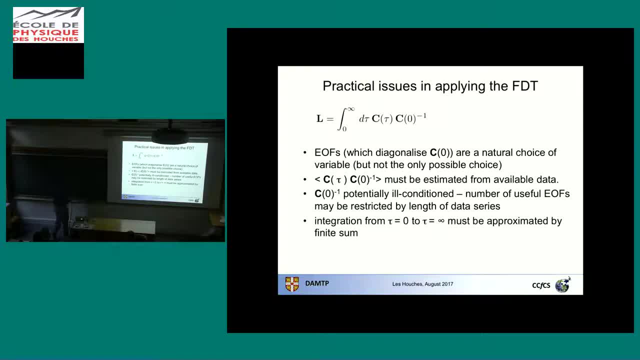 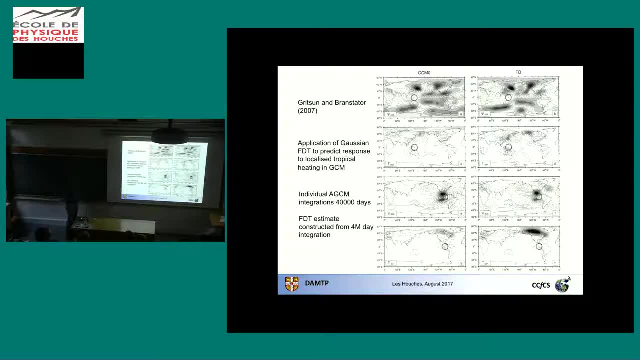 Well, so I mean. So one reason why this might not work is, If we take an experiment like Gritsen and Branstadter's might be, for example, that the forcing they've applied is not small in the sense that 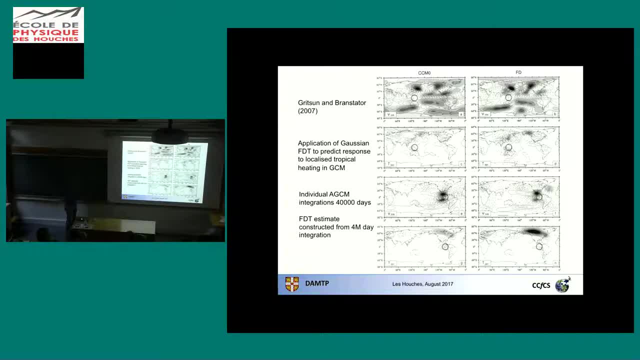 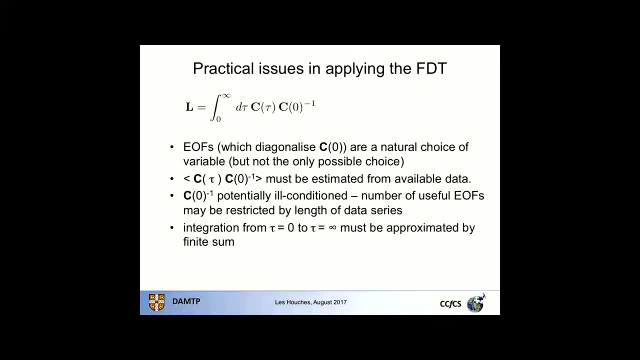 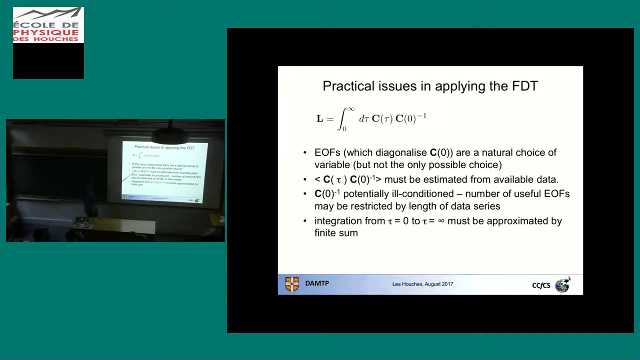 the change in the PDF of the system is small. Yeah, So I mean in terms of practical issues, I mean you've got to evaluate this operator. Yeah, As with many degree of freedom systems, you might try to find a sort of optimal representation of the system. 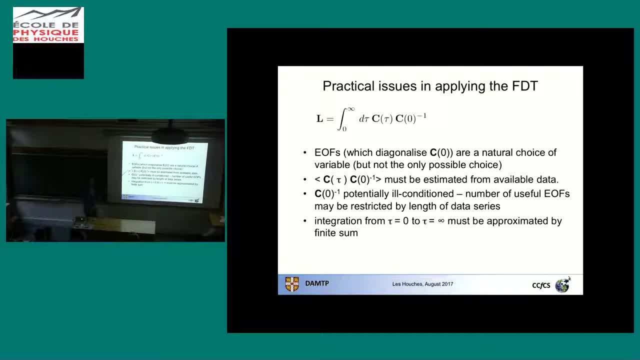 So you might, for example, use EOFs- These are the eigenvectors of the covariance matrices- as a basis. Once you've chosen your basis, you've got to estimate this thing from the available data. So clearly. I mean this is a statistical estimate. 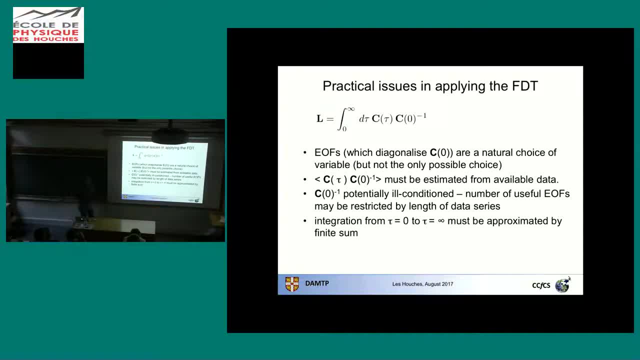 You know you have some finite time series of your system. You're trying to make an estimate of this quantity. This inverse is potentially ill-conditioned. Essentially, this is the covariance matrix. So the parts of this matrix which corresponds to small amplitude fluctuations. 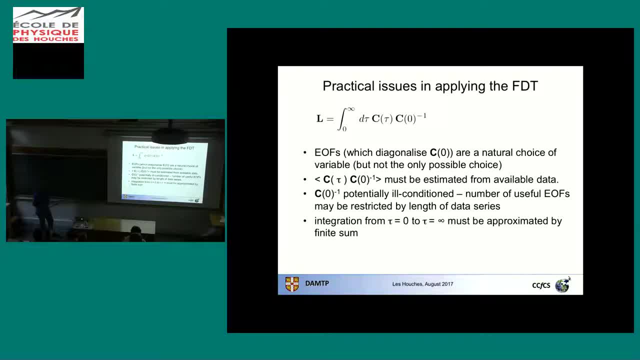 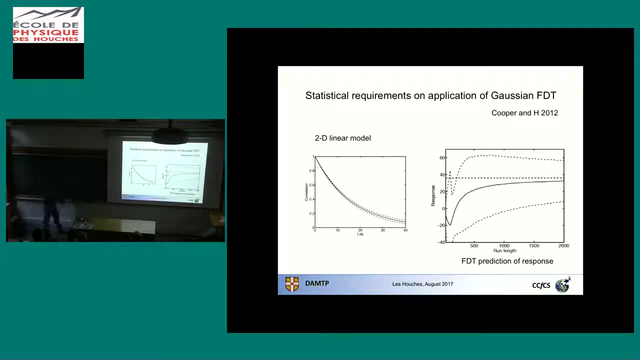 give you a problem when you do the inverse. And then obviously you've also got to think about the effect of this integration. Where do you truncate the integration? So one can sort of illustrate some of these problems. I mean, this is for just a very simple system. 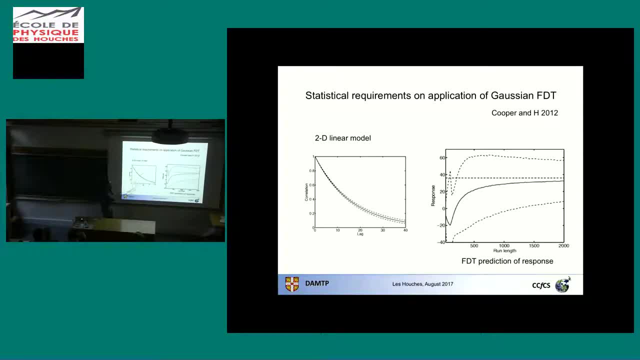 For example on this picture. this is the exact response. This is one variable in the system. This is the exact response. This is how the fluctuation-dissipation estimate converges as you increase the length of the data set, For each length of data set. 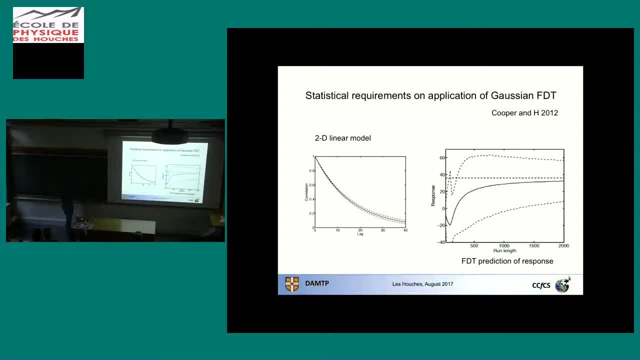 one has to accept that for a given you've got a finite number of realizations and there is an uncertainty about your estimate. So this is the. You've taken a very, very large ensemble. You've taken the mean of that ensemble. 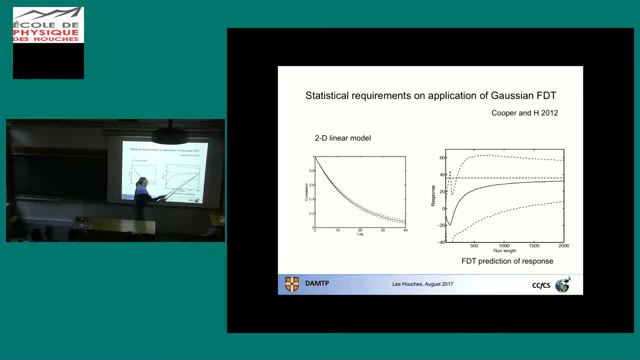 That's kind of converging convincingly towards the exact value. But if you were to take individual sub-ensembles then of course they would vary. So there's a One could talk about. There's a kind of bias. 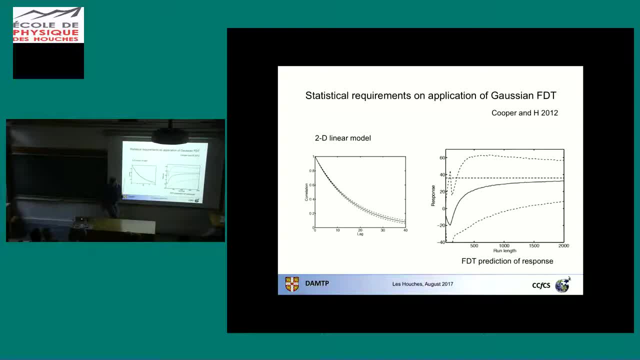 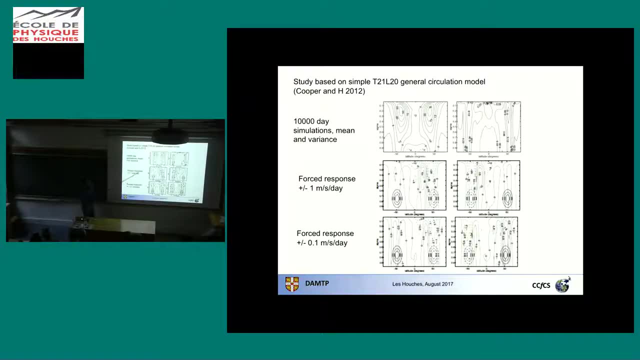 and there's an uncertainty. if you like, Here's an example of the effect of linearity or not. I mean, this is from again, a simple circulation model. You've applied a forcing, So in this case the background circulation is symmetric. 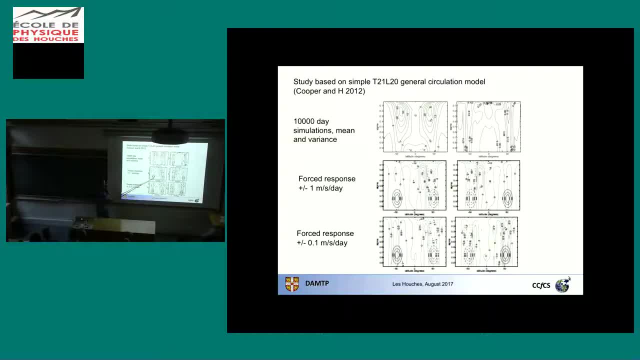 This is the zonal wind. You've applied a positive forcing in one hemisphere and a negative forcing in the other hemisphere, And then here is the opposite. Okay now. so if you were in a linear world, then the kind of response you see here, 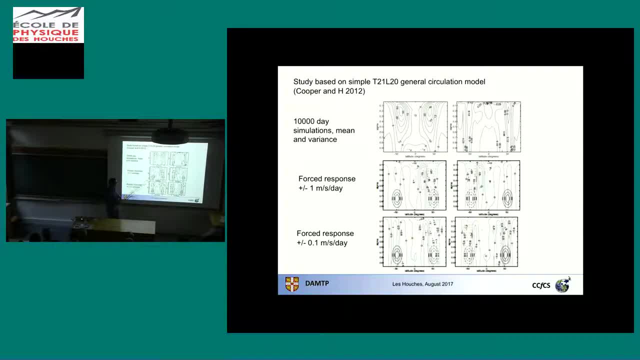 should be the opposite of the response you see here, But clearly for this magnitude of forcing it isn't. On the other hand, if you reduce your forcing then you can get into a more linear regime. Okay, so one has to check those sorts of things. 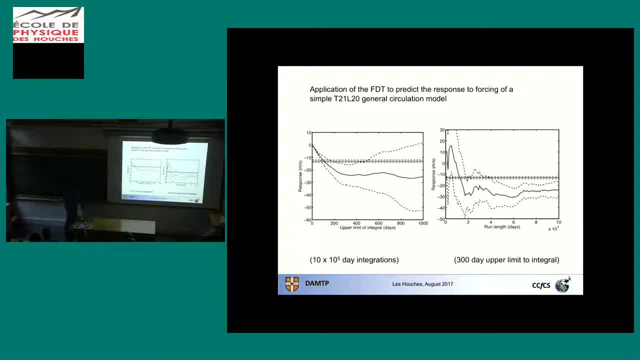 So I mean, the point of this work was really to kind of try to look seriously at some of these kind of statistical issues about the finiteness of datasets, varying the upper limit of the integral and also varying the truncation, varying the number of EOFs you include in the representation. 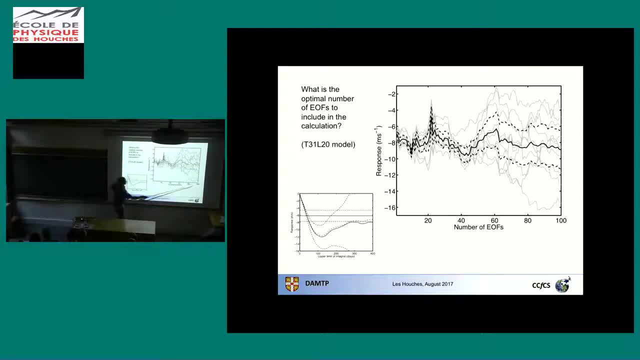 So, for example, this picture shows the predicted response as a function of the number of EOFs you include in your basis. right. And then again, the solid line is a mean over many ensembles and the gray lines are individual ensembles. right. 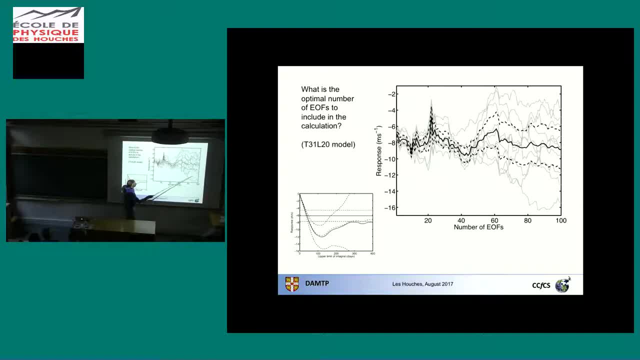 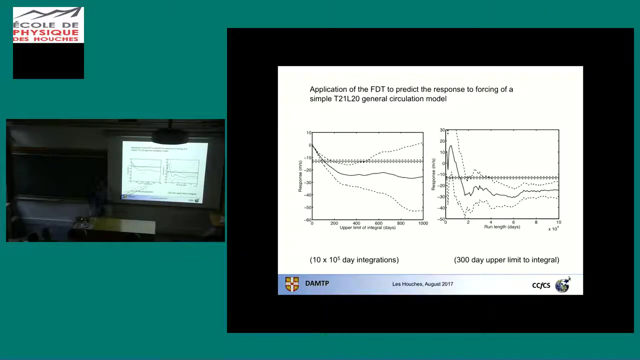 So what you find is you include more EOFs, you get more and more uncertainty in your estimate. So I think the sort of message of this is: there are kind of practical statistical issues here, but there is still evidence that you're not converging to the right answer. 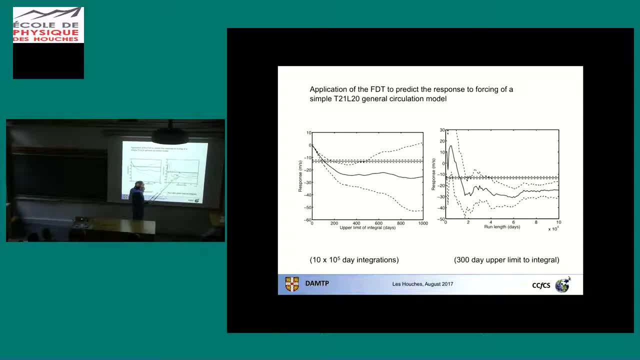 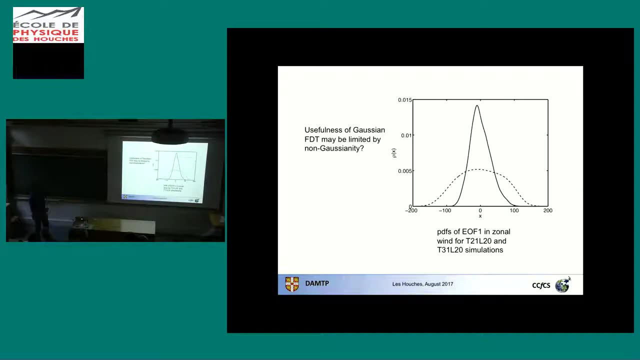 Okay, if we take this case, for example, This was the right answer. You're apparently converging to this one here, Okay. so then, one question is: well, of course, this approach has been based on the assumption that the system is Gaussian. 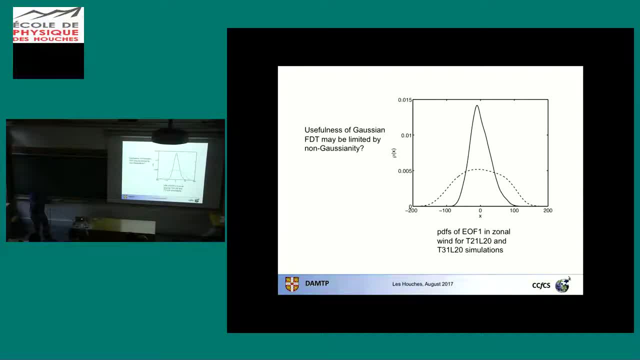 but why should the probability density function of this model tropospheric circulation, or indeed the real tropospheric circulation, be Gaussian? Okay, if you plot the PDF of a particular variable, then for two different simulations. here's one PDF, here's another PDF. 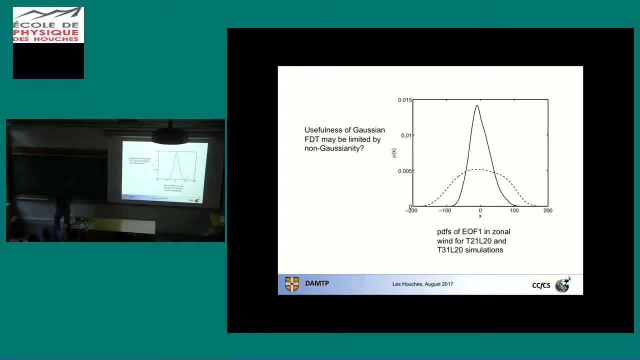 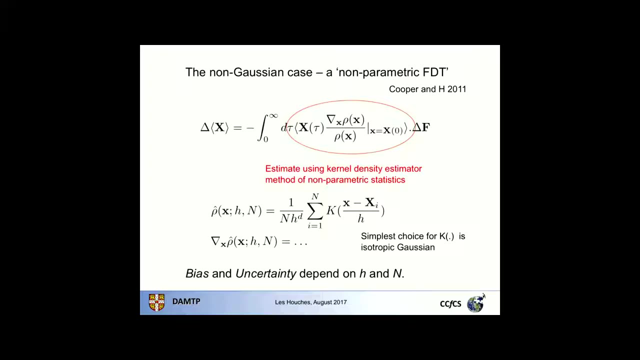 I mean, are those Gaussian or not? I mean they're clearly not exactly Gaussian. And then, of course, if they're not exactly Gaussian, well how much non-Gaussianity do you need to disrupt your answer? So this kind of motivated us to try to use the non-Gaussian FDT. 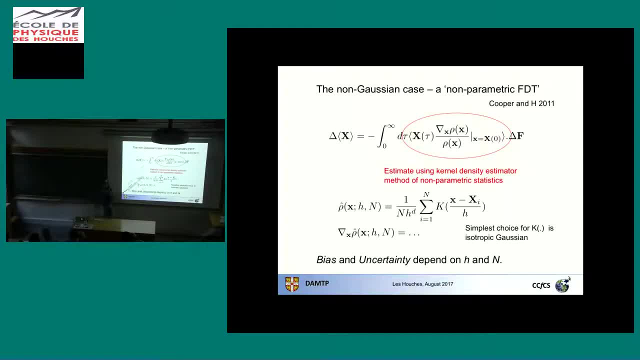 Okay. so if we go back to the non-Gaussian expression, this expression is involved, involves lagged covariances evaluated for the undisturbed system, right, But the difficulty is that this function is an unknown function. right, It's got the probability density function in it, okay. 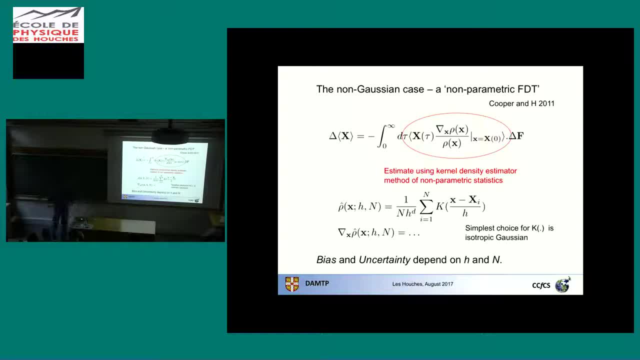 On the other hand, of course, if you've observed the system for a long time, you can estimate the probability density function. There are standard procedures for doing this, So the approach we took was to use a kernel density estimator to estimate the probability density function. 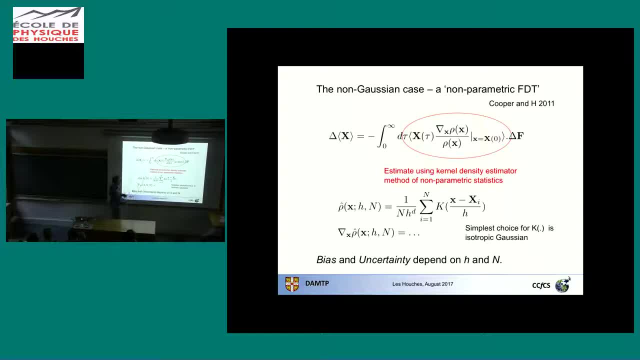 and hence to evaluate, estimate this thing okay. And again one has the usual practical issues associated with kernel density estimators, that typically one is choosing a kernel function, one has to kind of choose a shape factor and then the shape factor. 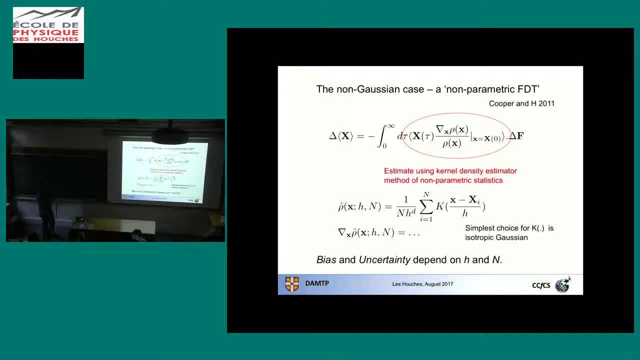 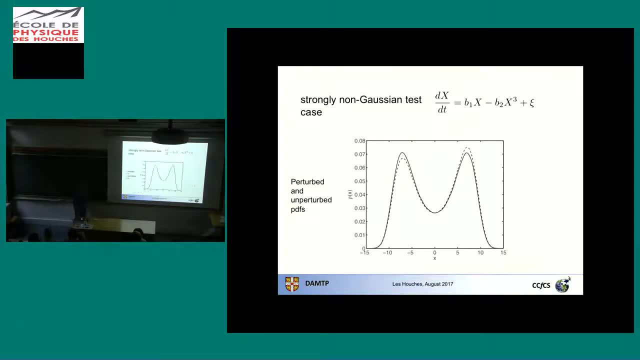 the shape factor H. you might have to adjust as you increase the number of observations in your record. So here's an example where the non-Gaussian approach works. I mean so this is a system, a simple equation driven by noise. The PDF looks like this: 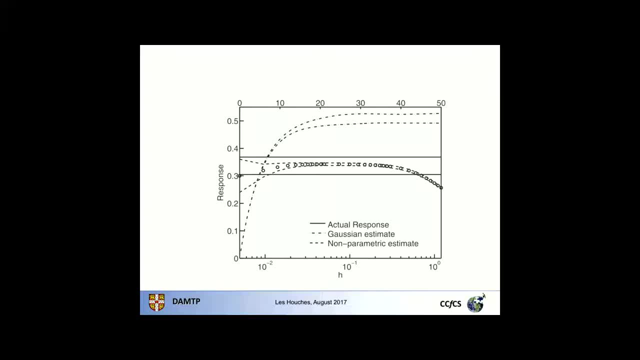 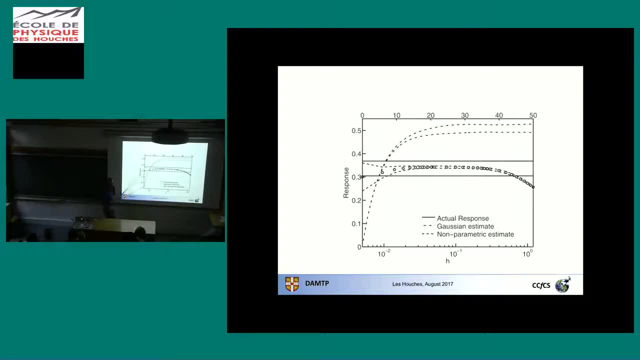 It's clearly not Gaussian, If you, if you do again look at this, is a single variable representing the response. so the Gaussian estimate is up here, okay, And the actual response is here and the non-Gaussian estimate matches the response, okay. 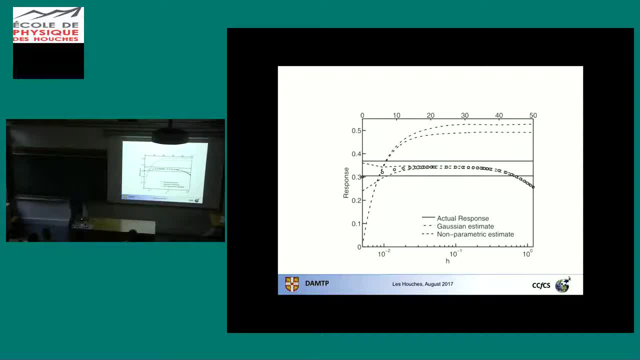 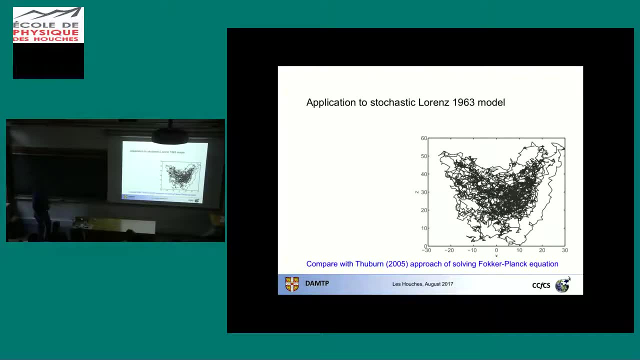 So you've sort of done the job in this very simple case. Can you go to a more complicated case? Well, I mean, we tried this with a stochastic Lorenz model. So again, this is another system which one feels, provided the stochasticity is not too strong. 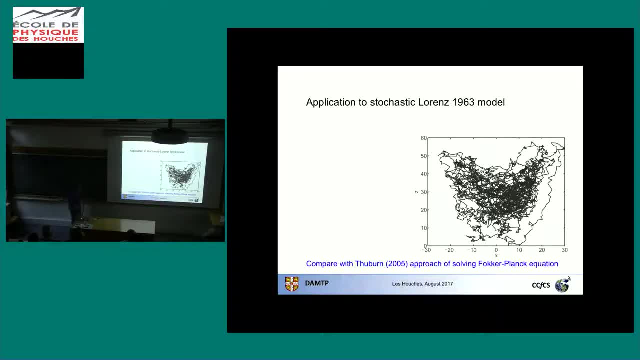 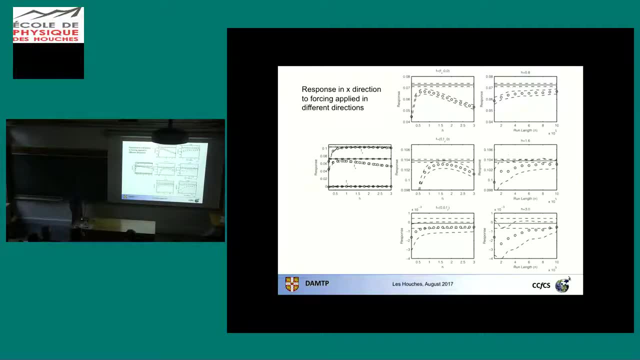 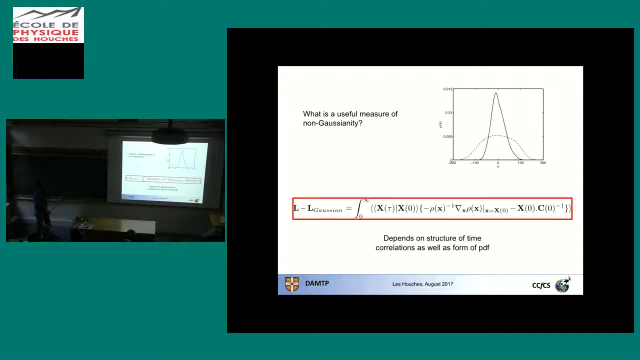 that it should be strongly non-Gaussian and one can get reasonable success with applying this non-Gaussian fluctuation dissipation with this system. But this does actually leave the question of you know what's a useful measure of non-Gaussianity. 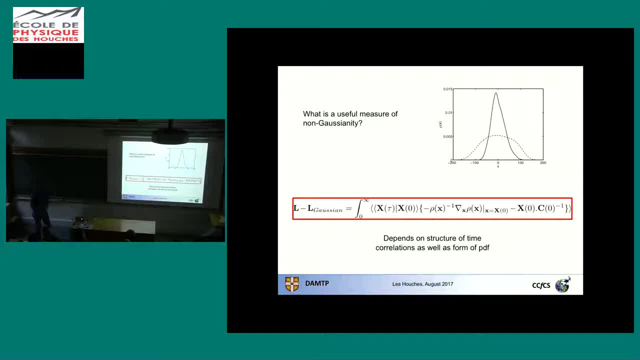 because you know we can. what one would really like is a quantitative measure of non-Gaussianity which you can use as a basis for deciding whether or not the Gaussian approach is going to work or not, And actually that's kind of rather subtle. 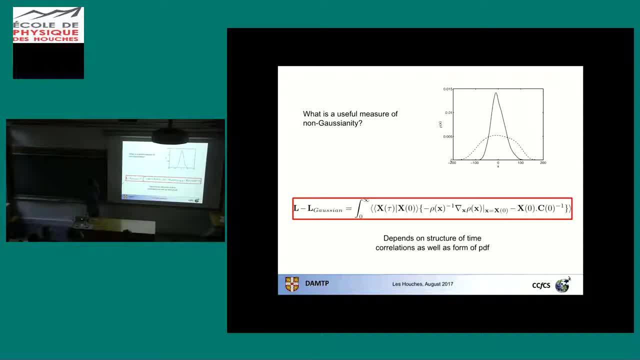 because the difference between the complete operator and the Gaussian operator is expressed by this expression here, and this thing here is certainly non-zero if the system is non-Gaussian. but one also has to take into account sort of time correlations, So if the time correlations have a particularly simple structure, 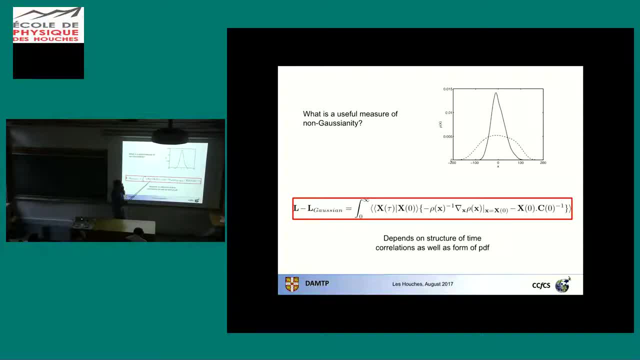 where the expected value of x given time tor is a linear function of the value of x at time zero, then actually this thing disappears, right. So the appropriate measure of non-Gaussianity here can't just be determined by looking at the probability density function. 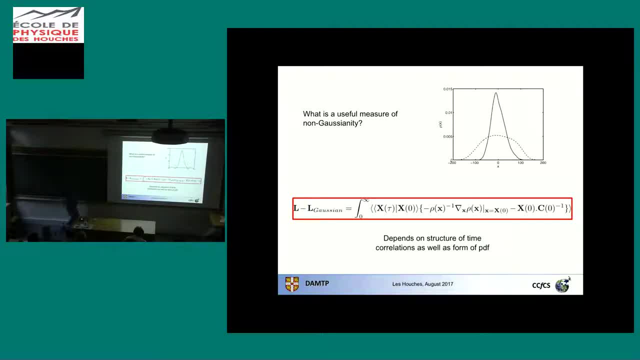 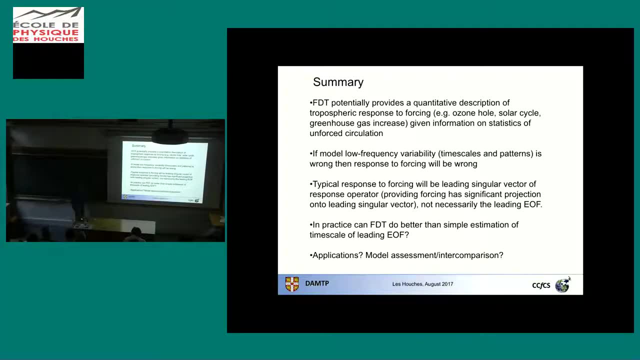 One also has to look at some measure of the time correlations. So it must be almost time to finish. So these are the kind of takeaway messages. So potentially the fluctuation dissipation theorem gives you the response of, say, the troposphere to a forcing right. 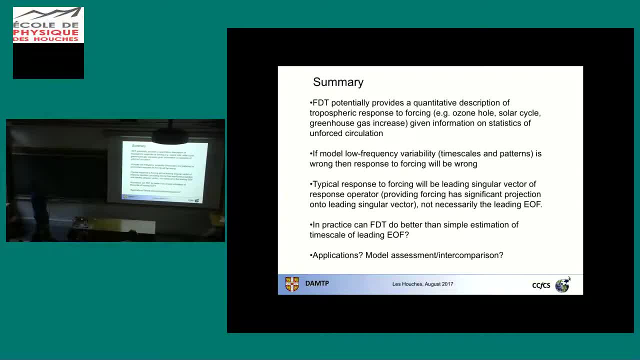 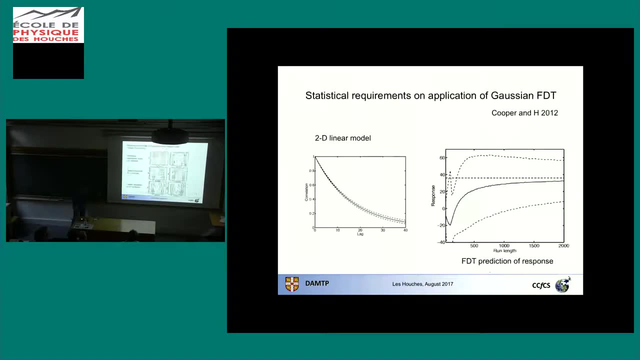 If you've got enough information on statistics of the unforced circulation, then you can predict the response to a forcing. Actually, one of the kind of key insights and perhaps you might say at the moment the concrete insight, is that the response to forcing 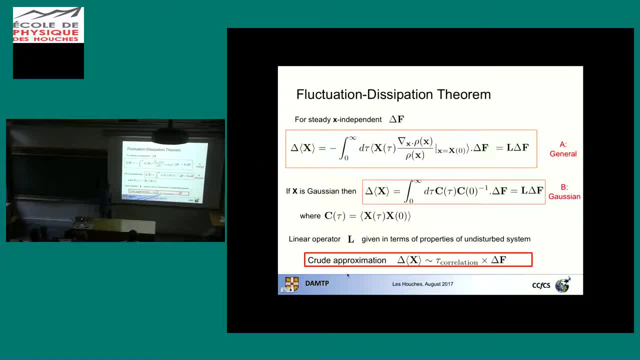 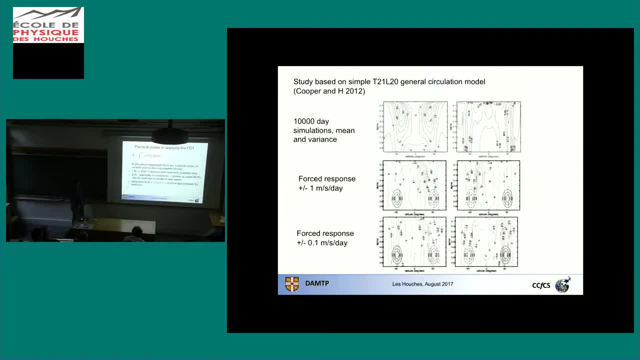 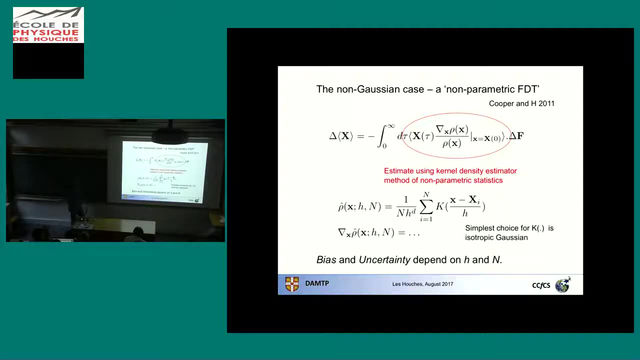 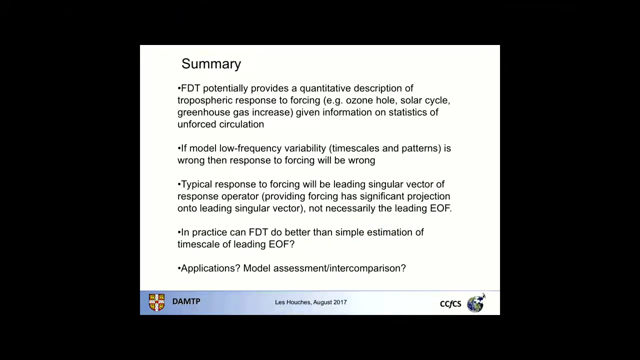 is determined by the correlation time for the unforced variability. So what that tells you is that if your model has the wrong timescale of its internal variability, it will give you the wrong response to forcing, And that's an important insight. I mean other messages, well, 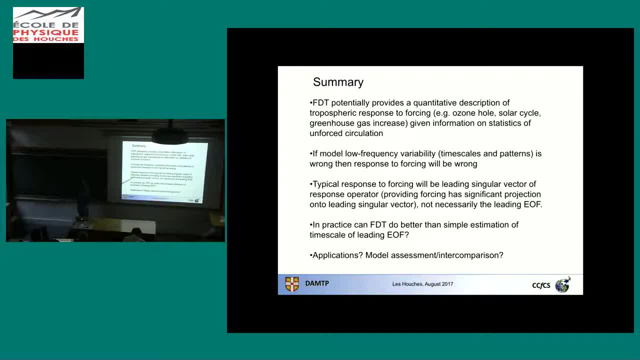 one can construct this response operator. So typically this response operator will have a kind of leading singular vector and for most forcings the response will be, you will see, the leading singular vector. But that leading singular vector is not necessarily the leading EOF. 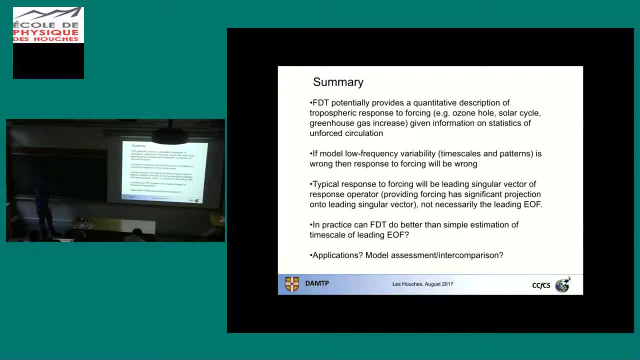 It's not the sort of shape of the largest variance in the system And that's a sort of confusion that people have. As I've said, I mean, perhaps the most important insight that one has at the moment is that what's important is the timescale of variability. 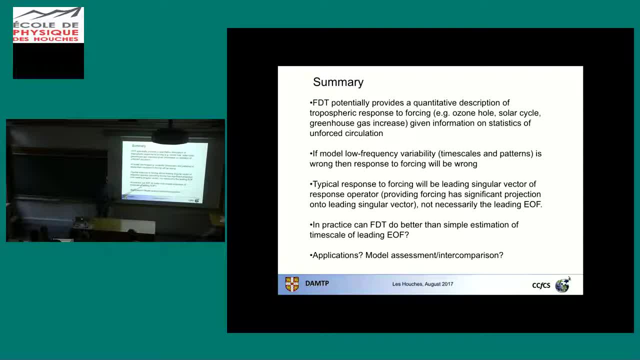 I mean. I think the real question is, can the fluctuation dissipation theorem do better than that? I mean, what you would like would be not only the relation to the timescale of the variability, but at least some kind of skill in relating the spatial structure of the forcing. 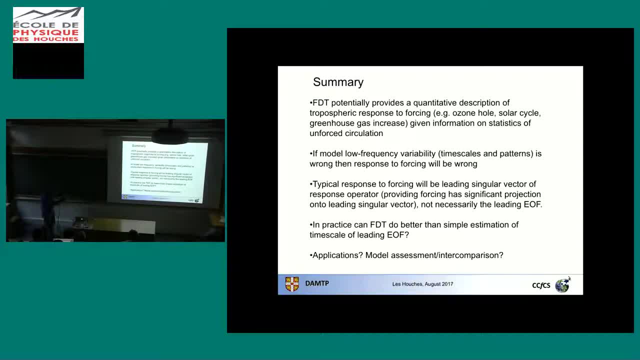 to the amplitude of the response right, And it's not really clear that anyone has successfully used the FTT to do that. I guess that Gritsen and Brandsatter have made some progress. There are various other things I could talk about. 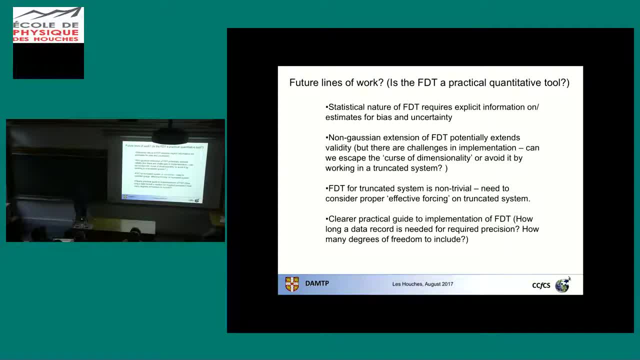 but I don't know. There are various future lines of work. I mean, one thing I feel that's been neglected is that in applying the FTT, you have to realize that this is fundamentally a problem in statistics, so that when you provide an answer using the FTT, 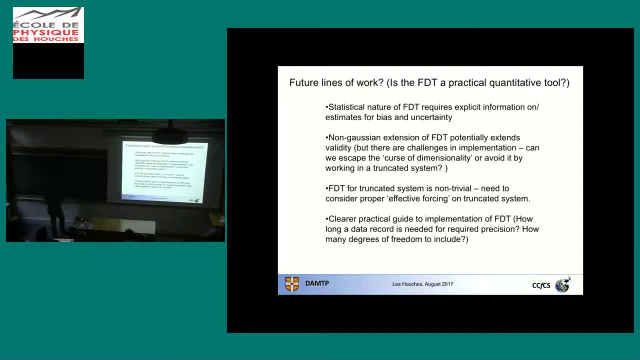 you should be also estimating the bias and the uncertainty in the answer. That information should be kind of provided. I've shown that in principle there's a non-Gaussan extension, but there are big challenges in implementation. I mean, we implemented it. 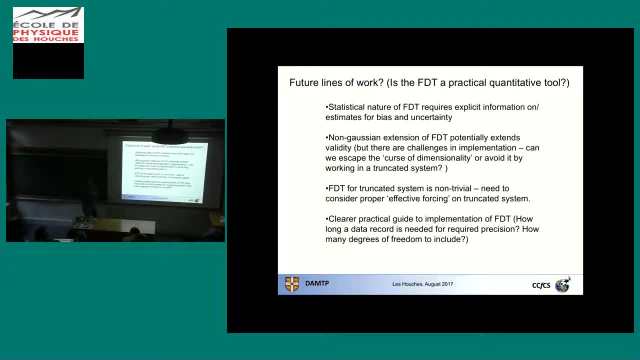 for a three-degree-of-freedom system. There's something called the curse of dimensionality, which basically says that estimating the probability density function gets much, much, much harder as you go to larger and larger dimensions. okay, You need to think quite carefully about truncation actually. 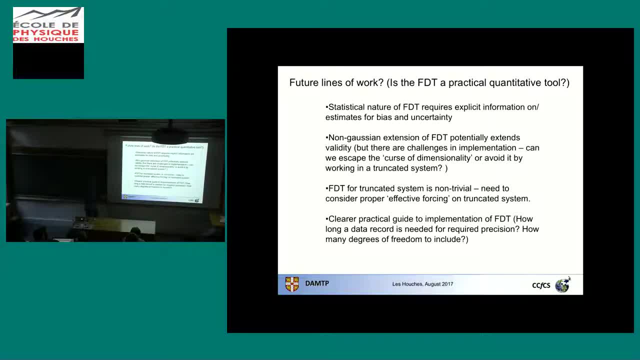 You can't simply truncate the system. It's not obvious you get the right answer simply by truncating the system and looking at that. So I sort of feel in some ways that there needs to be a clearer practical guide to implementation, a sort of user guide. 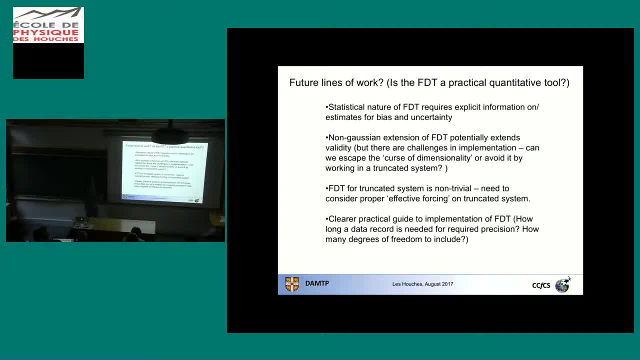 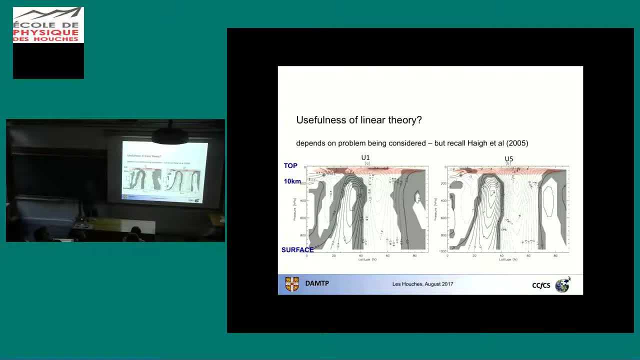 You know, the big question is: how long a data record do you need? How many degrees of freedom do you include? How do you do it? But I mean there are. it does seem to be worth thinking more about this problem because the idea of a linear operator. 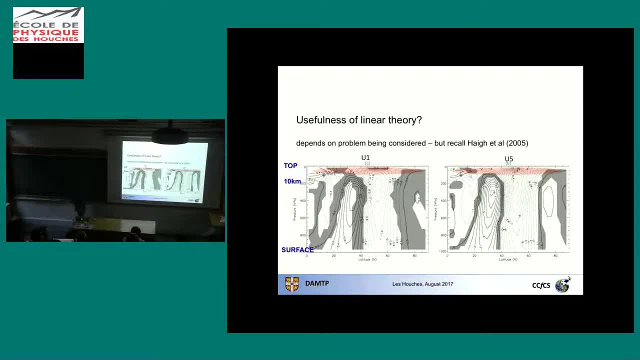 seems to be remarkably useful. I mean, I showed this example earlier of the Hegetal experiments. you know where you were getting the same. this looks like a linear problem. You've perturbed the stratosphere by one here and by five here. 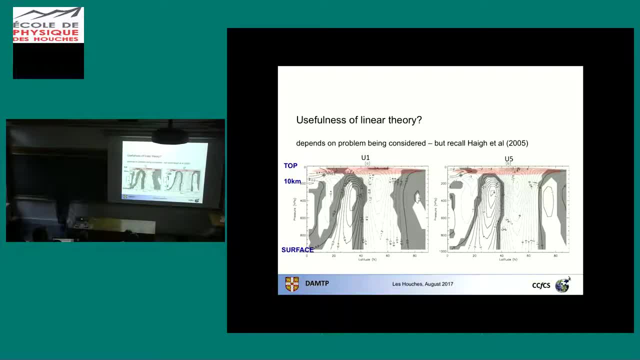 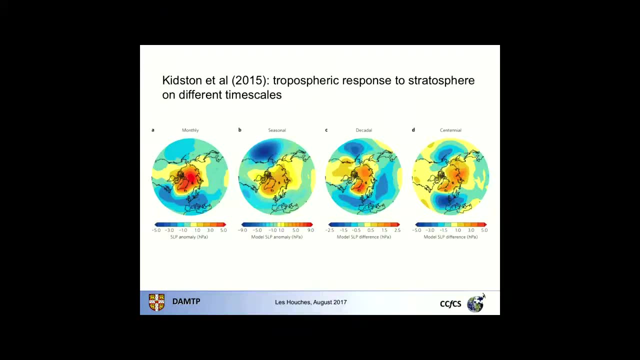 You're getting a spatial structure of the response which is similar and about five times as large, right. So another interesting sort of manifestation of this is that, if you look at, this is from a review paper on the effect of the stratosphere. 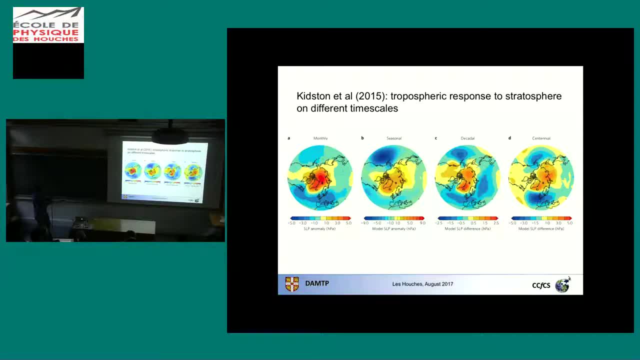 on the troposphere in the extratropics if you kind of look at different measures of the effect of the stratosphere on the troposphere on different time scales. so this is called a monthly response. This actually is a tropospheric signal. 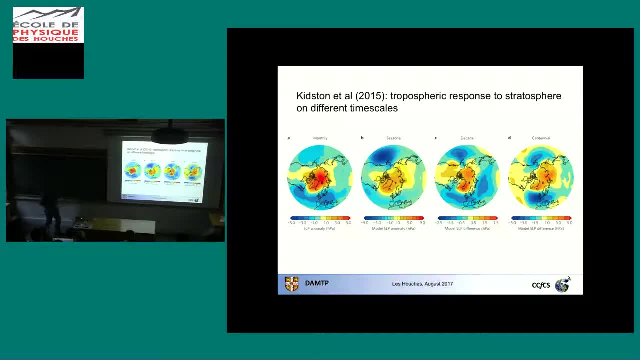 following a sudden warming. This is a seasonal response. I'll now have to remember how that's different to the sudden warming one That's probably with some kind of radiative change. This is a decadal response. This is this kind of solar cycle type response. 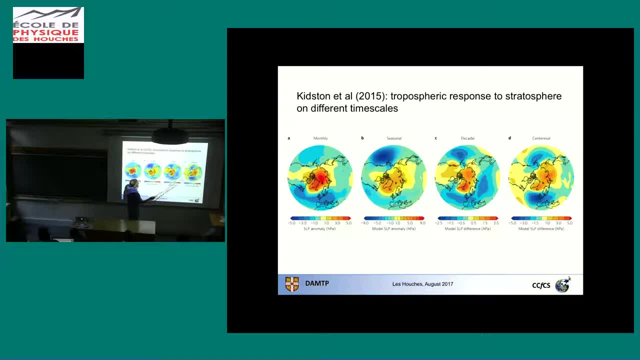 This is a centennial response, So this would be a kind of climate change response. Yeah, there is quite a lot of similarity in the patterns here. okay, So you know you can the idea that some kind of linear theory. 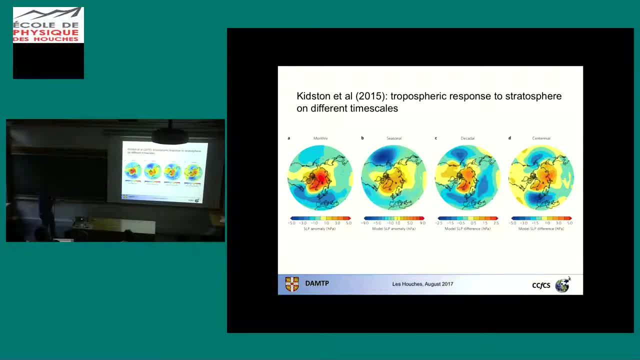 is useful here, and what you're seeing is the pattern of a preferred response is potentially useful, And the pattern of the preferred response is essentially determined by the tropospheric circulation. So that you know, for example, the pattern has a in climate terms one would say that 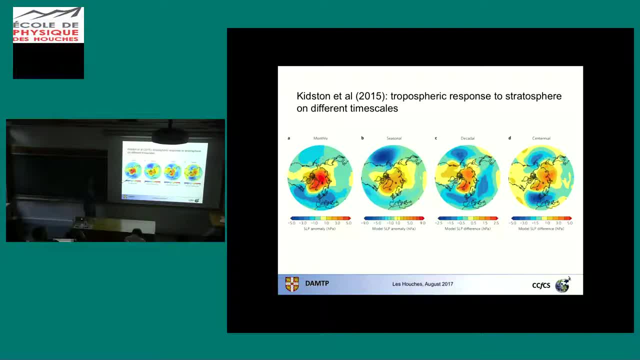 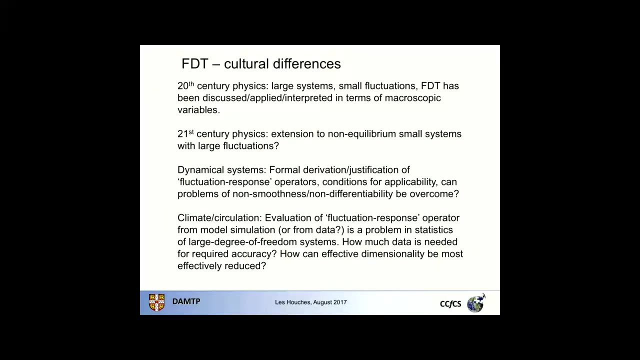 the pattern has a large component which is associated with the Atlantic Oscillation. That's determined by the tropospheric circulation. It's not determined by the details of where the forcing is applied in the stratosphere. And then I could sort of finish on cultural differences. 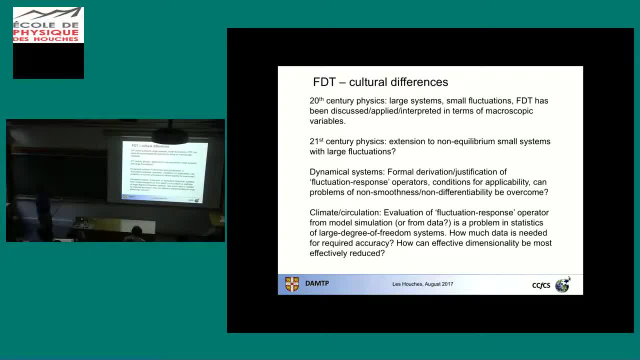 I mean it seems. I mean, of course, the fluctuation dissipation theorem means different things to different people. I mean, so the it's. I think in classical physics you've typically been looking at very, very large systems. 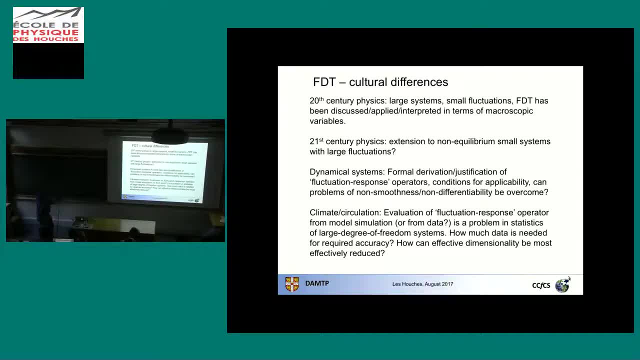 And fluctuation dissipation theorem is essentially giving you a deterministic. you know a number right which is describing this very, very large system. You can use thermodynamics to give you explicit predictions. In the world of dynamical systems, people are more interested in. 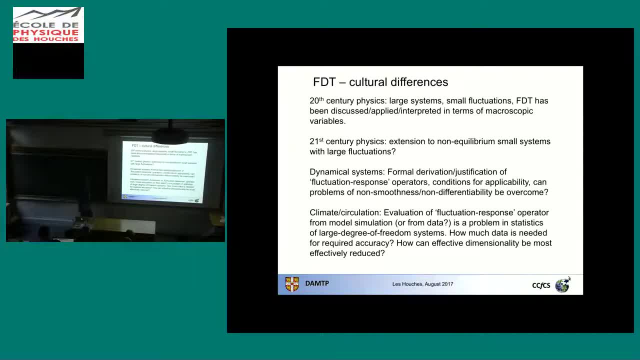 sort of formal justification of these theorems. You know, the question would be: does your probability density function really vary smoothly as you apply small perturbations? Okay, actually, you know, if you look at very, very simple dynamical systems, 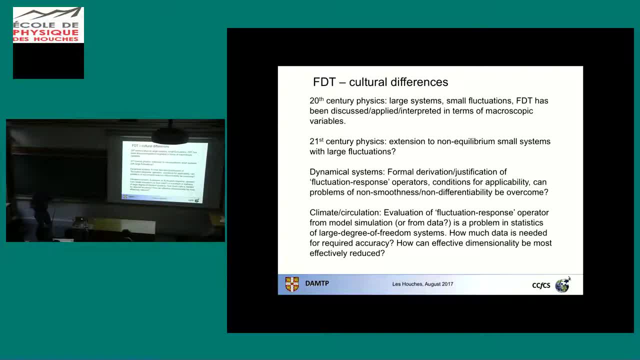 you know tent maps and things like this, then of course you can generate examples where the PDF does not vary smoothly. But then you might one mile to the question. well, actually, is that really relevant to the real atmosphere or ocean? 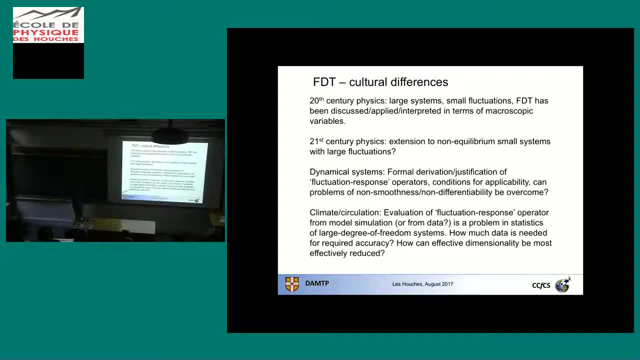 I mean in the world of climate or circulation- then clearly you can use fluctuation dissipation to evaluate your operator from a model, simulation or from data. It's a sort of problem in statistics, So you need to know how much data is needed. 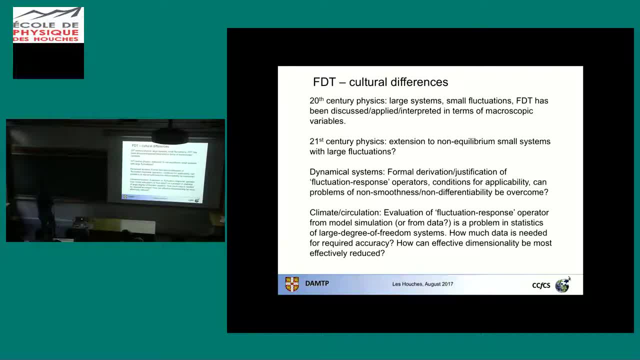 and how can you reduce dimensionality? But what you're not doing here is you're not- you know, you're not- providing a sort of external theoretical prediction of the response operator. You're taking a system and you're using the system itself. 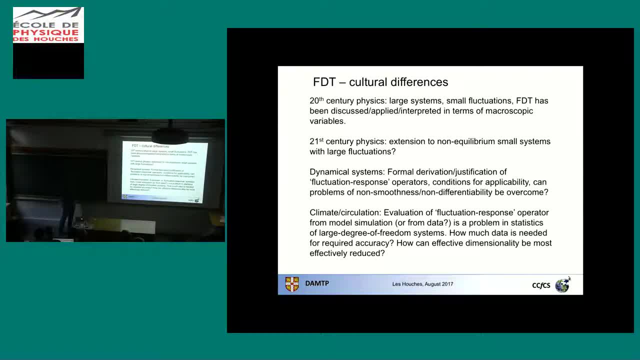 to provide the response operator. okay, Now you might say, well, is that worth doing? Well, because it focuses on the relation between variability and response. I think it is very valuable. You know it says to you if your system has the wrong variability. 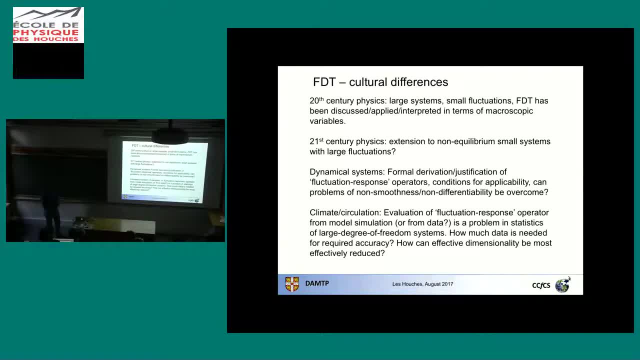 then you will get the wrong response. Then, of course, the dynamics comes. It's like if you have a model which has the wrong variability, the question is: why does it have the wrong variability and how do I improve it right? 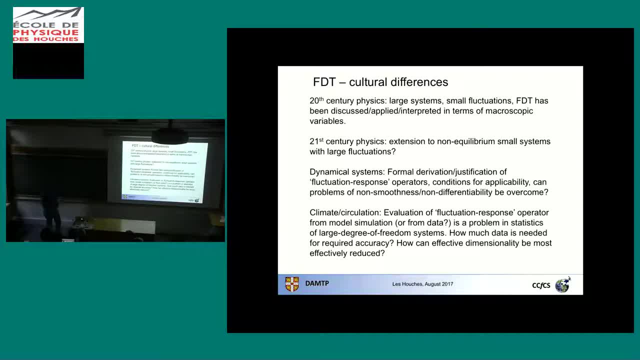 And the fluctuation dissipation theorem doesn't give you any insight into that. But the simply making the link between variability and response is potentially useful. I'll stop So for the FTT. so if the FTT can work, it seems forcing needs to be small. 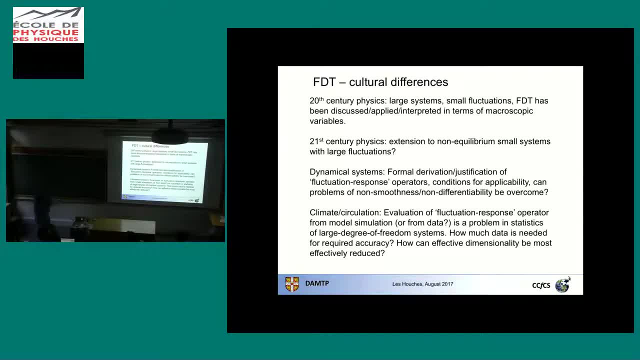 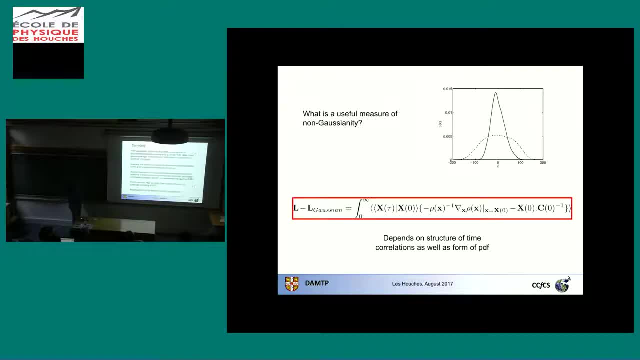 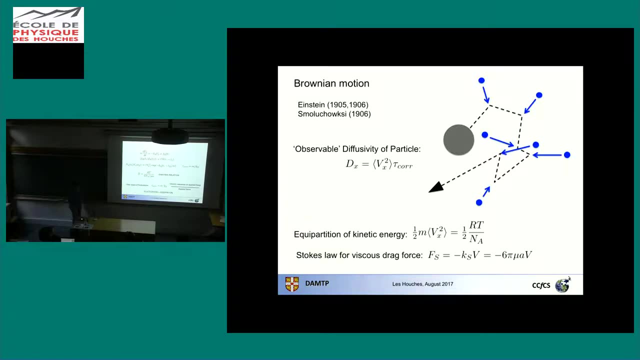 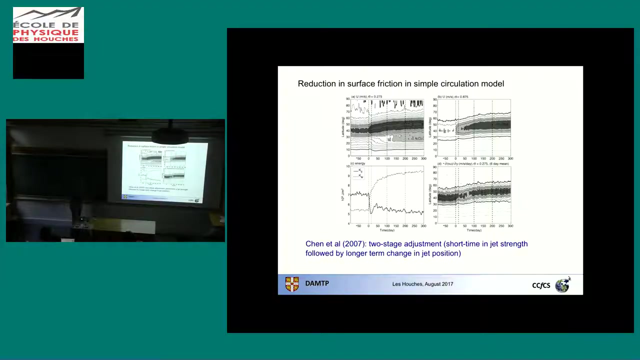 Do we have a good understanding about what kind of forcing can be considered small for the climate system? Well, I think that one, yeah one does by doing experiments. So you know, perhaps changing greenhouse gases over 100, next 100 years? 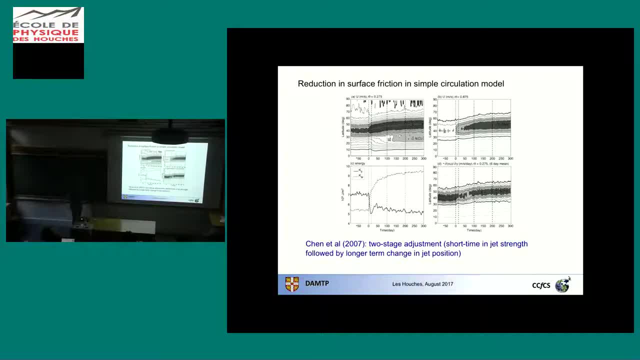 is a small perturbation. yeah, is a small perturbation in this sense, okay. On the other hand, perhaps if you quadruple or carbon dioxide, then that's not okay. But I mean, but those are sorts of that sort of information. 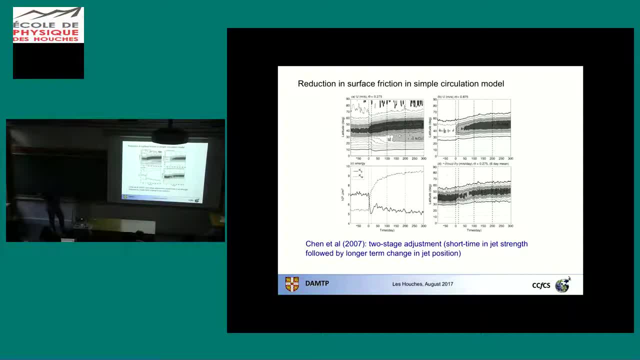 you can get from experiments right So, but it's something. I mean, I would think of it as something you need to bear in mind when you were doing experiments. You showed these plots where we had the true answer, the true response of the system. 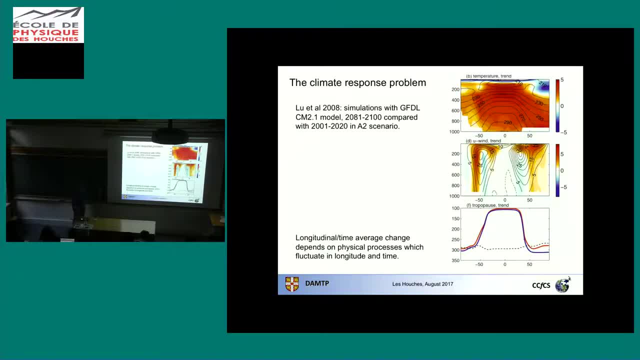 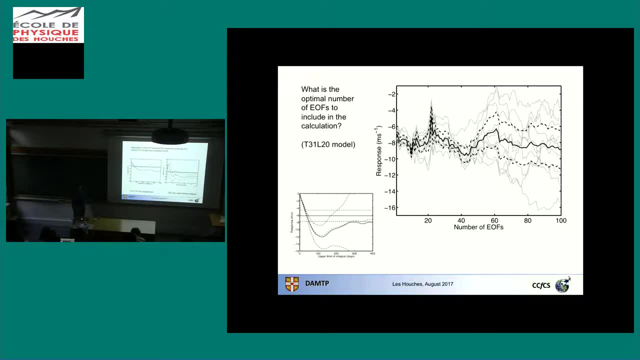 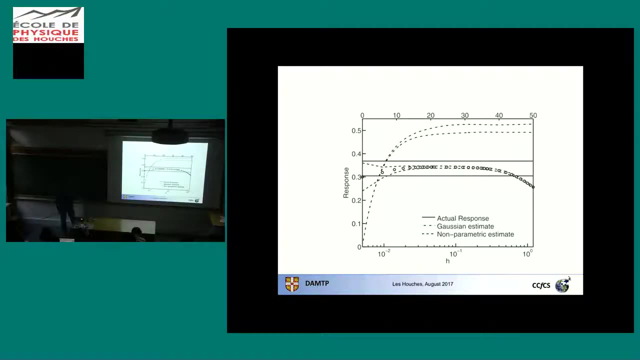 and the one reconstructed with Gaussian FTT, and then the one where you used kernel density estimates. Yeah, And the very first plot you showed of that, it seemed to converge first and then diverge again. yeah, So it can be. could you provide an explanation of why? 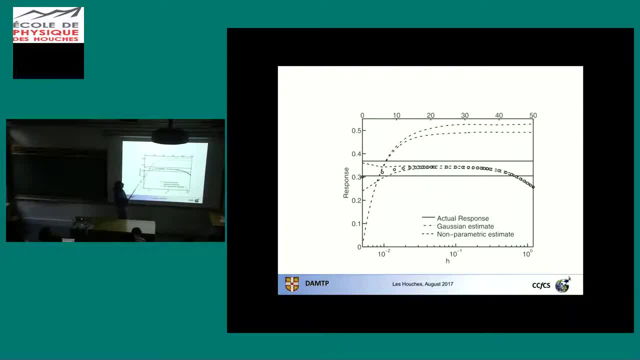 Yeah, so which curves are you talking about? The non-parametric estimate, These ones, Yeah, seems to converge and then diverge somehow. Yeah, okay, that's right. So I mean, this is a case where I was kind of going. 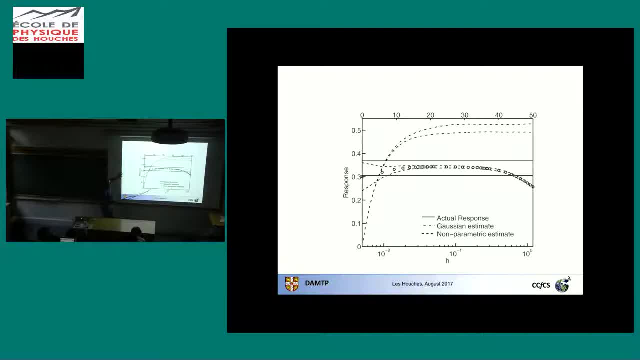 rushing through material, right, But this is an interesting thing to talk about. So, basically, what you're for this curve, what you're plotting here, is as a function of this sort of scale factor for the kernel density estimates. Okay, so if you've got, 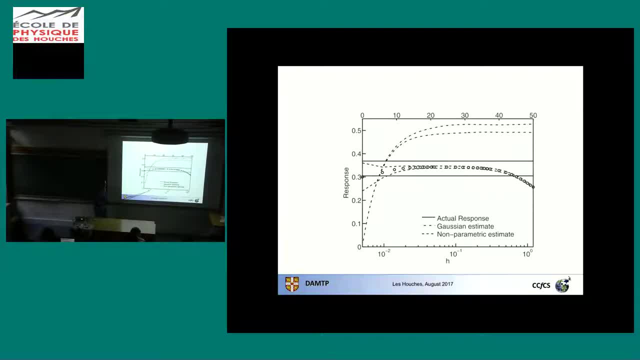 if you have a small scale factor for the kernel estimate, density estimator, then in principle you get an unbiased result. but it may, but it has large uncertainty, Okay, and that's manifested by the fact that you've got a large distance. 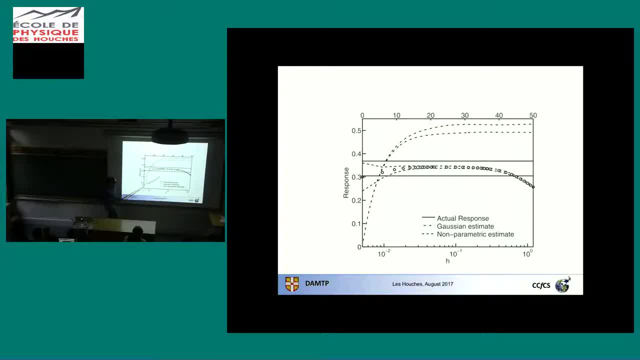 between these two lines. okay, As you increase the scale factor for the same length of data record, okay, your uncertainty decreases. so these two dotted lines move together. but then you at some point start to introduce bias, because basically you're trying to construct a PDF. 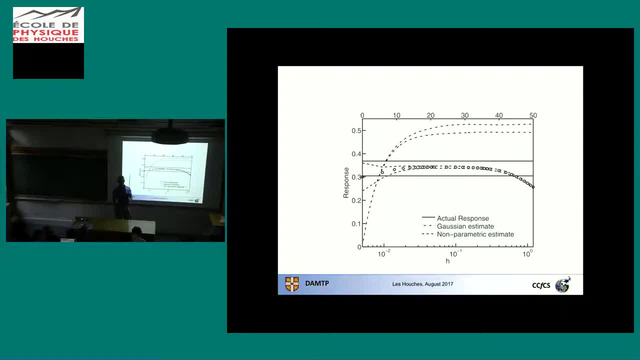 imagine you're trying to construct a PDF which has this scale in it, using kernel density estimators which are made up of functions with this scale right. You're clearly not going to get it right, so there's a bias. Okay, so this is bias. 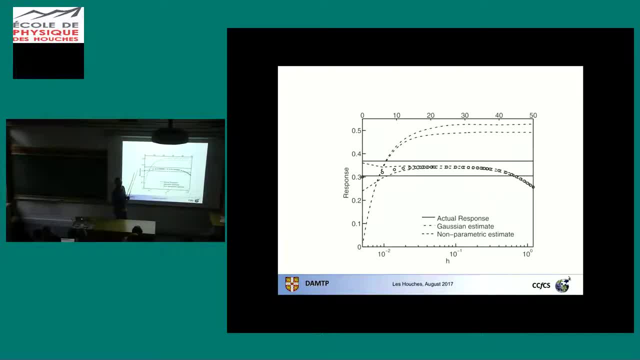 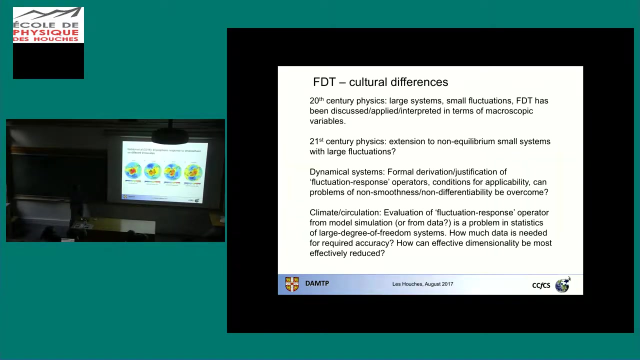 and this is uncertainty. So when you calculate the change in an observable, when you show the formula, it's an ensemble average of the covariance matrices. Can you give an example of how exactly do you calculate, like all the variables in the table? 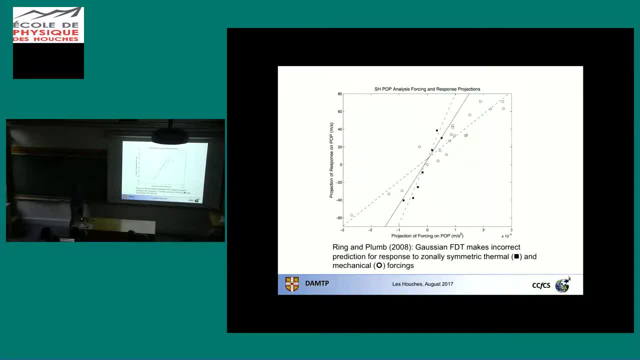 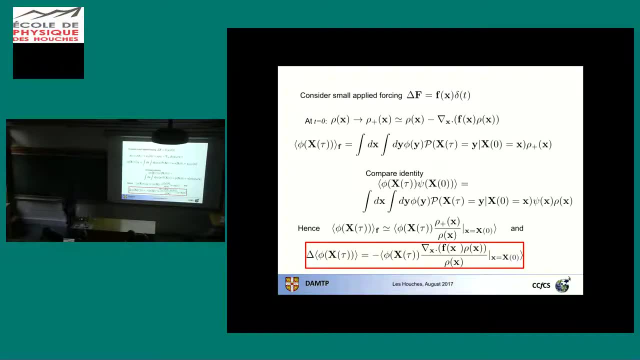 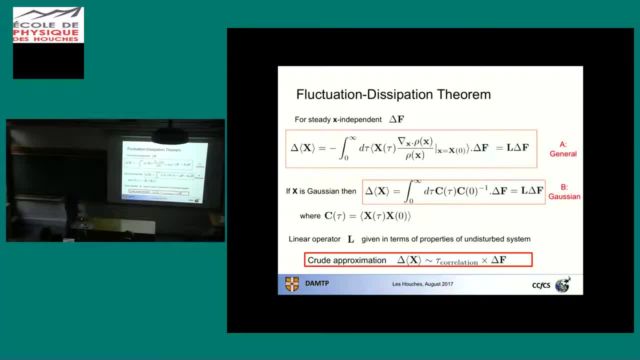 C, C, tau, It's not shown here. Next one, Next Yeah, Yeah time at any given instant. I'm sorry. So it's basically so this thing let's focus on. no, actually, let's go to here, right. 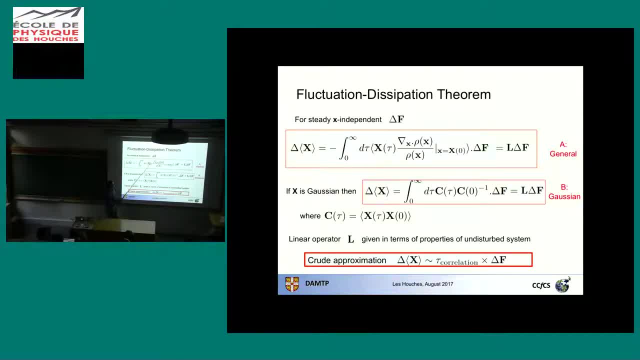 So this is the state of the system at time tour, okay, And then this is a function of the state of the system at time zero, okay. So this is a and then I'm taking the expectation. so it's a kind of lag correlation, okay. 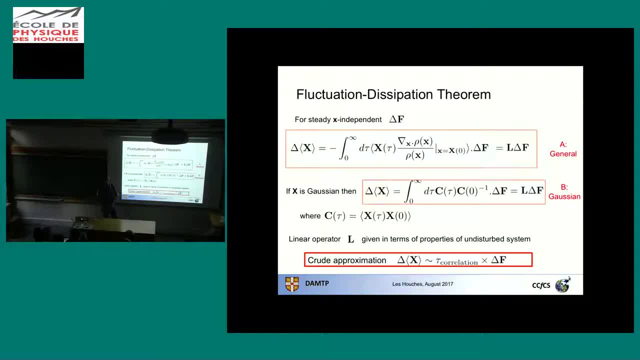 And then I'm integrating over tour. So I'm calculating a certain sort of lag correlation with lag tour and then I'm integrating over tour. So it's more that you've got sort of variability in time okay, And your tour is setting a distance between two times. 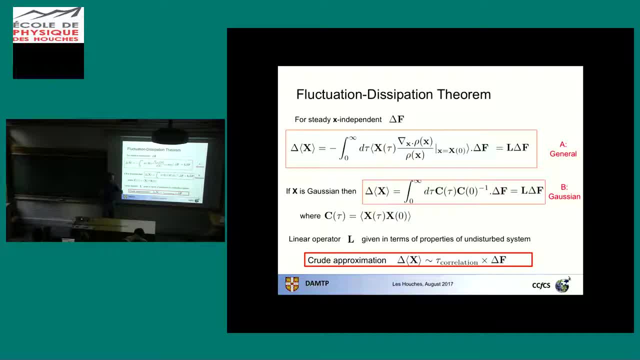 and you're moving through the system, keeping tour the same and averaging the correlation between the value here and the value here. okay, And so that gives you the value for a particular value of tour, and then you're integrating that over tour. Well, exactly, that's right. yes. 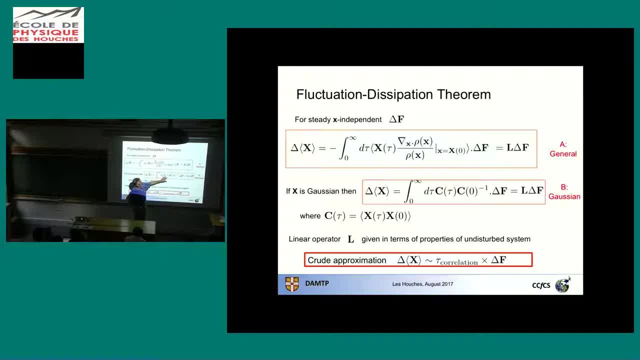 Yeah, So these would be. this is a covariance matrix, which is the matrix of covariance, lagged covariances, between every pair of variables. Yeah, So in one of the first practical application you mentioned, by Krit Sun and Brent Stadler. 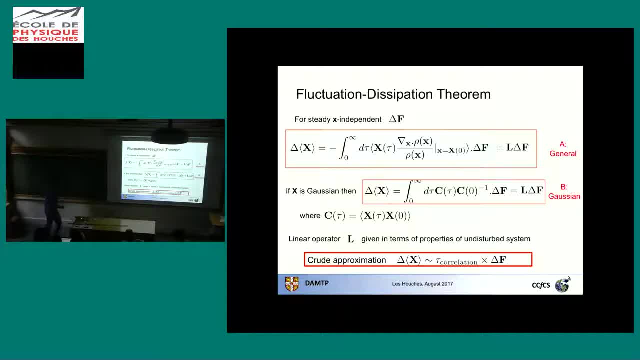 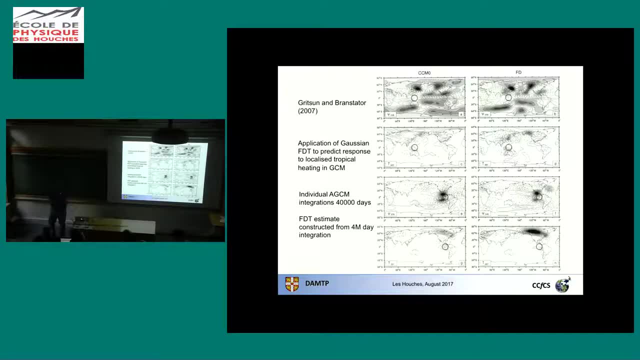 you mentioned that they needed to integrate the models for four million days. You, yeah, so that's. they. estimated the. they used four million day integration. Yes, So it's a bit of a surprising number given that, for example, even in the observations, 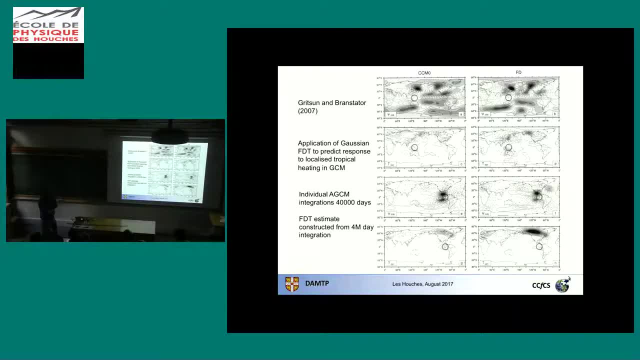 to calculate the observed climatology. we don't have that number of days. So what does it really mean that you need this huge number of days to get statistics? Doesn't it mean that the method is flowing in the first place? Yeah, so, if you like. what I'm saying is that 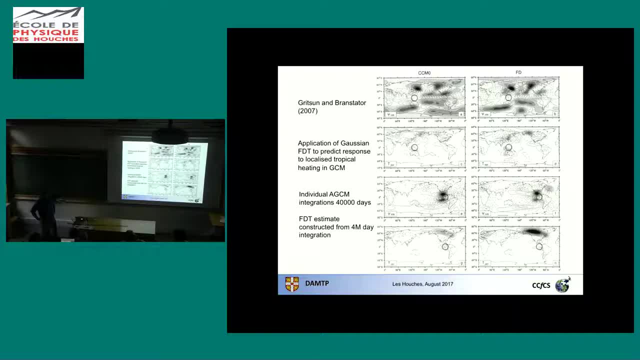 what I think is needed beyond, say, the Gritsen and Brant, the Gritsen and Brant study- is more insight into where does this number come from and what do you get if you reduce it. When do you stop getting anything useful? 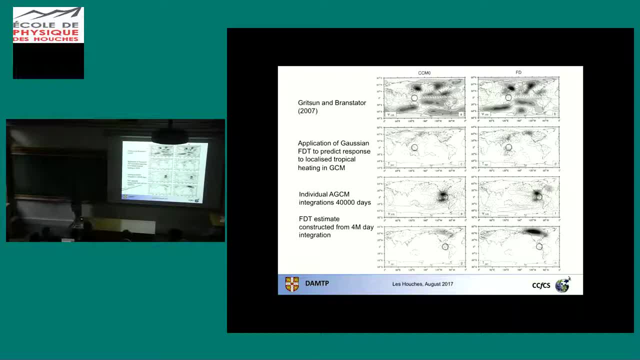 So Gritsen and Brant Stadler. they do actually say we have tested the sensitivity. error results to reducing four million. Okay, We find that they're very insensitive. Well, okay, in a way that's reassuring. But a more practical question might be: 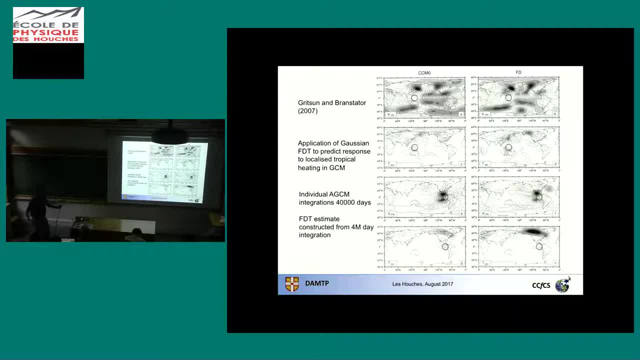 well, supposing I only used 100,000 days, then do I get anything useful? So what I would like to have done myself but haven't quite managed yet. but it would be to come up with a more practical user guide. 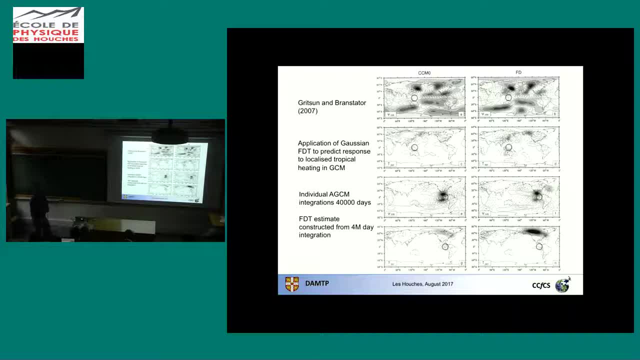 Given a system, given some details of its behavior, can I say what useful information I can get for a given length of data record About these statistical problems? in many problems in physics people have not tried to compute the response from this cubo formula. 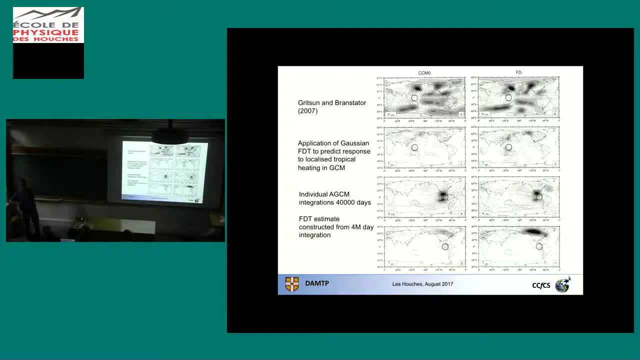 or from the other formula with logarithmic density, but the just computed the response directly from the definition, as is done here, actually through the intermediate plot. So there is a real question about why should you use something more complex than just computing the response by adding or forcing, and computing the response of the statistics. 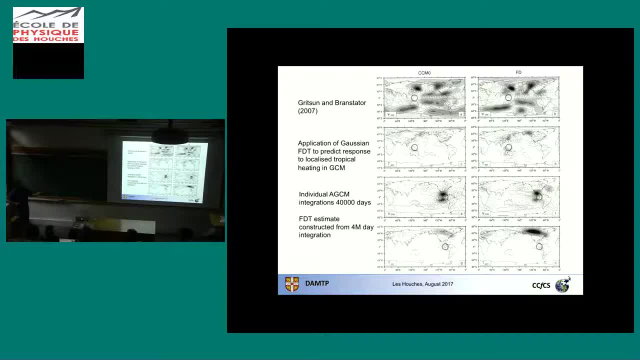 Once again, I think that it's a fair comment. right? Yeah, Thanks, Yeah, Same here, Same here. if the task you are setting is estimate the response operator and I go away and try and do it. this method and you go away and try and do it. 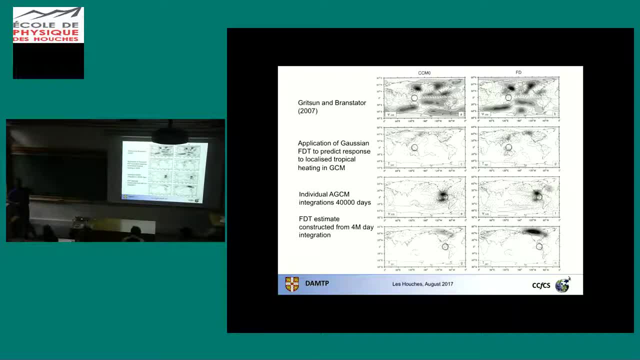 and you do it by simply doing lots of false problems. I mean, you might well end up with a better answer more quickly, But again, one doesn't know that in advance. But then the other thing one's looking for is kind of insight into how the system works. 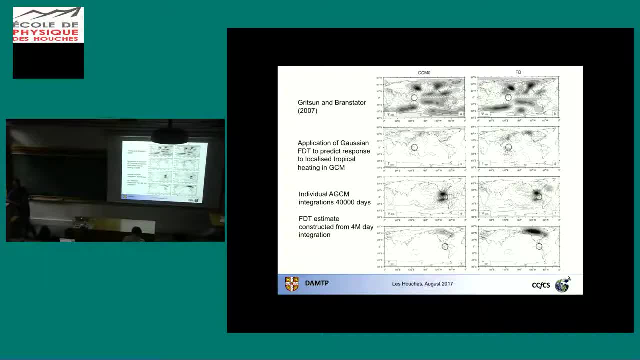 So that approach wouldn't kind of reveal the link between the timescale of variability and the response to forcing right. You would simply get an answer. So there are kind of advantages to different approaches. So another comment is that you have insisted on the 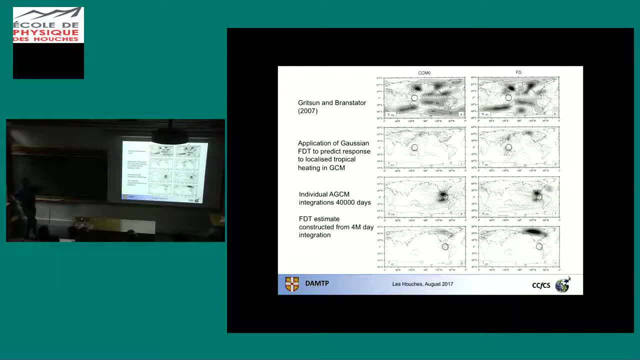 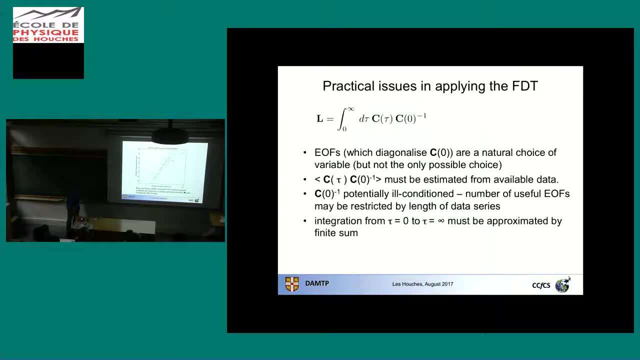 what you said, what is called the static response, just looking at the final value. But in one of the plots you have shown at the beginning, you were showing actually the temporal response. Indeed, that's right, But I mean one could. 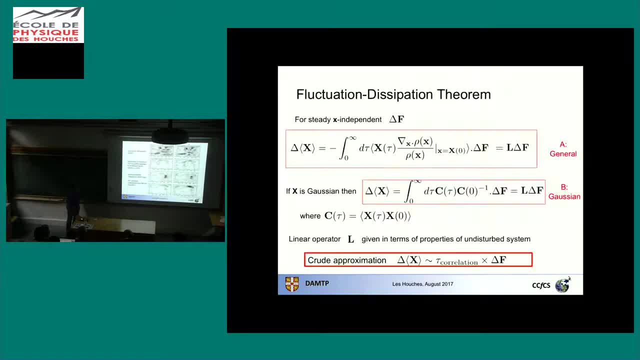 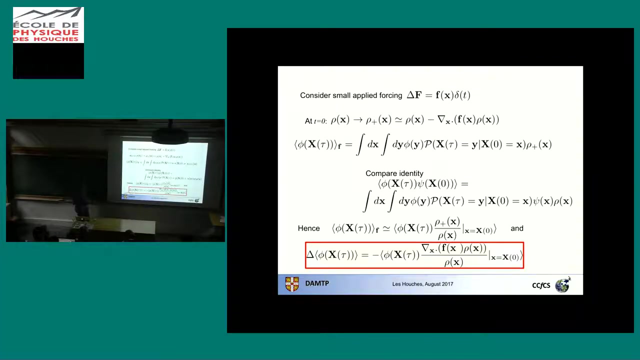 It's a fairly simple step to kind of modify this to give you a temporal response. I mean you simply. Again, you know one simply is going back to the. You know this is the response to a delta function forcing. Then you're simply integrating this. 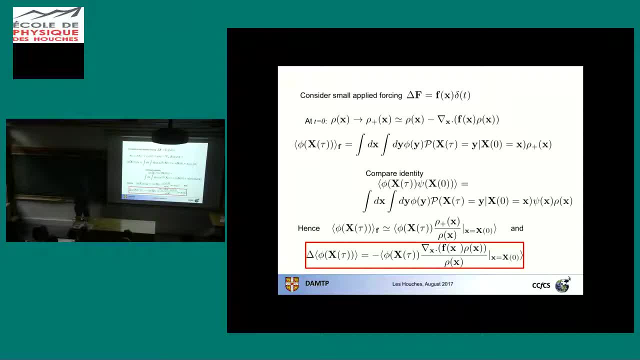 with a suitable waiting function in time to get the time-evolving response. But actually I mean, Grant Branstad has kind of worked a bit more on that problem actually. I'm not sure if I understand that right, but so don't you have to make sure? 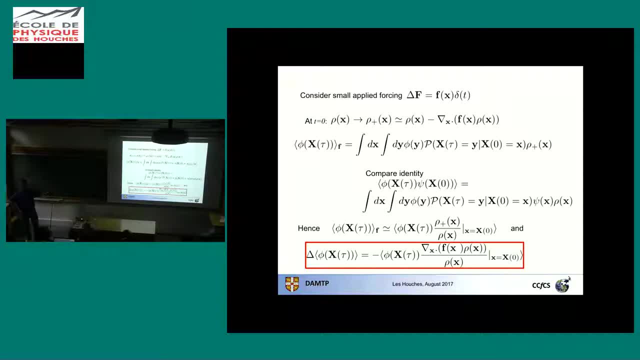 that the forcing that you apply at the second step actually exists in the internal variability. Otherwise, your response functions do not exist right Or they're not represented in your truncated EOF world And the studies you showed so, the one where you just were before the Christian thing. 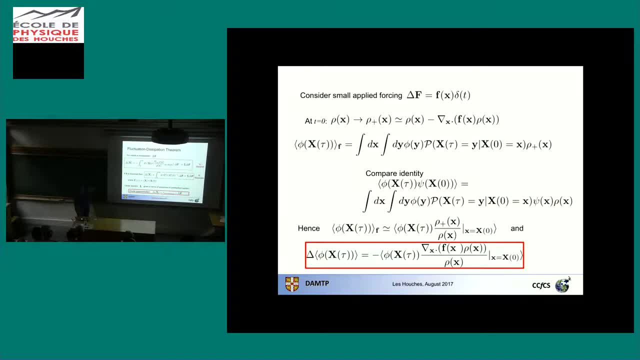 there's an AGCM, so they have an aninu in the first place, basically, or not? So what was the last thing you said? The slide with the eight panels, one of the first where we've just been before, where you're forced with aninu-like warmings. 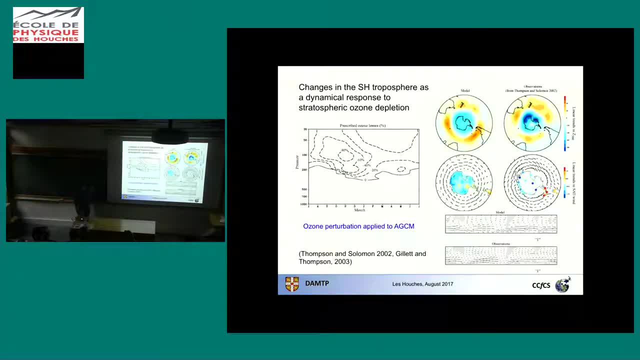 the circles in the tropics. Sorry, you were looking. Am I going in the right direction? I don't know. No, you don't, because not in the beginning. Which slide? am I going to A few further, Further back? 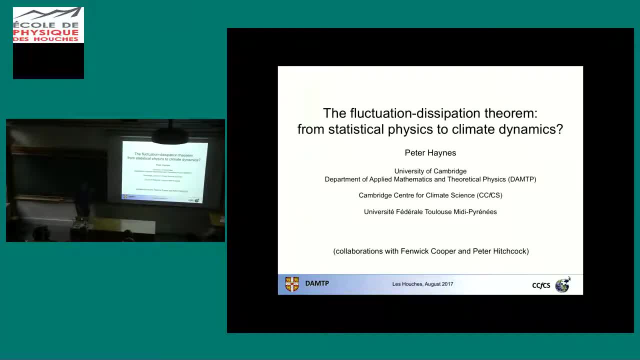 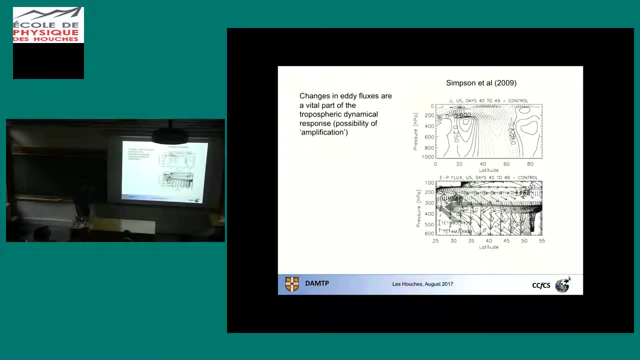 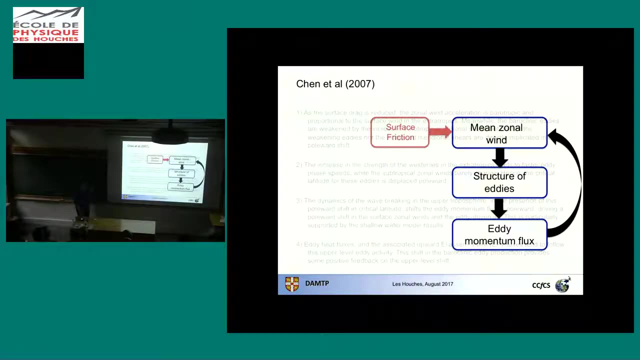 Yeah, there you are. That's the beginning. No, no, no, You mean this direction. No, I just can't pronounce the name Grinston and Branstad Grinston. yeah, Okay, right that one. There we are. 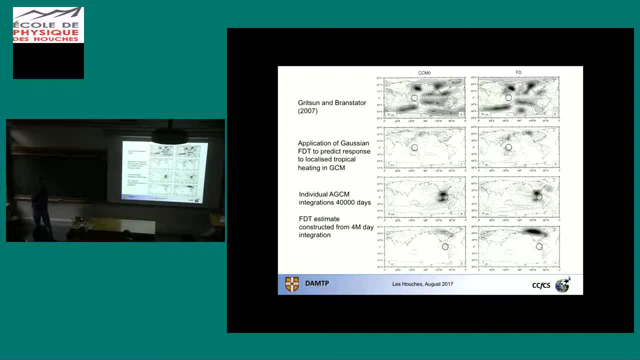 Okay, so they try to force some aninu-like stuff, right, Yeah, So and does their control have a variability that captures aninu is basically the question. If the control one doesn't capture the forcing that you have later, how can it project accordingly? 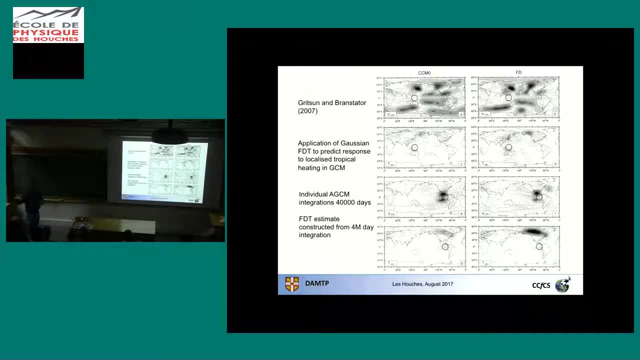 Yeah, well, I think, yeah, the general point is a good one. I think I wouldn't worry too much about Let's not talk about aninu, right, because that isn't really there in this model. I'm heading to the general point. 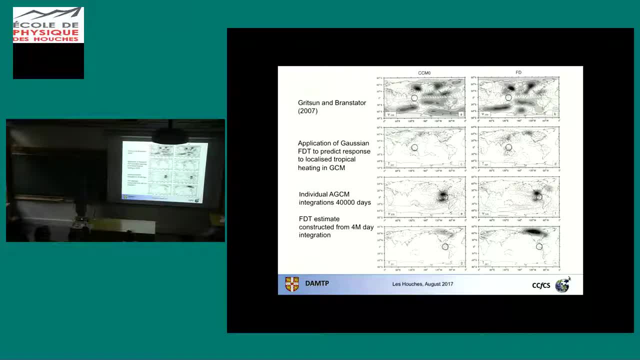 Yeah, but the Yeah, yeah, yeah, it's. It's clear that one You would have a problem, in a sense right, if some region had no variability and your forcing was applied in that region, Something obviously goes wrong, okay. 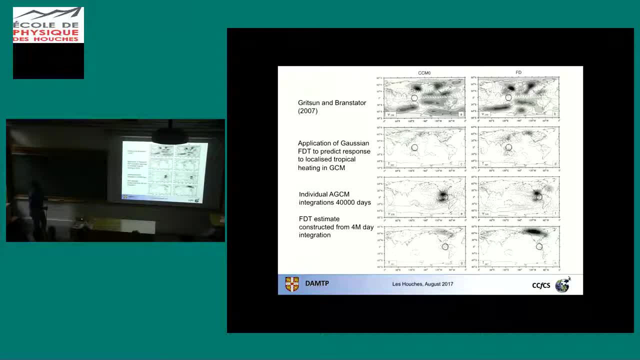 But then you know, why should that? You know? are there regions that really have no variability? I mean, I mean, I think, yeah, what I would? I mean one thing that I would say right, which is not necessarily agreeing or disagreeing, right. 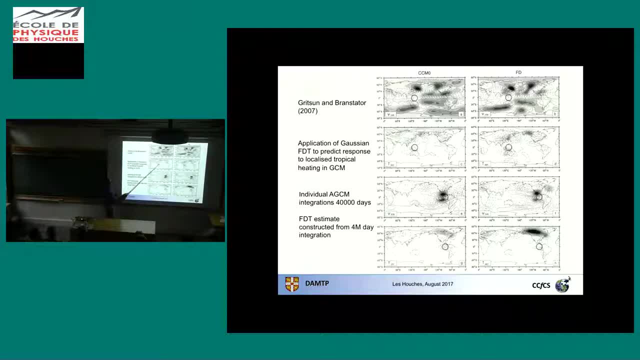 but sort of different is that it's kind of One sort of imagines that if one is looking at- Well certainly if one is looking at- The response in the tropics, then one has, Yeah, one would imagine that that depends. 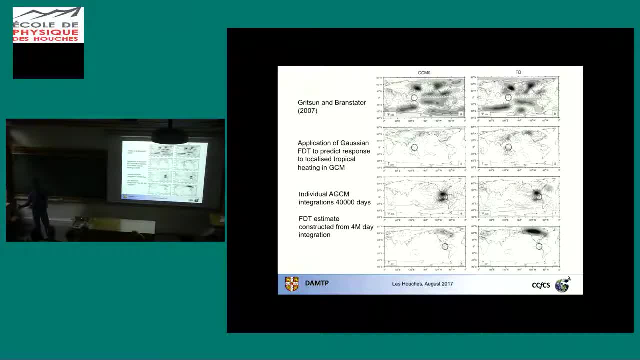 on variability in the tropics, right? So if your model has the wrong variability, then you will get the wrong response. Is that a compromised position? Well, no, but again right. I mean, there's the question about you know. 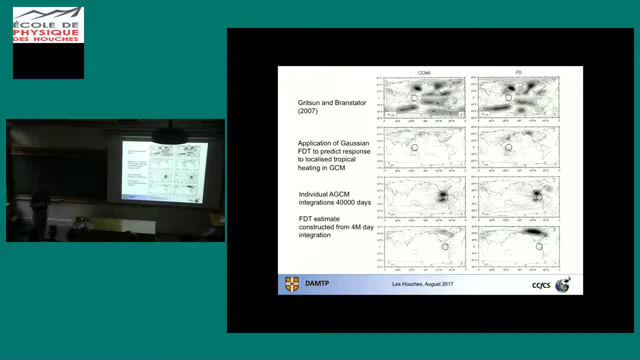 how to understand the model response right As opposed to the right responses, which is the response to the real atmosphere. so If the model has unrealistic variability, say in the tropics, then the model will give you the wrong response in the tropics. 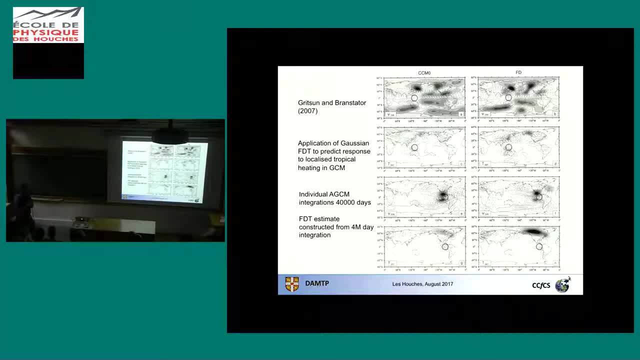 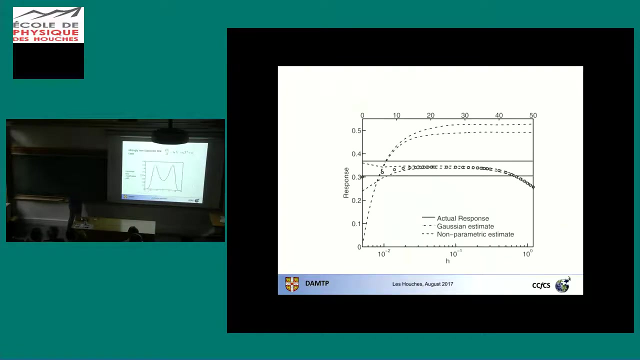 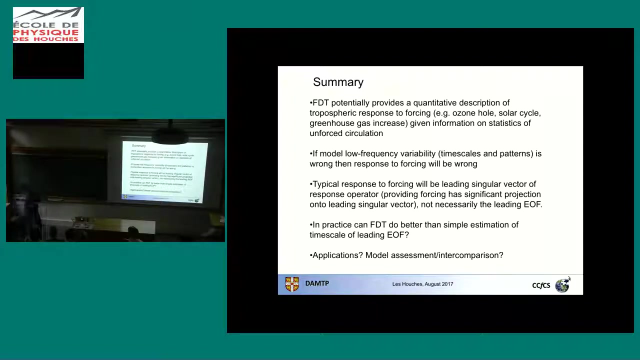 Oh, yeah, yeah, yeah, Hmm, Okay. so may I make a last comment about your slides, about the history and maybe the different focus during the last century. Which one Culture- sorry, The cultural one Culture- was a dangerous use? 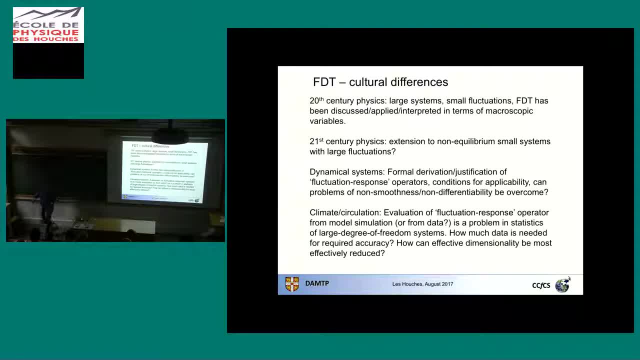 The cultural difference. Yes, so I think the- So what you call 20th century physics is related to the Green-Kubo formula. Yeah, And so this is basically the, I guess, the middle of the 20th century. Yeah, 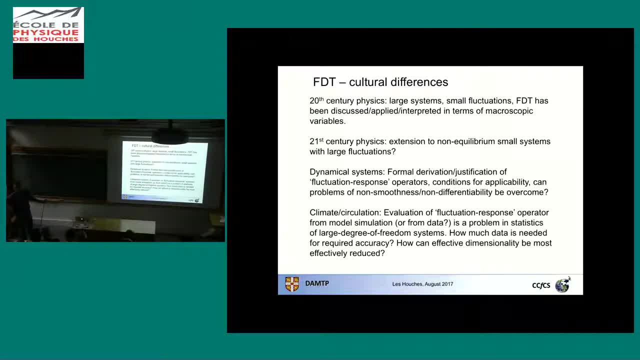 And before, And then the formula you use with the gradient of the logarithm of rho divided by rho. So this formula has been written first by Decker and Acker, I think in the 19th century. Yeah, Yeah, Yeah. 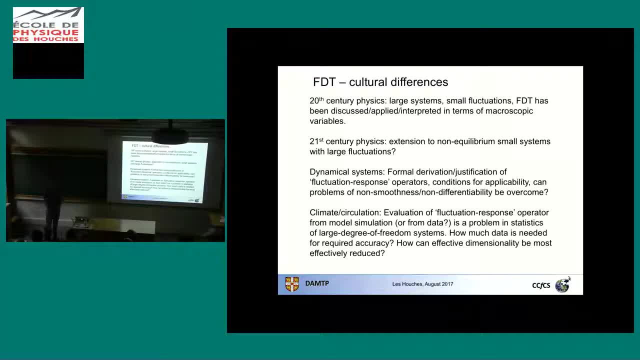 In the context of the Fokker-Planck equation. And then I guess what you mean here- dynamical systems- is the works by Ruel and the collaborators- about trying to justify this for deterministic dynamical systems. I mean, I guess that this is. 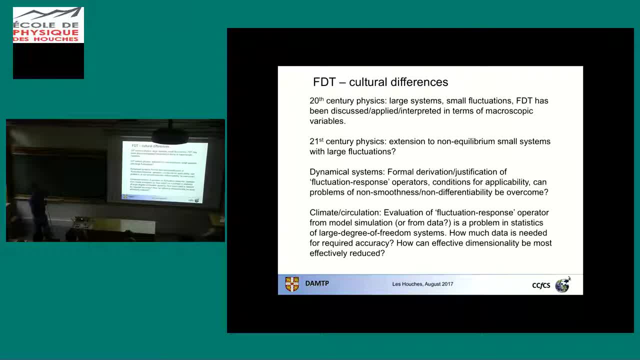 a slightly confused slide right, But it's partly prompted by the fact. Well, the first thing would be that when I remember once talking about this- not work- to a physicist or someone I thought was a physicist And you know- I sort of said you know. 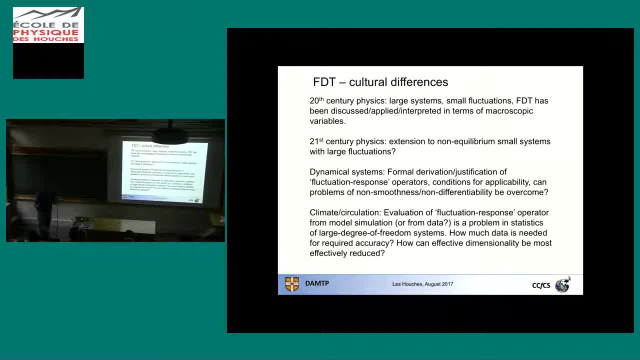 thinking about this formula, and the formula had explicit covariances in it And his kind of reaction was well, kind of, where's the interest in that right? Because it seemed to me he was coming from a world where he would be using you know. 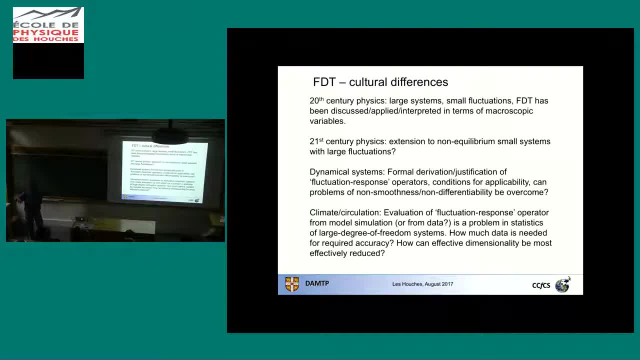 thermodynamics or other physics to predict what those things would be. to predict what those things were. okay, Yes, in physics, for instance, there were shining light on liquids or any kinds of materials, And then they were looking at the response. 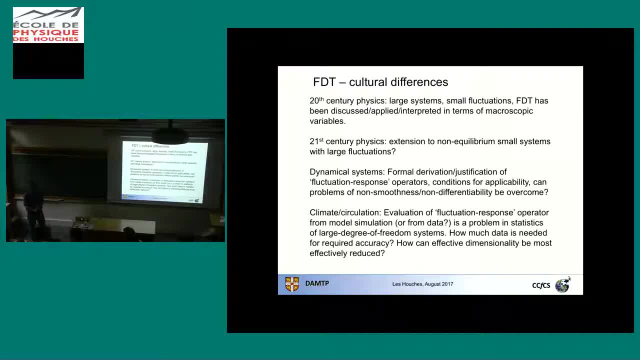 And then they knew how to relate the response to the transport coefficient, the viscosities, and also the temporal behavior, the susceptibilities. So that's what it was used for: actually to measure the transport coefficient. So it was used to measure the dynamical response. 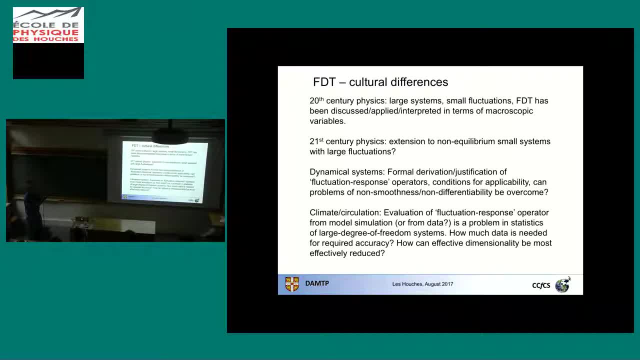 But I mean, I think it sort of comes down to what you know, what can you get out of the application of the theory, right? So if people sort of thought- Someone who came to this seminar and thought I was going to provide to the operator, 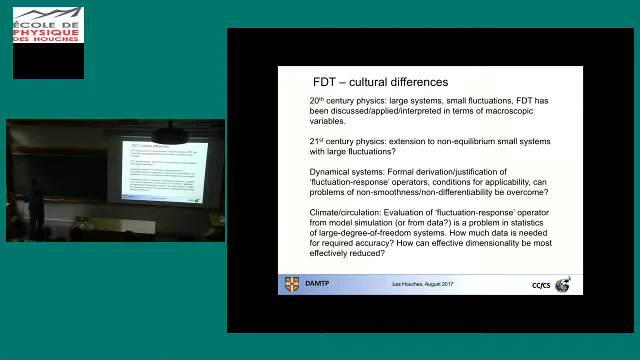 in terms of sort of some you know, geophysical parameters or something right would go away, disappointed, right. What a waste of time because I didn't ever present an operator in terms of sort of external physical parameters, But you know. but the operator does give you something.